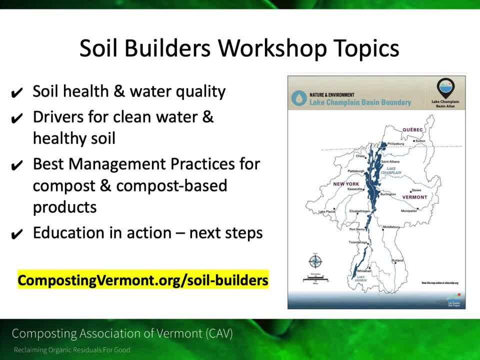 sort of an introduction and then topic specific best management practices for compost and compost based products. So really getting clear that not all composts are the same And to get the results that we want, we need to understand which products to use for which applications, And Deb will be. 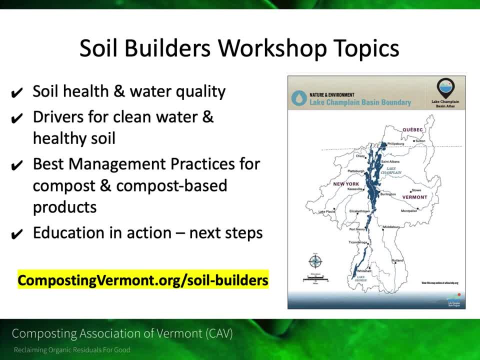 going into a bit of that today. And then we also have these education and action or next steps. We've had one of these so far and this is really like now. we know all this great information. What do we do? How do we actually affect change in our communities and in the water? 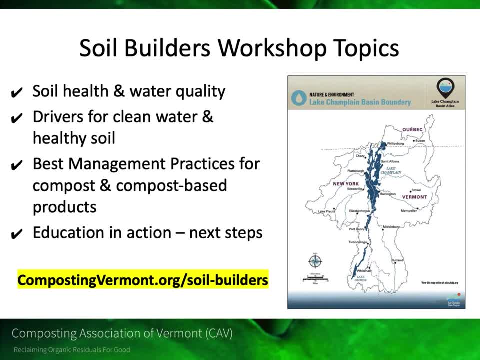 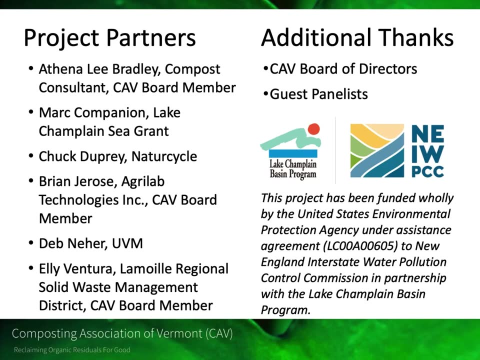 quality and the lakes and rivers and creeks that we all enjoy. So all of this information in the prerecorded webinars are at compostingvermontorg forward slash soil builders. Just a quick thanks to my project partners: Athena Lee, Bradley, Mark Companion. 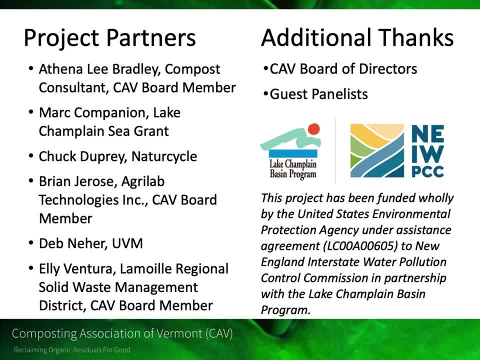 Chuck Dupre, Brian Gerose, Deb Nair and Ellie Ventura. An additional thanks to the MICAV board of directors, as well as the guest panelists that we have participating in different webinars that are really making this program so successful, And, of course, a big thank. 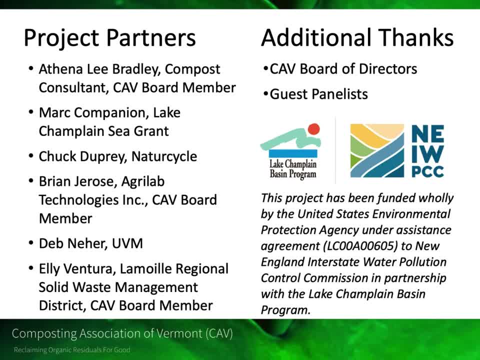 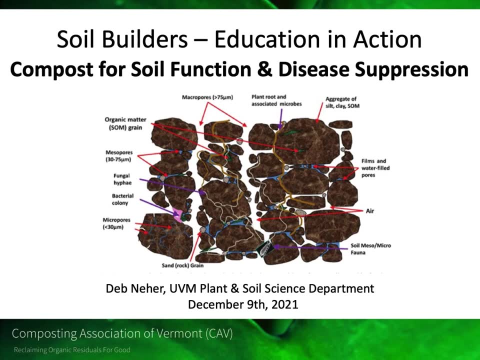 you and acknowledgement to the funding that we've received from the Lake Champlain Basin Program and the New England Interstate Water Pollution Control Commission, who are supporting this work. And so now on to the fun stuff. that is why you guys all came. I'd like to introduce Deb Nair. 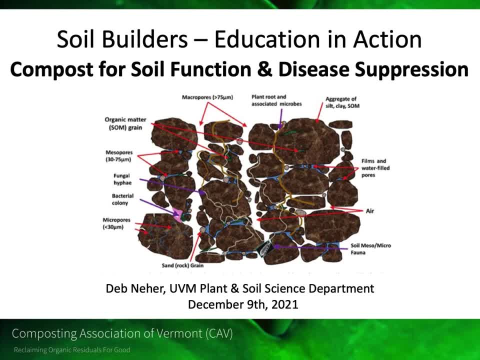 who is a colleague and a project partner on the Soil Builders Program. Deb is a soil ecologist in the Department of Plant and Soil Science at UVM. During her master's she gained a foundation in theoretical ecology and then focused on ecology and epidemiology of root pathogens for her PhD. 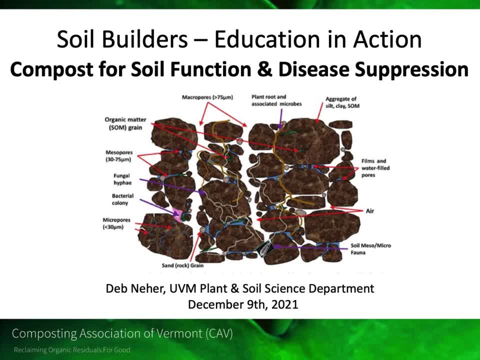 Deb then began research on nematode community indicators. She spent six years at North Carolina State University, my alma mater, where she initiated her research on biological indicators for environmental monitoring of soil using nematode community indicators. Deb held faculty positions in biology and environmental science at the 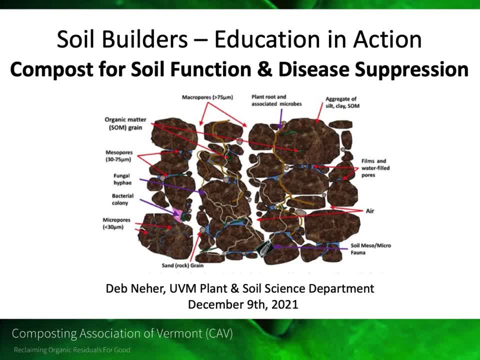 University of Toledo in Ohio, and in 2004 she joined the University of Vermont as department chair of the Plant and Soil Science Department. In 2018, Deb resigned from administration in order to: In 2018, Deb resigned from administration in order to. 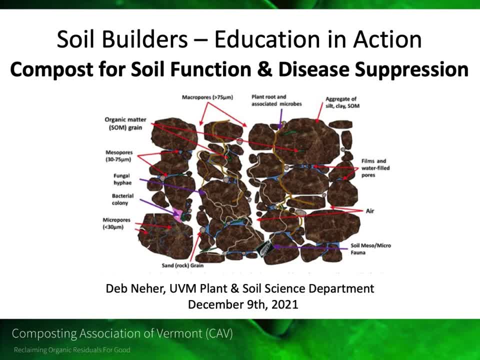 be a graduate student and then retired from the University of Vermont as a postgraduate student, In focus on applications of her extensive research to farming and to inform policy. During the past several years, her research has included pilot studies on biological communities and compost and their role in disease suppression, including farm trials looking at compost-based products. 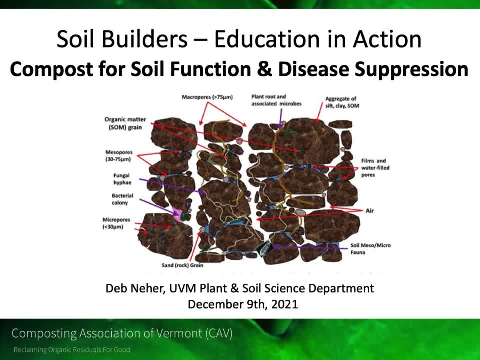 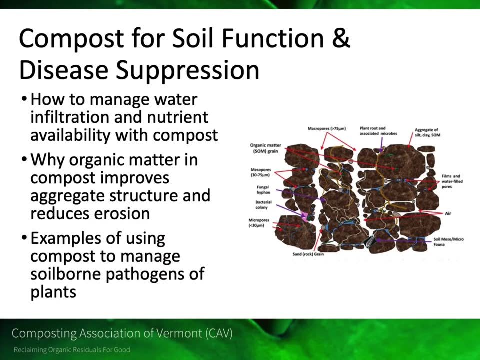 for soil function and disease control. We're going to be hearing a bit about her research today, which is really exciting. So, Deb, take it away All right. Thank you, Natasha, for that very nice introduction, So we're just going to jump right in. There's kind of two parts to my 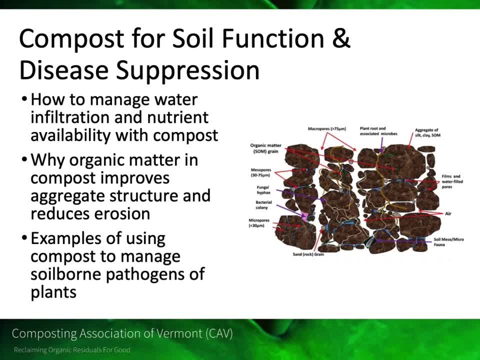 presentation today. The first one will be looking more at physical properties of soil, And then the second part will be focusing on my research related to using compost for disease suppression. This illustration is one I really like over on the right. It's one that kind of gives you an overall perspective about how physical properties of 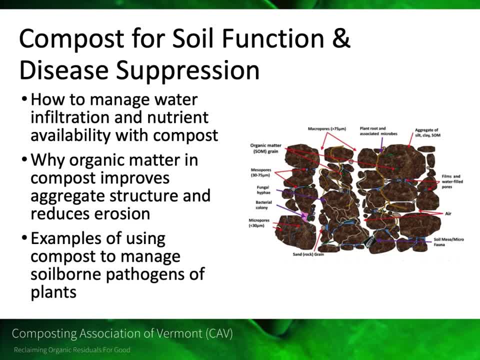 soil can relate to water infiltration, as well as providing habitat for the living portion of soils, And in today's webinar, we're going to focus on three things that I have in bullets: How to manage water infiltration and nutrient availability. Why organic matter and compost improves aggregate. 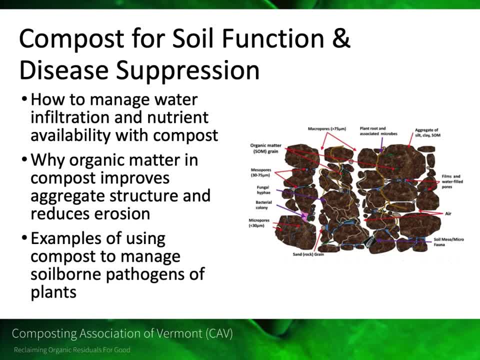 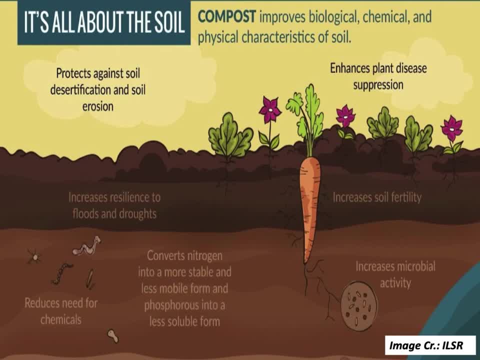 structure and reduces erosion. And then examples of using compost to manage soil. So from the previous sessions we had, we discussed about when soils are disturbed or degraded they really do not function properly, But we can use compost to help remediate degraded soils and 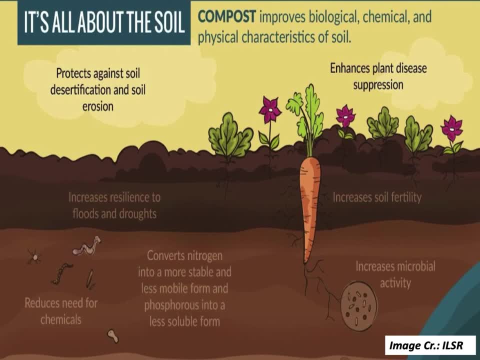 add resilience by contributing to all the characteristics of healthy soils. The ultimate goal with compost and healthy soils is to be able to grow plants, to grow vegetation And then the vegetation. once that's there, the rooted structure can help help hold the soil and nutrients in place and help protect our water. 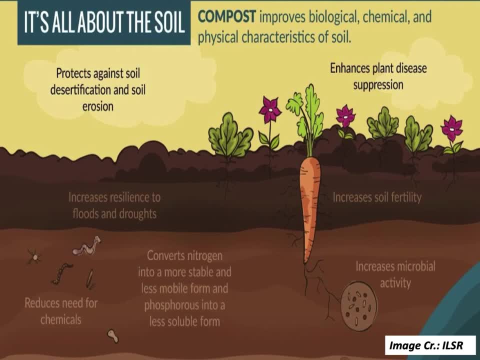 This tripartite relationship between soils, plants and water is possible because compost helps soils absorb and retain nutrients and moisture, And it protects plants from diseases and pests, serving to protect watersheds, And this is really important for having a healthy Lake Champlain. 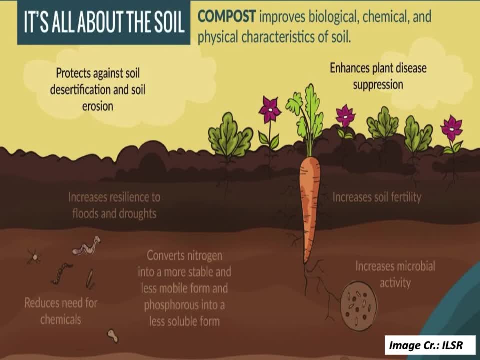 plain ecosystem. we want these healthy soils to help restore native species habitat, nutrient filtration, flood resilience and sediment retention. When we do have healthy soils, the phosphorus will bind to the soil particles that erode from the stream banks and help protect. 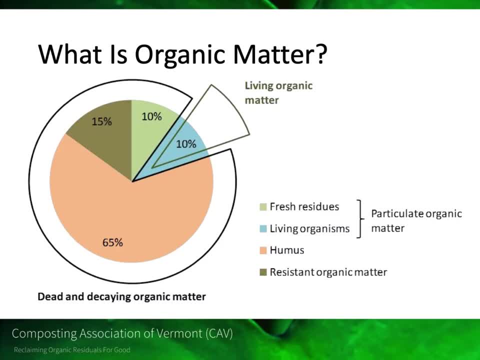 our water quality. So one of the key contributions that compost provides is organic matter. You know, remember, we have soils made of mineral particles. There's pockets, open spaces that contain air. This is also where a lot of the soil biology lives And organic matter, And that organic matter is the 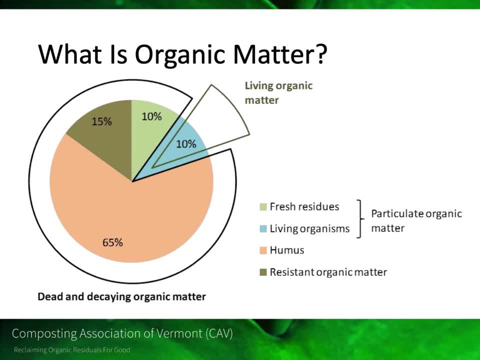 component that compost can really add to soil. And organic matter itself is really the portion of the soil that houses and feeds the biological components of soil. So what is organic matter? You can see in this slide: it contains plants. It contains plant residues, plant roots, animal residues. It's got living materials as well as dead and decaying materials. 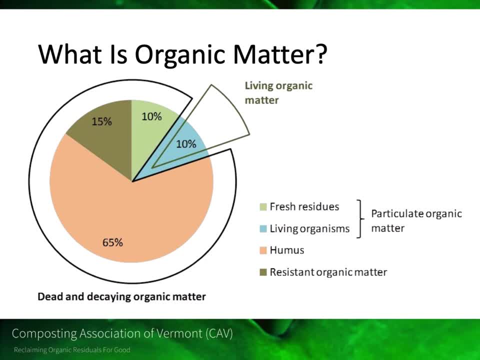 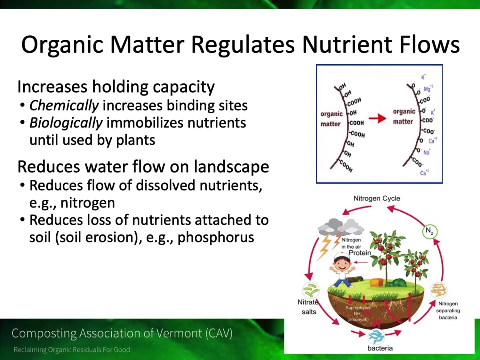 Soil. organic matter itself really profoundly affects soil properties and the functioning. It's involved in aggregate formation and the stabilization. It provides an energy source for the soil organisms. It helps with water retention, acting like a sponge, and for nutrient storage. Organic matter helps to regulate nutrient flows. Compost itself improves- you know- chemical characteristics. 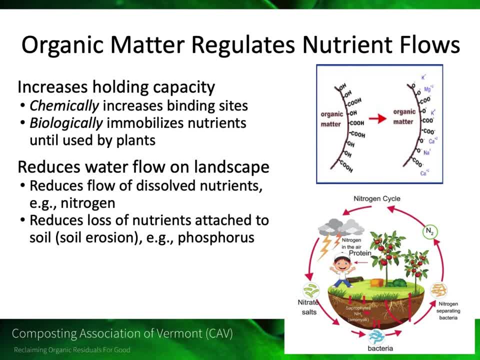 You know these nutrients providing nitrogen, phosphorus and other micronutrients and especially affecting their availability when the pH is appropriate. But there's a couple key components on terms of how this works. One is that it relates to capacity: Organic matter increases the holding capacity of these nutrients. 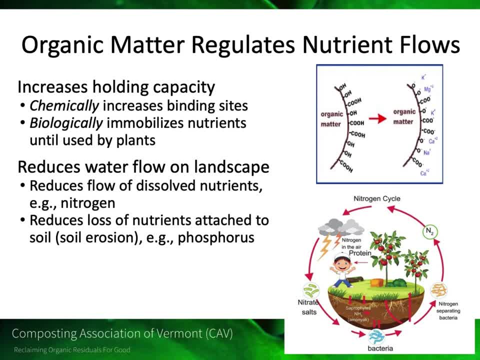 the key features illustrated on the upper right. where the surface has these, it's a surface covered with negative charges And it ends up nutrients have a positive charge, So these can attract to each other like magnets. So opposite charges attract And it's a number of these. 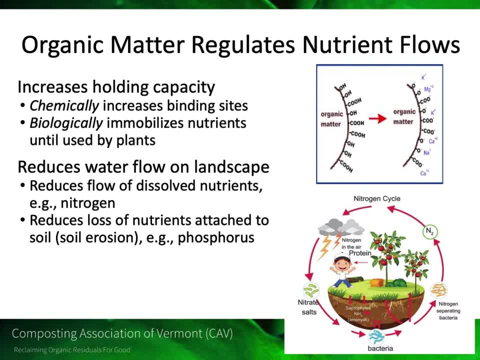 charges that can attract nutrients that we refer to as capacity. So we can also think of it as this is the part that we say exchangeable nutrients, because these nutrients, can you know, attach and detach from the surfaces of organic matter. At a landscape level, compost helps hold nutrients by 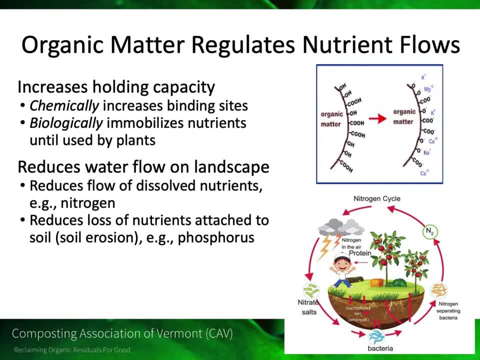 helping to reduce the water flow And this helps reduce the loss of nutrients that are dissolved in that water, And compost is also helpful in reducing erosion because the nutrients are going to adhere better to the soil And in healthy soil the phosphorus is binding with these soil particles, as I mentioned before. 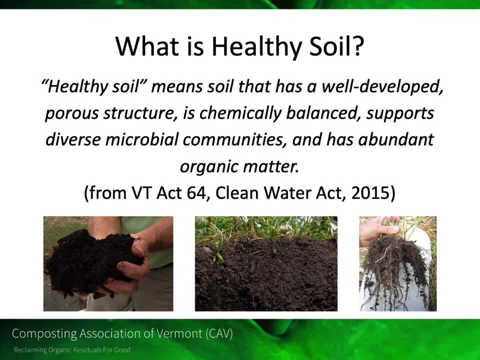 And this helps maintain water quality. So what is healthy soil? We're lucky. here in Vermont, the definition of healthy soil is actually in statute And it has the following attributes: Porosity is a key feature. It's the porosity of the soil that really is the factor that improves. 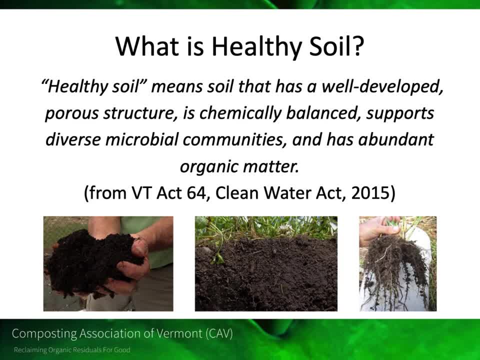 water infiltration and retention. It's the porosity that also is the space in the habitat for the soil organisms. A healthy soil is also chemically balanced, you know, with a moderate pH which helps regulate the nutrient availability. If you have a neutral pH then you don't risk say having reduces the risk of heavy metals in. 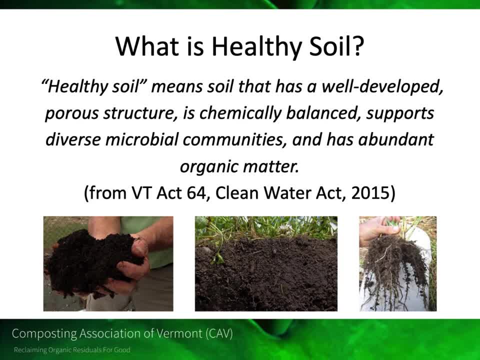 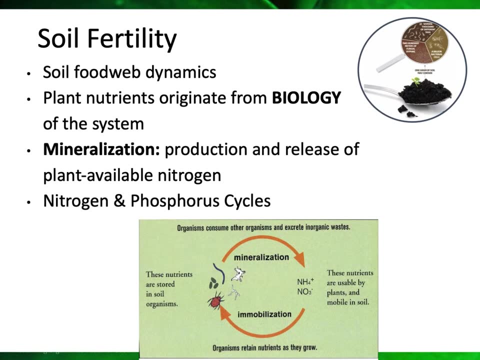 solution. And a healthy soil also has an has abundant organic matter, And it's this organic matter that really holds moisture and nutrients just like a sponge. So compost contributes to more than just more than nutrients. Fertilizers only provide nutrients, but compost is also providing that organic matter and the microorganisms that are. 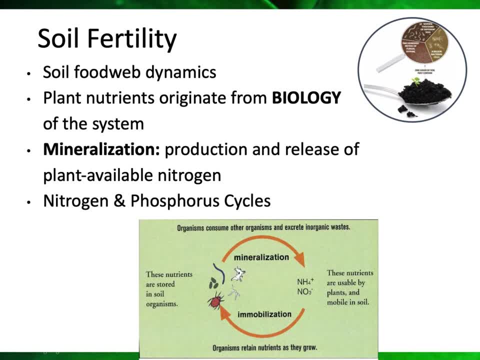 recycling nutrients. So with compost you're not just getting that nutrient product, you're also getting the machinery that helps regulate the solubility of those nutrients that fertilizers do not have. The term mineralization is referring to. it's kind of the name. 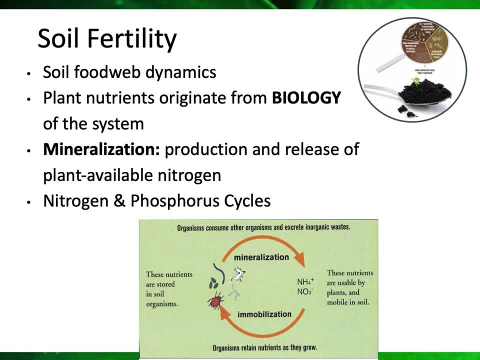 of the process of converting between different forms of nutrients And can. it can apply to both nitrogen and phosphorus cycles. Complex food webs in soil contribute to ecological processes that include decomposition and nutrient cycling. These are both essential to food production, as well as the purification of soil and water. And in the upper right hand. 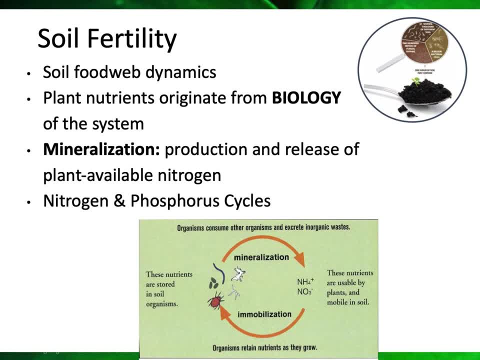 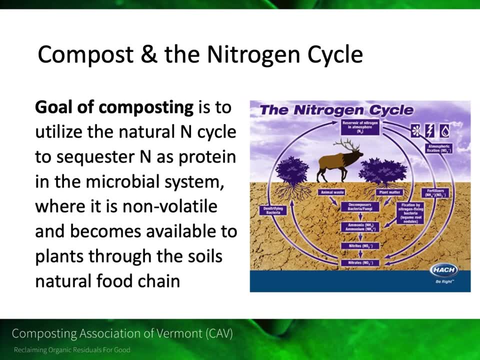 corner. it reminds me to tell you that one teaspoon of soil can hold as many or more living organisms than there are people on earth. Now let's talk a little bit about the nitrogen cycle. Plants cannot take up atmospheric nitrogen, Even though atmospheric. 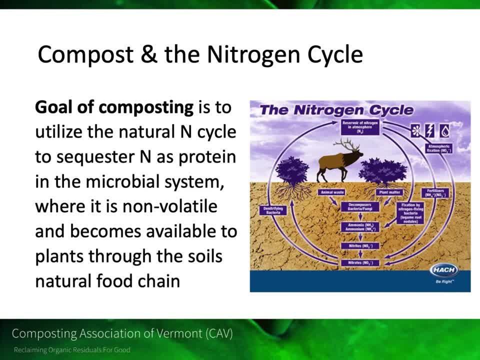 nitrogen is very abundant. those molecules are held together with a triple bond And this is a very difficult bond to break. However, there are some very specialized bacteria that can make that conversion and converting it nitrogen into either nitrate or ammonium. 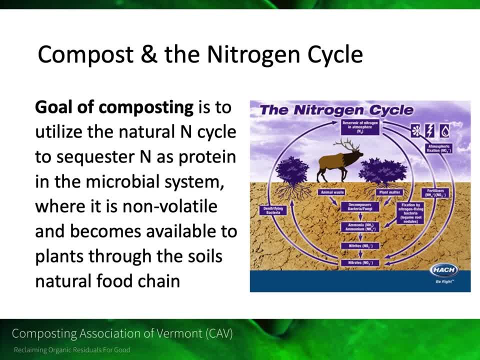 which are two forms of nitrogen that can be converted into nitrate or ammonium, which are two forms of nitrogen that can be converted into nitrate or ammonium, which are two forms of nitrogen that plants can take up. These forms can also be produced as synthetic fertilizers. 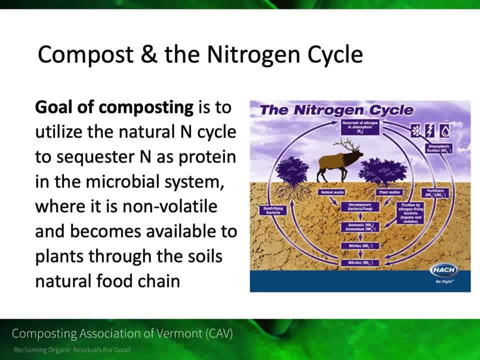 but we can achieve these by nature, you know, through microbes. And then there are also some of the microinvertebrates, like protozoa and nematodes, that also help with this conversion. The bacteria: there are nitrogen fixing bacteria that are able to capture this nitrogen gas. 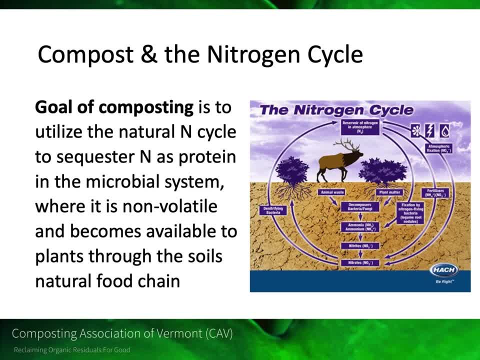 from the atmosphere and convert it into ammonium, which is a form- that of nitrogen- that is produced out of nitrogen that plants can take up. Protozoa and nematodes also excrete ammonium as a byproduct. Remember what I said about compost, adding organic matter and thus the 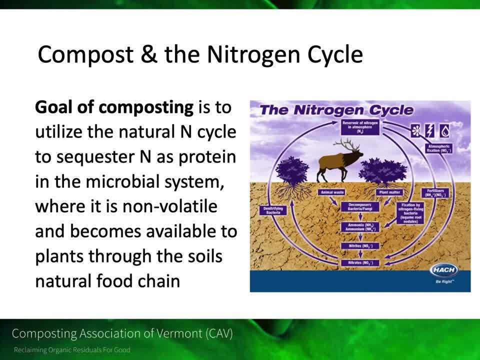 capacity of soil to exchange nutrients at its surface like magnets. Well, this is where I kind of think of compost as acting like a savings account. It's providing organic forms, okay, that are kind of holding the nutrients in the bodies of those living organisms. 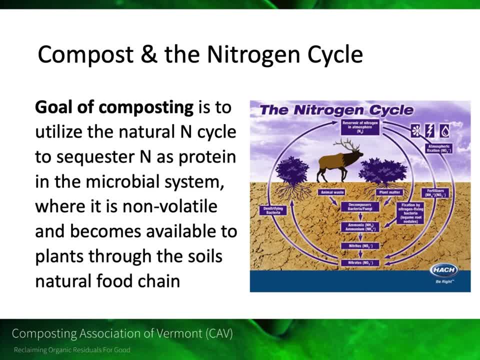 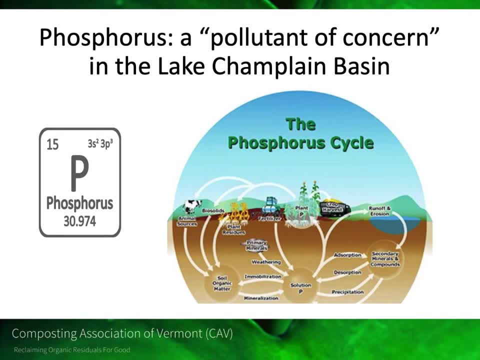 or maybe even dead and decaying organisms. Therefore, kind of making sure that they're kind of making that release a slow release so that it can time it better to plant nutrient availability. All right, Next phosphorus cycle. This is a pollutant we hear a lot about. 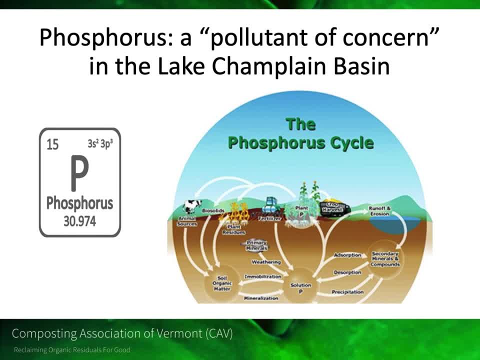 here in the Lake Champlain Basin We don't get phosphorus from air and we have to mine our phosphorus from phosphorus containing rocks And there's a finite supply of phosphorus So we don't want all our phosphorus going into the lake. You know this is a limited 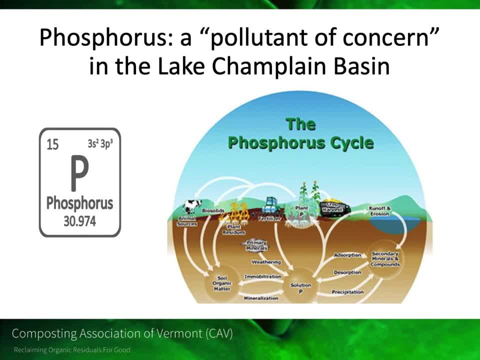 source. We want it, therefore, as an essential ingredient for, you know, our food production. Phosphorus is essential for life. It's in every molecule of DNA and every cell membrane. Those membranes contain what we call phospholipids, because it's got phosphorus attached to the 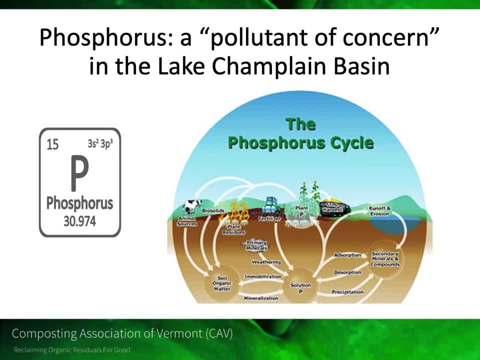 fat, the lipid molecules. Now there are organic and inorganic forms, soluble and insoluble forms. It's the soluble forms that get into Lake Champlain, But phosphorus is not a soluble form. The insoluble forms attach tightly to clay and they flow with erosion sediments. 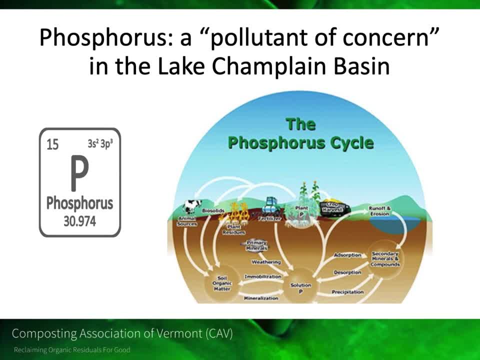 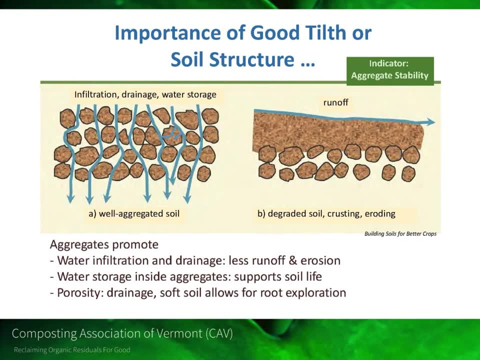 And this is where, if we have organic matter, you can increase that kind of magnetic capacity and holding those more tightly and preventing them from flowing. A measure, an indicator that I find incredibly valuable for soil health is that of aggregate stability. If I had to, 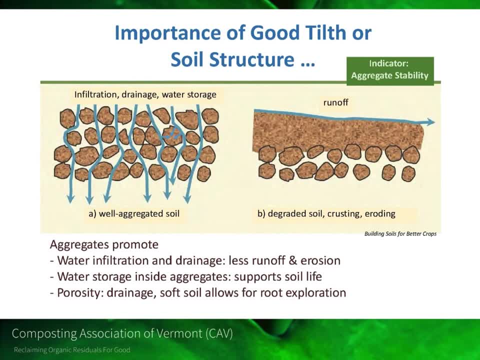 choose one metric to measure for soil health, it'd probably be that because it combines water and the biology of soil. Now let's talk about what the function of these aggregates are. A well aggregated soil is illustrated on the left. It's promoting water infiltration. 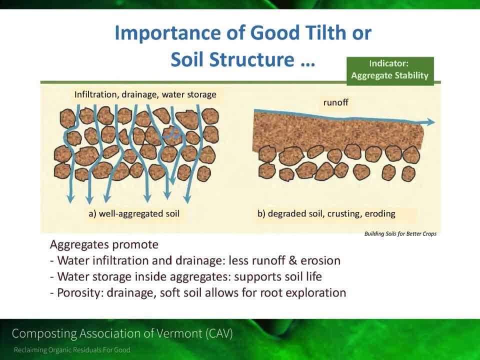 drainage as well as water storage, And that is because of its porosity. The water is able to move through there. In contrast, if we have a compacted or a poorly aggregated soil, like on the right, if we have water coming there, it's not going to infiltrate. But 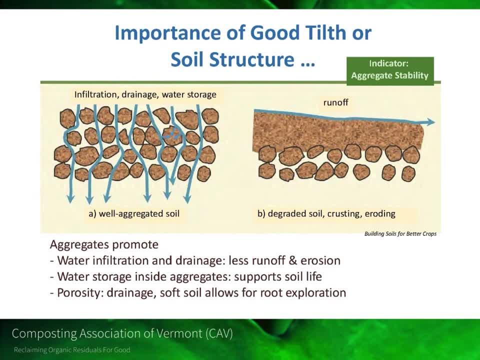 on the left. it's just going to run off the surface. I like to think about compost as kind of being one of the best irrigation systems. It provides better moisture retention and less watering and allows you to be conserving of water and help also reduce runoff pollution. 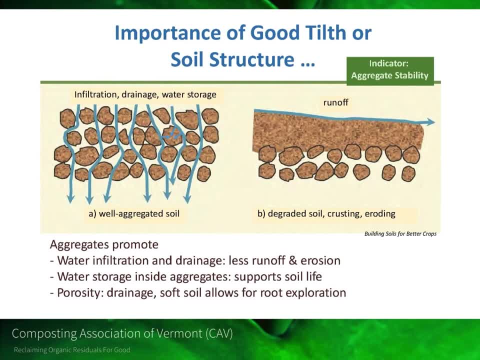 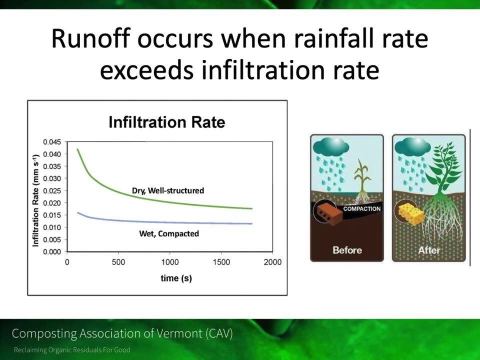 These pores also will not only provide drainage, but, again, these are spaces are needed for root penetration, for plant growth as well as providing habitat For the soil biota. So, if we have plenty of soil aggregation as well as organic matter, 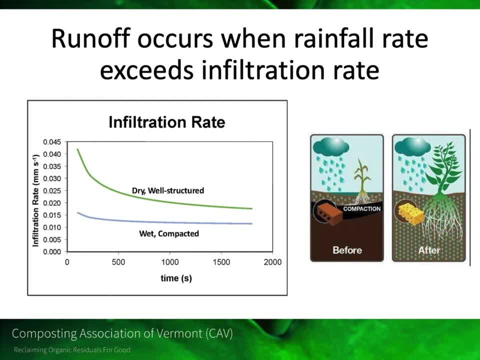 this helps keep the soil kind of fluffy and prevents it from compacting, which helps to improve water infiltration as well as root penetration. On the panel on the left, the graph there illustrates nicely how infiltration is much more efficient in well-structured soils in the green compared to the two compacted soils. 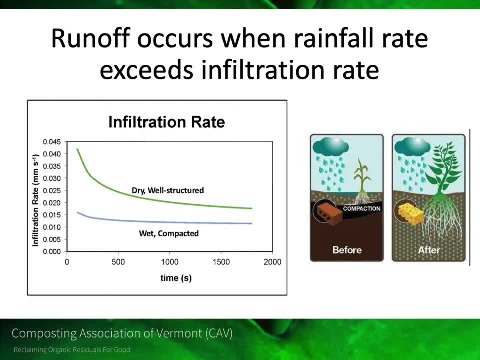 And on the right, illustrates how having the aggregates in the organic matter gives the soils a sponge-like quality, helping to provide a physical matrix that helps protect the integrity of the open pores within it, And, in contrast, compacted soil behaves kind of like a brick. 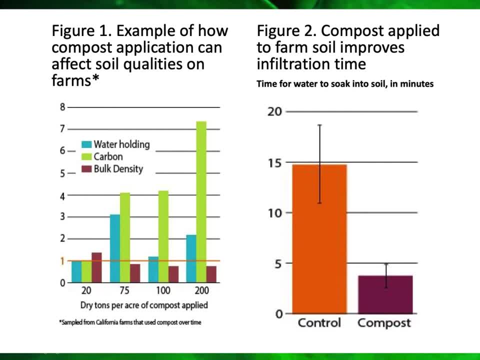 Now, why is compost considered to be one of the cheapest irrigation systems? Well, these data help tell the story. These data reflect a summary of the data. This is a summary of many studies where they looked at different types of compost that were added to soil and major changes in soil physical properties. 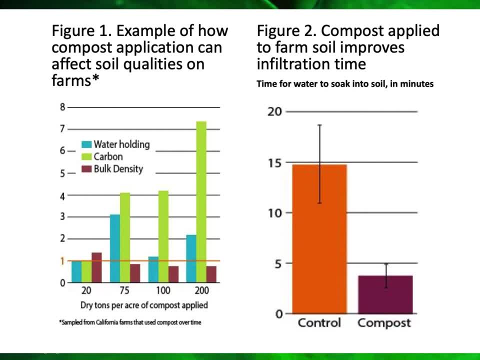 And these graphs illustrate kind of the summary findings. So on the left we can see, you know, more organic matter means the soil will hold more water And the NRCS, the Natural Resource Conservation Service, has estimated that for every 1% increase. 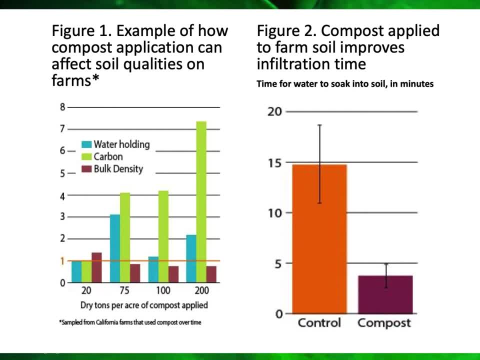 in organic matter in the top 10 inches can hold approximately 27,000 gallons of water per acre. When you now increase the carbon, compost is adding carbon but with that increase in carbon we're seeing a reduction in bulk density. 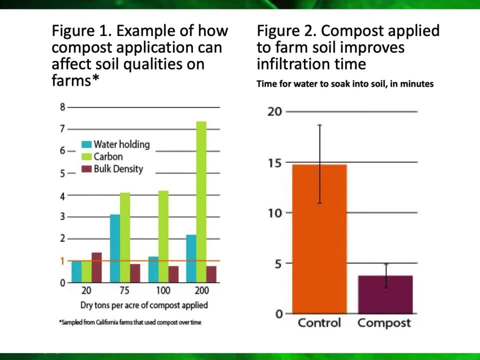 That's because lower bulk density is referring to that added fluffiness or porosity that we get. So we get more pore space means we have more room for the soil to store water And to kind of ensure to higher soil organic matter soil is going to hold more water. 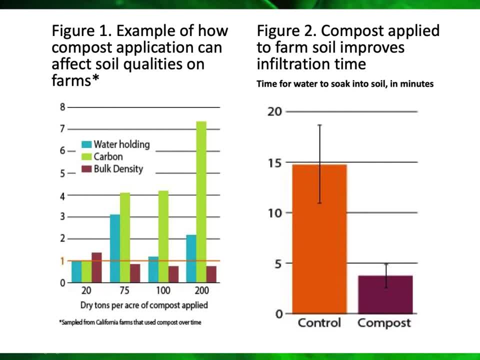 Then a low organic matter soil. on the right hand side we can see how compost allows water to infiltrate or soak into soil faster. So when you have a heavy rain, more water is going to soak into the soil with compost added than if it's not there. 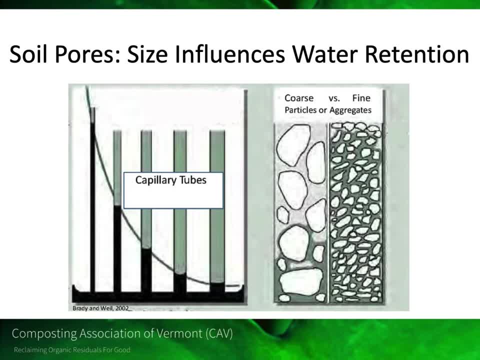 So let's talk a little bit more about this fluffiness or these pores. Okay, So I think of soil. pores really behave a lot like capillary tubes. If that doesn't mean a lot to you, Think about straws, drinking straws, and they come in different widths. 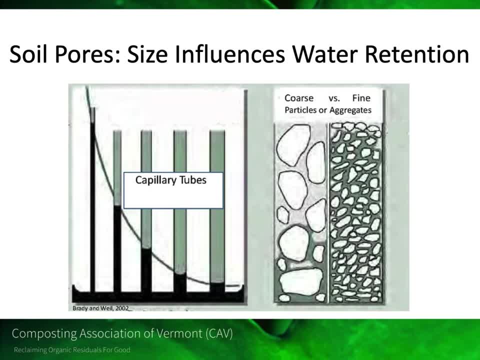 You get thin, narrow ones and you can get fatter ones. Okay, So soil pores kind of act like that, partly because water adheres to surfaces and those that adhesion to the surface will slow down the movement of water and it ends up and 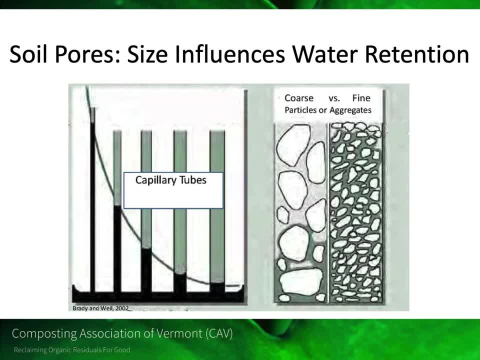 you can see on the left hand panel, the dark colored is the water that the thinner tubes are going to hold the water more tightly. Then the wider tubes- Okay, Wider tubes- are going to drain faster than are the narrow tubes. Now, if the soil pores in soil are so narrow, like we might find in what we call heavy soils, 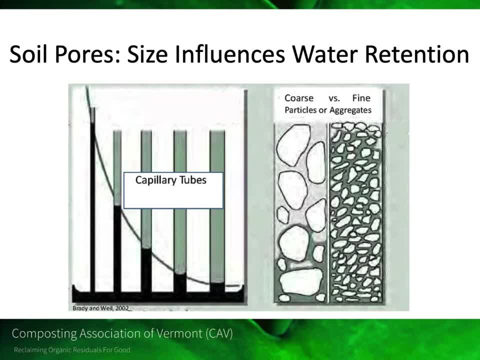 or clay soils. it may have a lot of water there, but the plant cannot extract it because there are so many surfaces that hold that water on so tightly. So you can have water but it might not be available for plants. So a healthy soil is going to have a mixture of these different pore sizes. 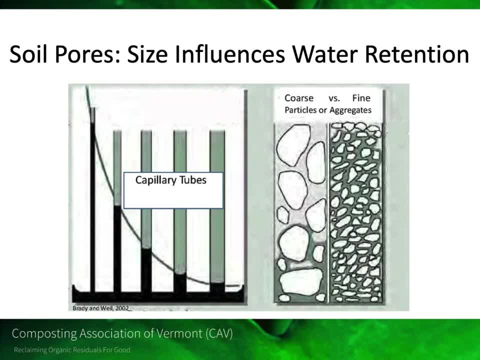 Okay, Because you need some narrowness to keep the water there, but you need some that are wider so that you can extract the water as needed and also have space for all the soil organisms. So you can see kind of pictures of a couple of different types of soil and how the coarse 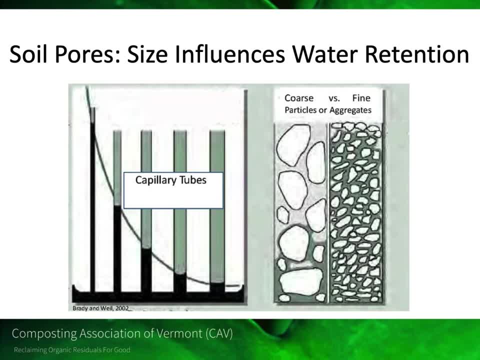 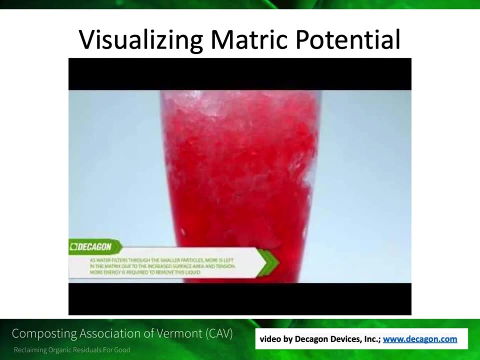 particles have these, the proportionately more wider straws and the fine soils. higher clay would have proportionately more of the thinner straws and hold water very tightly. Okay, In the next slide we're going to have a little video. I think you'll relate to this activity- drinking from a straw- and this is going to illustrate. 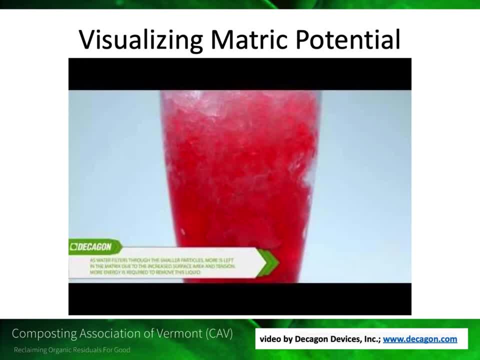 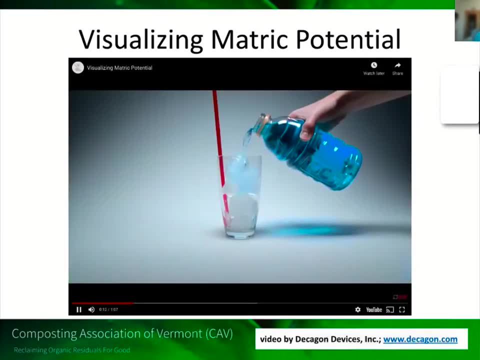 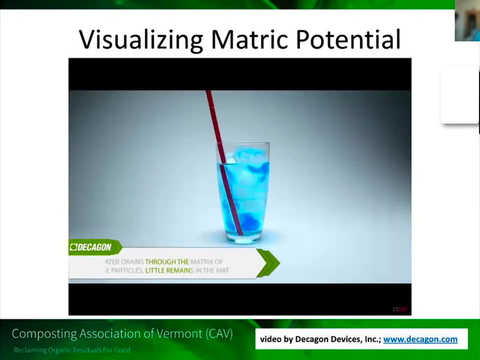 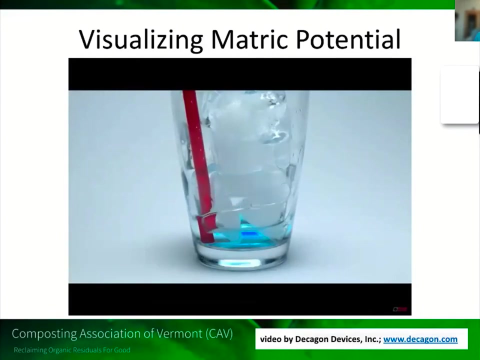 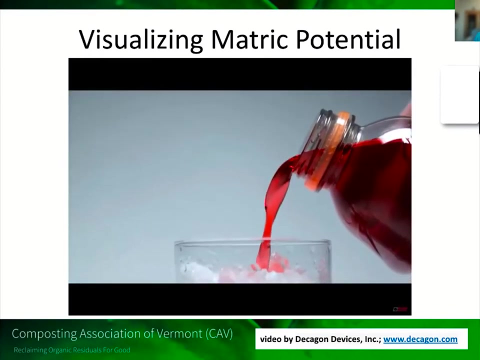 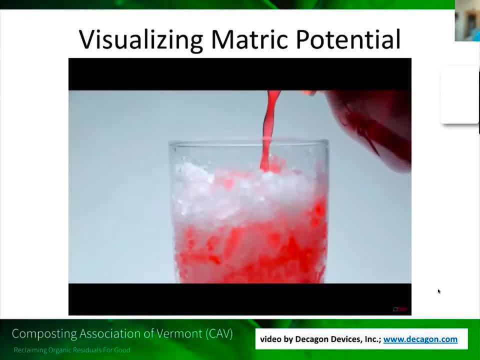 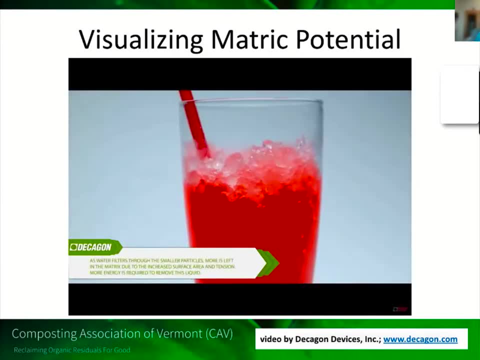 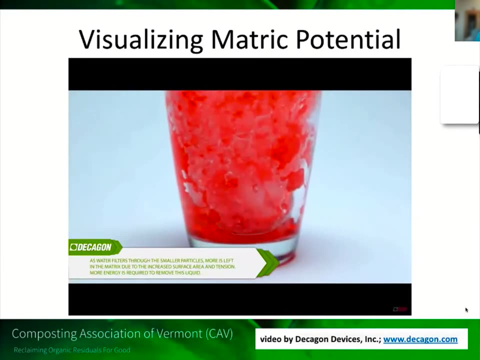 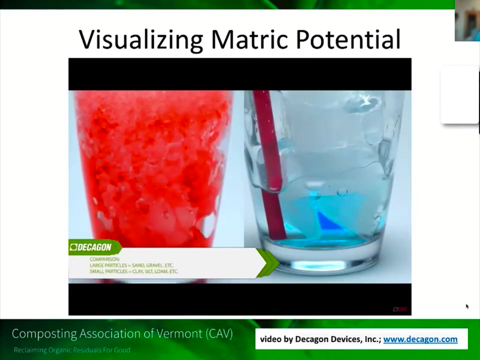 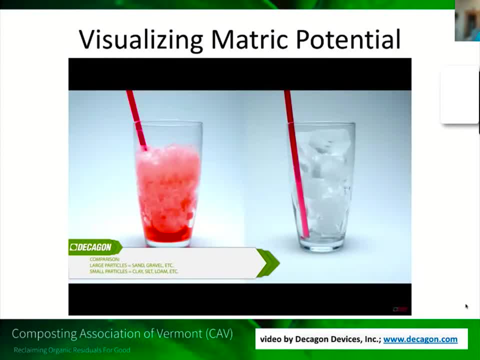 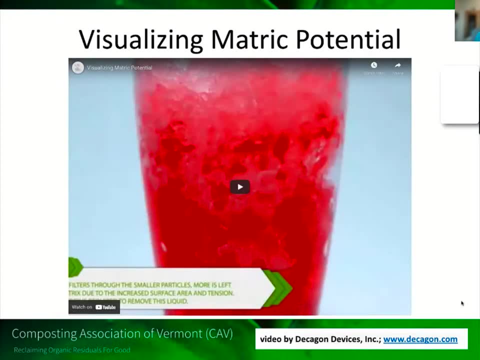 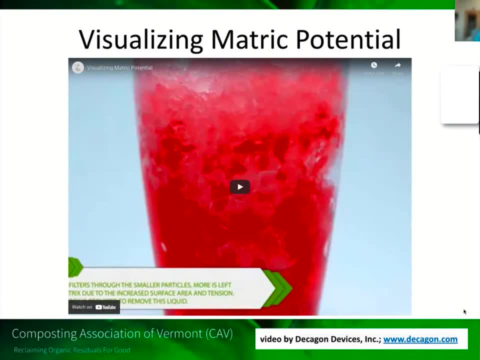 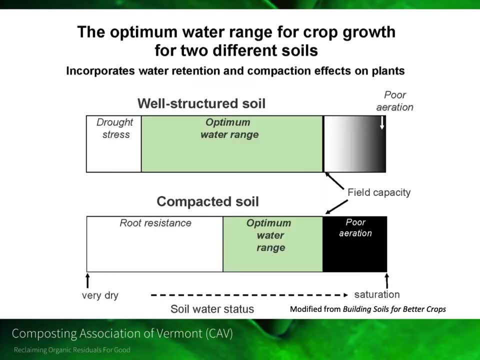 fine, like the crushed ice are going to hold on to that water and you can't, no matter how much suction you have, you still just can't pull it all off. all right, so let's move on and think about kind of, what is the optimum water range? uh, for crop growth for? and we contrast a well. 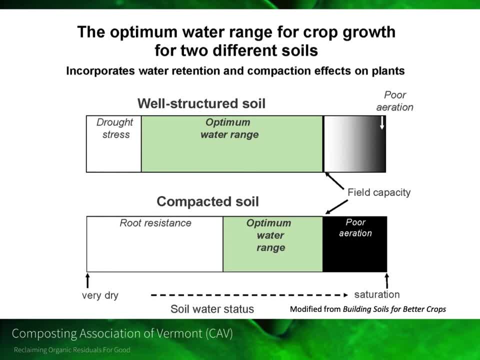 structured soil versus a compacted soil. in the well-structured soil, we can see this balance here, that really a balance between what i'll say- water and oxygen. okay, um, you have kind of this optimal water range, but there's still plenty of pores that are open so that you can get air in there. 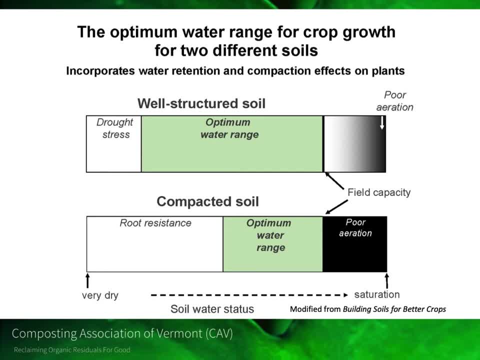 soils are teeming with life and most organisms need oxygen. they need water, but they also need oxygen to breathe, and if you deprive them of oxygen, they're not going to be able to breathe oxygen. it's basically suffocating these organisms. most plants need oxygen there too, in the soil, so 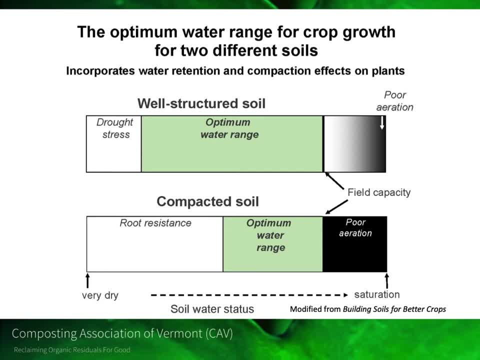 well-structured soil is going to provide, you know, this nice balance. but if we get a compacted soil we get a lot more resistance to plant growth, as you can see on the left-hand side of that panel, and the pore spaces become smaller, like that crushed ice and the water. 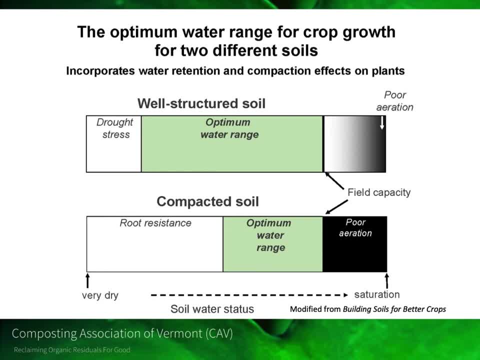 is there, but we can't. those don't drain very fast, so we don't get very much oxygen in there, and so those can become anaerobic. this also affects just who can live there in terms of organisms. if you have a compacted soil, you're going to allow bacteria and fungi to live there. 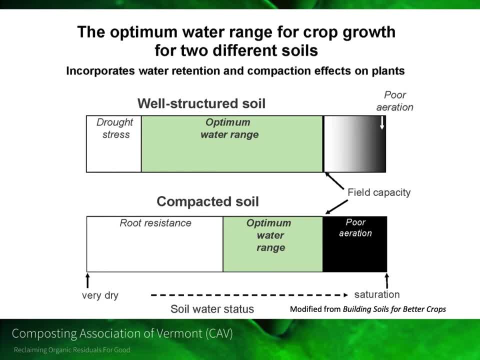 but it would be harder for larger organisms like nematodes or earthworms or micro arthropods to live there, simply because the pore spaces are too small or too compacted for them to get in there. small organisms like nematodes and protozoa. they can't move the particles around, they're stuck with. 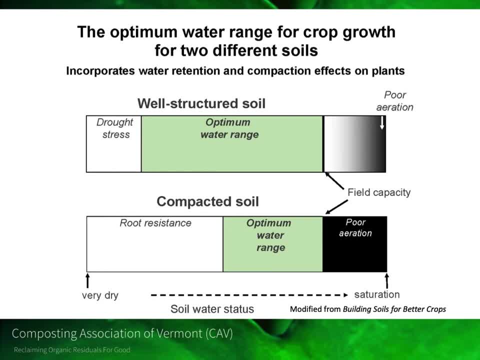 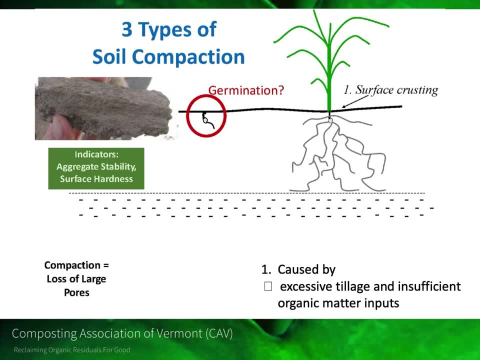 a physical structure. that is there. okay, let's take a closer look at the next slide with the compacted soils and the different kinds of compaction. there's three major types of compaction. before we get into those, i'll just draw your eye to the little green box there. it says indicators. 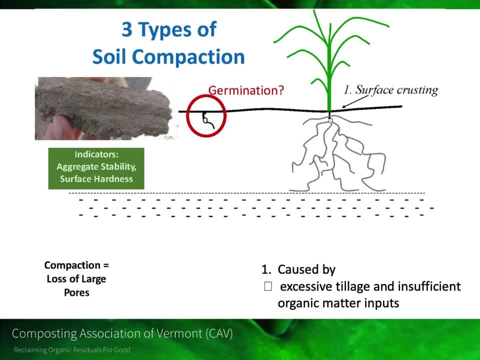 a couple ways that we can measure. compaction is through the measurement of aggregate stability as well as if we look at penetration, which is a measure of surface hardness. so three kinds of compaction. the first is kind of a crusting that surface or physical crusting at the surface. 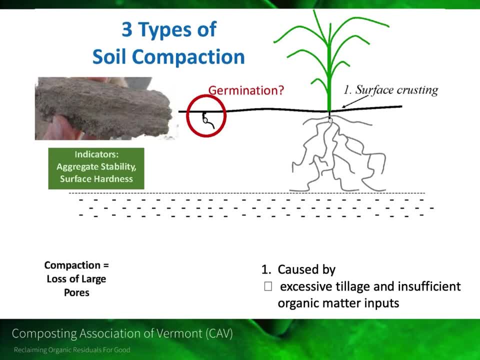 this can happen when the rainfall is hitting a fine layer of particles, and they be there's. they become tightly bound so it almost becomes like a cement cemented surface. there can be less erosion, but it makes it really hard for a germinating seed to make a way. 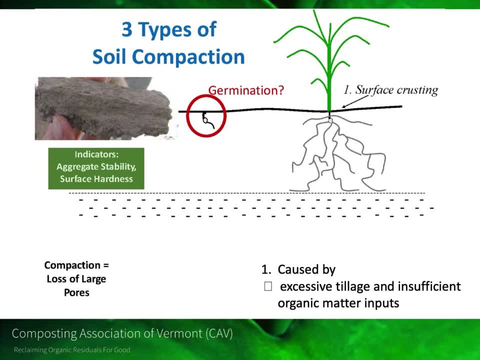 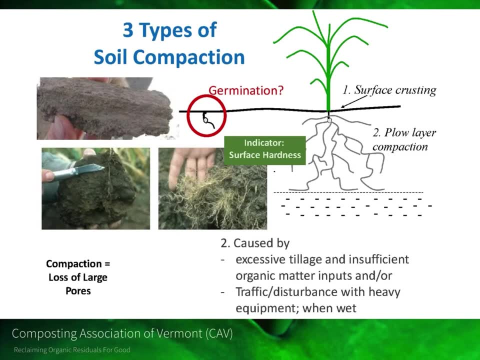 its way through. there. it's caused by excessive tillage and insufficient organic matter inputs. second type of compaction would be called a plow layer compaction and this is a result of, you know, a repeated tillage at the same depth and it can lead to what we call a plow pan. 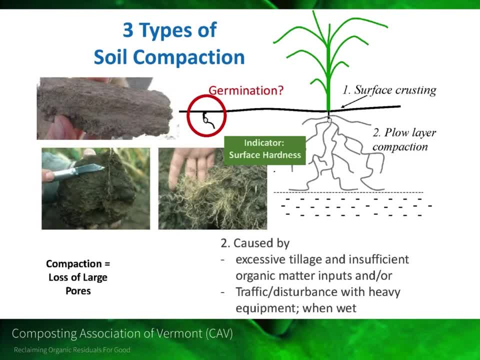 which is just a compacted layer that's right at the depth of the plow implement and the creation of this plow layer compaction can prevent water from infiltrating very deeply and it can also resist root penetration to various depths, making plants more, stressing them out, and 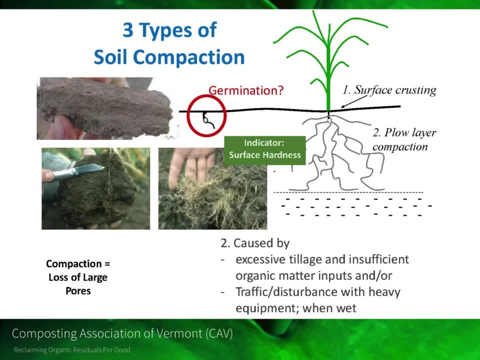 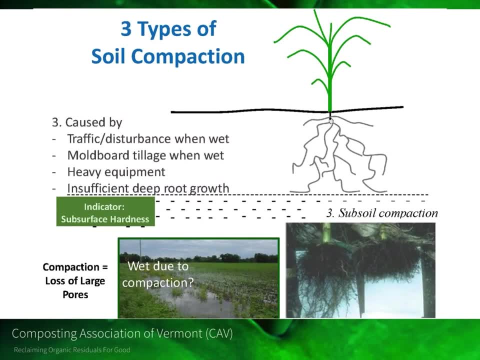 making them more susceptible to drought simply because they don't have access to the reservoirs of water that are at deeper depths. the third type of compaction is called subsurface compaction, and this would be any that would inhibit root growth and penetration that might affect the anchoring of a plant and and reducing access to nutrients and water. 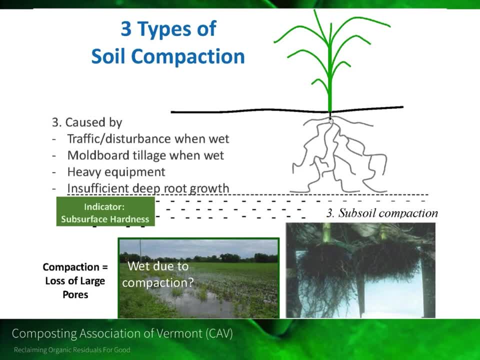 deeper in the soil. so it's just a deeper compaction layer, and it's also going to make plants more susceptible to issues with drought just because they can't access the water. notice on the little picture there, though, in the lower left, that could when we see ponding. 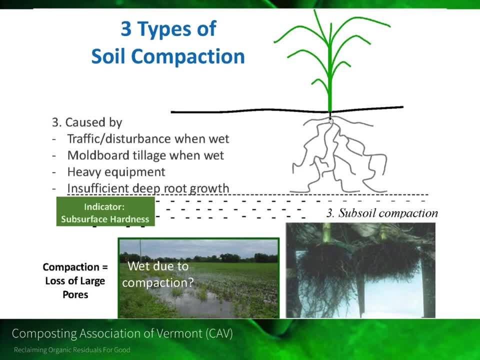 of water on the surface after rain that could be due to compaction, just because the water it's not flowing off, because you don't have the slope but it's not penetrating and infiltrating either. it's just kind of sitting there perched up on this compacted layer and 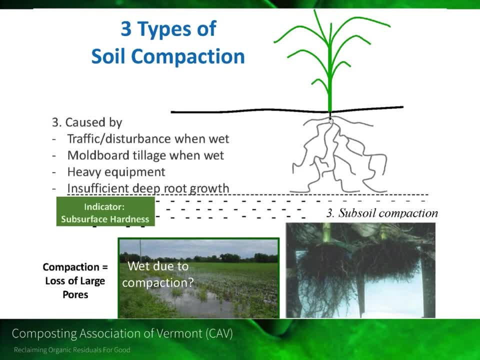 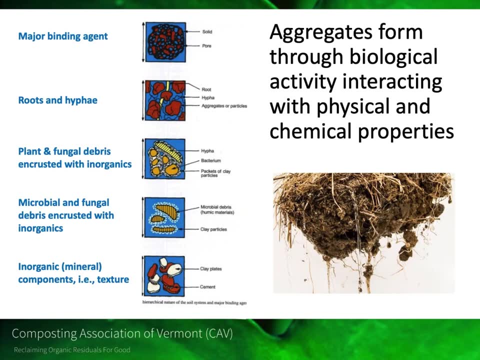 sitting there very long is going to make that system go anaerobic, which is pretty hard on plants and the soil biology. so remember i mentioned aggregates were an ideal indicator for soil health. i just want to, and the reason i say that is they're really a combination. 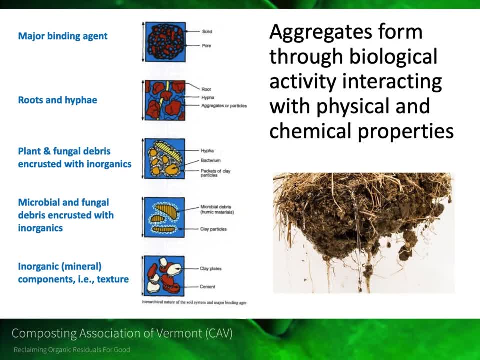 of, or measures of, biological activities that are also interacting with physical and chemical properties. so it's kind of like a whole system in and of itself. so if we go on the left hand side, you can see the components of how a aggregate is made. we start with kind of the 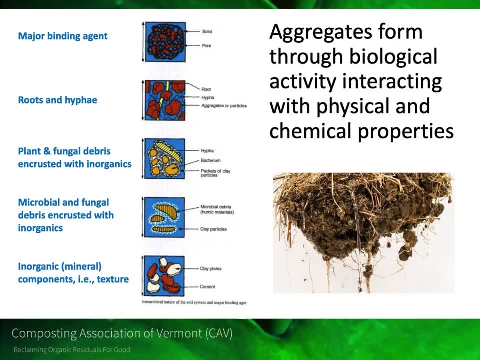 inorganic mineral particles like clay plates, and then those get covered with polysaccharides, that are sugars, kind of complex sugars that bacteria produce. that provides a glue-like substance to hold these materials together and then plant roots and the hyphae of fungi can act like threads to. 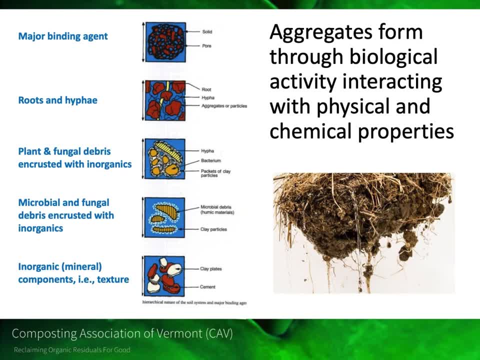 kind of bind these into larger components so that you can see, really it's a combination of the mineral particles. we got the bacteria and fungi as well as roots, and it gives us a heterogeneous structure that's going to allow water infiltration but also pockets of air and force for habitat. here's an actual slice of actual soil that we looked at. 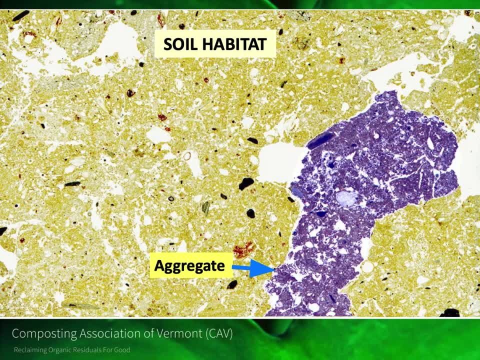 in my lab. that purple color is a bit artificial, but we just did that so you can see what an aggregate actually looks like. you know they- they're not perfect polygons by any means, but i think what i want you to notice is kind of just how porous. 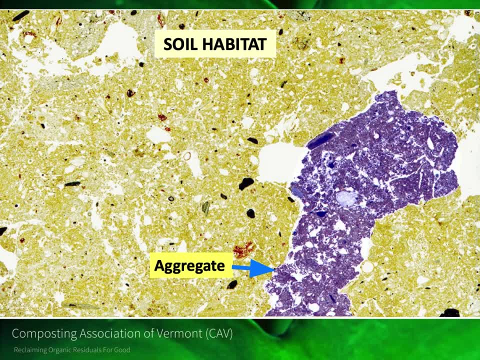 soil is. it's really like a fabric. you know, we look at soil and you can't see through it because it's so opaque and it's gritty and you think about it solid, but it's far from being solid. and if we can start looking at the networks of how those pores connect to each other, 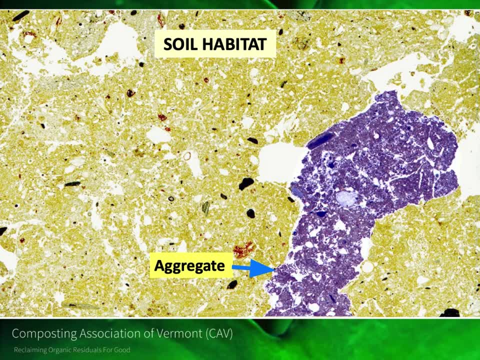 these are actually the highways of how soil organisms move around and disperse within this soil and we can think again of our capillary tubes here. those big open spaces are going to drain faster and if you can look at the victorian000. so the next three slides we'll have are just kind of some. 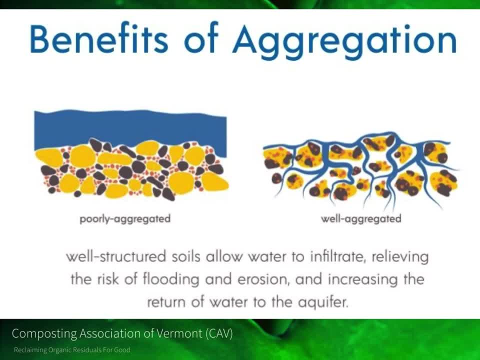 benefits of aggregation. to just kind of illustrate that, this slide just points out how important aggregation is. as you see, well aggregated soils on the right hand side. this allows water to infiltrate, it helps reduce the risk of flooding and erosion and it helps return, increases the return of water to the aquifer where, if we have a poorly aggregated soil, the water is ponding on the. 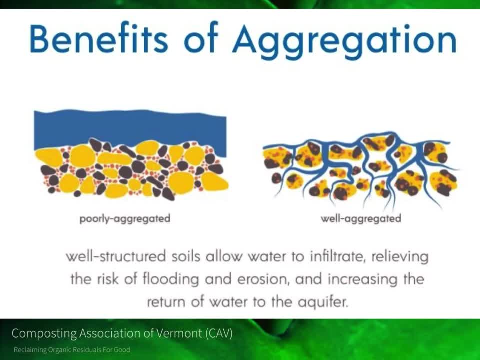 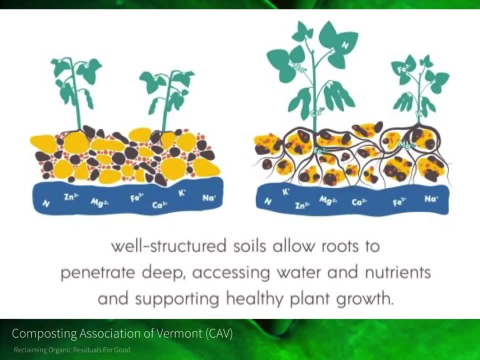 surface or, you know otherwise, eroding and flowing off of that surface, so we're losing the water. well structured soils also allow our roots to penetrate deeply so they can access this water and nutrients, which is especially important in in periods of drought and having deeply deep roots in the soil. 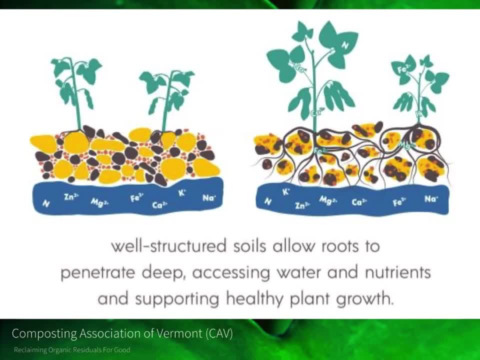 will help anchor those plants and help support healthy plant growth and help reduce stress on that plant so they can be more resilient or resistant to pathogens or other kinds of stress. and well structured soils help provide an optimal environment for the soilṒ. Micro, micro, radio referral capitals- the really key component of their ability to get as much land move. 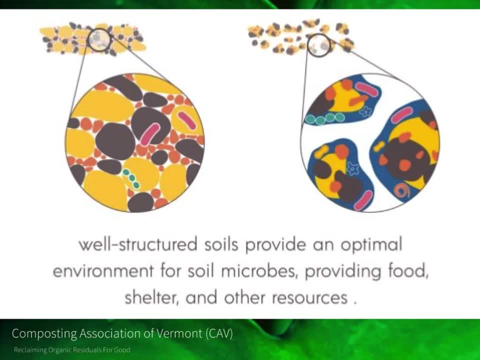 They're providing the food as well as the shelter in these soils. You know aggregates are acting like this whole system right, Integrating biology, physical and chemical. Now we have a short video to kind of demonstrate, you know, how water rainfall in particular, interacts with a well aggregated matrix. 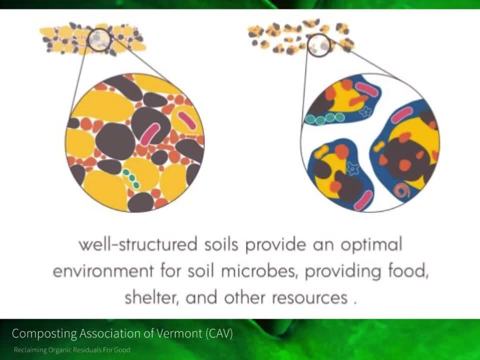 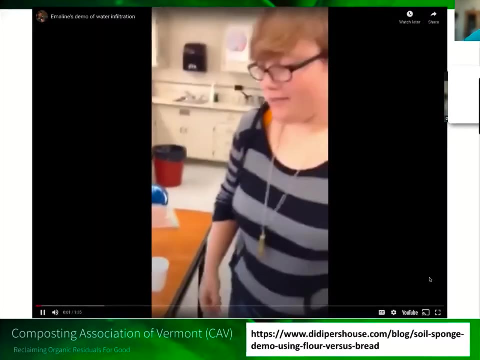 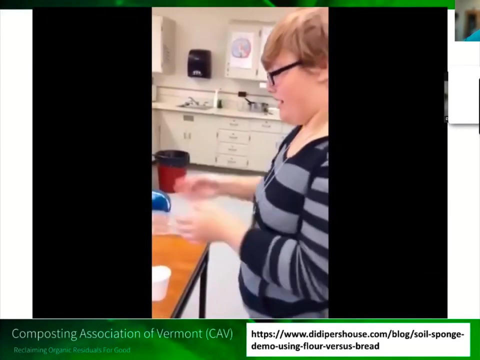 bread versus a poorly aggregated ingredient which is flour, And so we're going to kind of see the role how rain and a well aggregated soil interface. OK, so this is a quick little demonstration just to compare aggregated soil versus unaggregated soil. 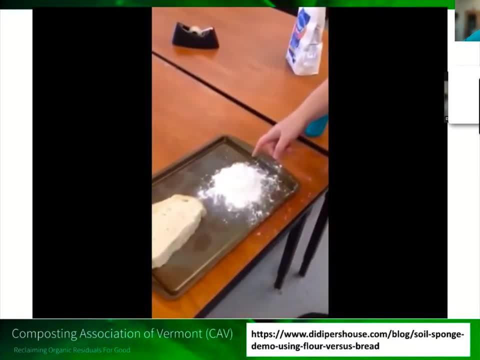 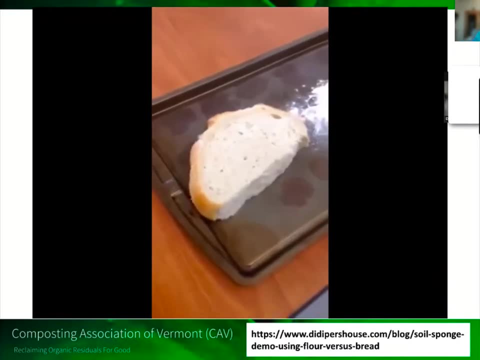 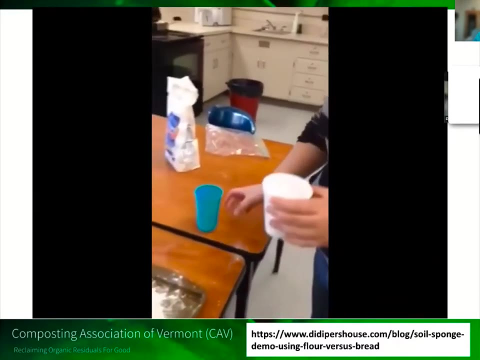 So our flour here represents our poorly aggregated soil, Doesn't have a lot of water, Doesn't have a lot of pore spaces, And our bread has all these nice little pore spaces in it, So our water infiltrates really really well. So this is styrofoam cup, poked a few holes in it to simulate rain. 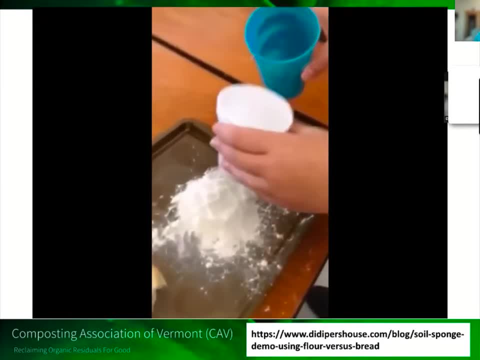 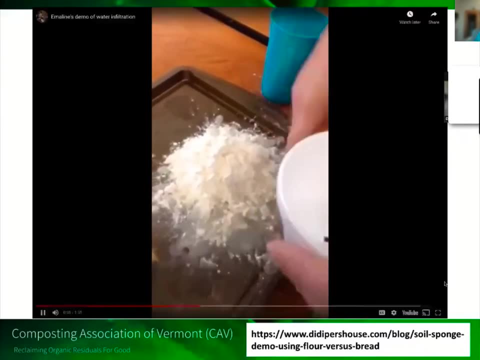 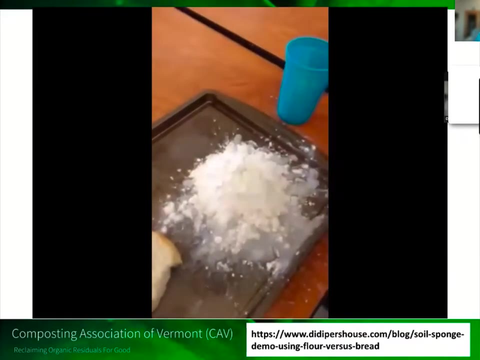 First I'm going to do over the flour, just so you can see. See, just kind of runs right off doesn't really go through. runs off carries all these particles with it, which is what poorly aggregated soil would do if it were to rain naturally. 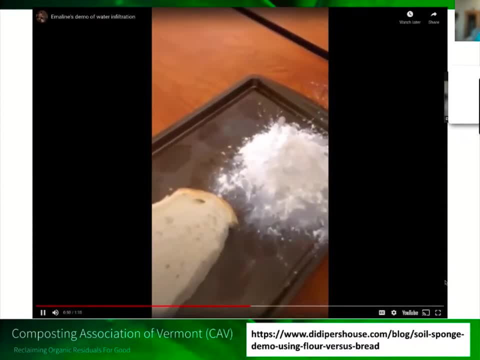 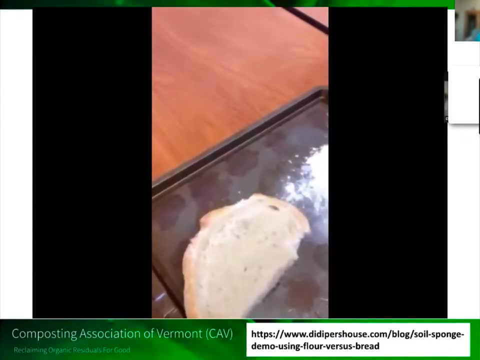 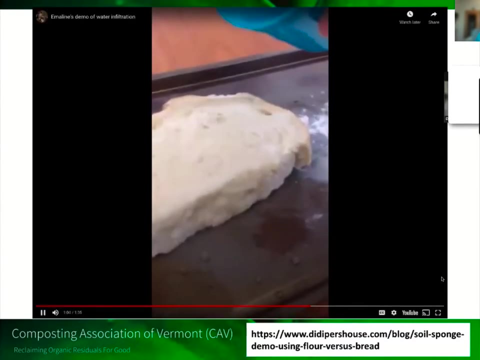 All this stuff would end up in our streams and our lakes and that's not healthy. But over our bread. you can see that most of it is absorbed almost instantly, all the way through. And see, even if it were to rain really heavily or if there were to be a flood, it still enters relatively well. 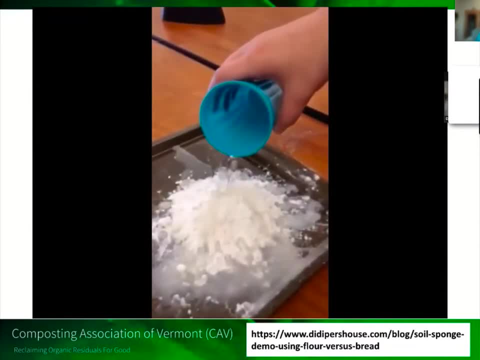 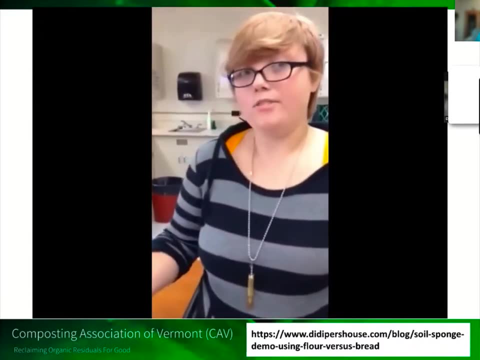 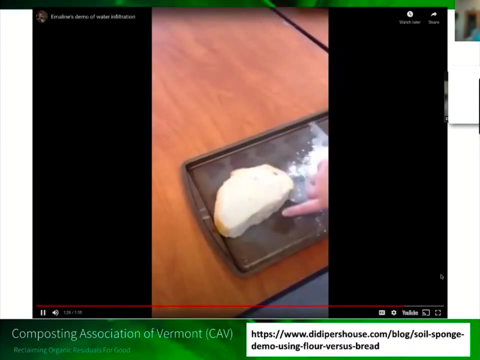 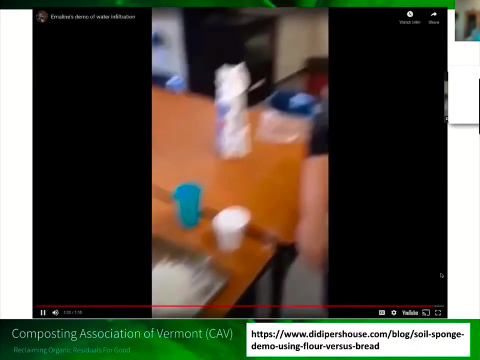 Versus. well, you come back over here to flour, It's just running off and taking everything with it. So that's a quick analogy to see how different soil types would work. So pore spaces, again infiltration. all the way through pore infiltration, everything just kind of runs off. 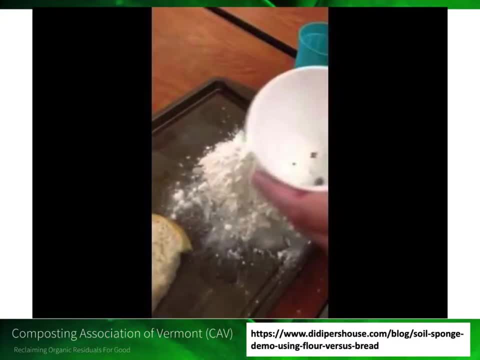 That's pretty much it. So you know, thinking of that video and what's going on, and back to what aggregates are comprised of, you can think of the yeast as really the biological component that's acting like the. it's converting the flour to the bread and it's helped providing the glue, in a sense, to holding that structure together. 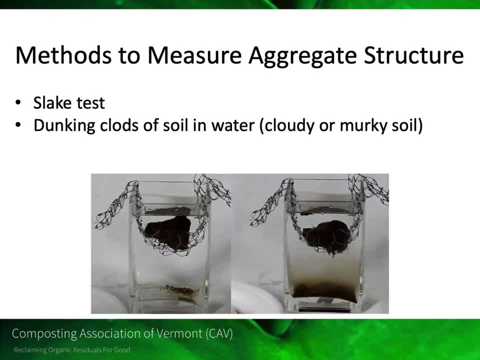 So you know, that's not a real sophisticated method that a commercial soil testing lab might run, but they might run a test that might look like this or this could just be something that makes a nice demonstration about what it will, how a well-aggregated soil works. 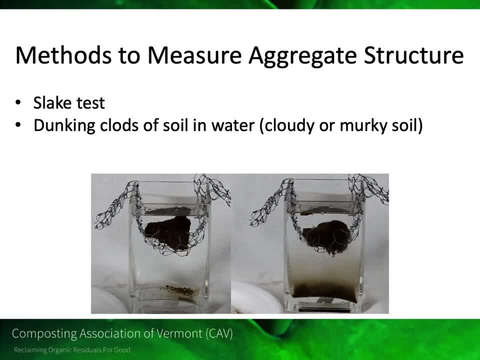 How a well-aggregated soil behaves. This technique is called a slake test And it's basically you're dunking clods of soil in water. If you have a well-structured soil, once you put it in water it's just going to be like on the left-hand side. 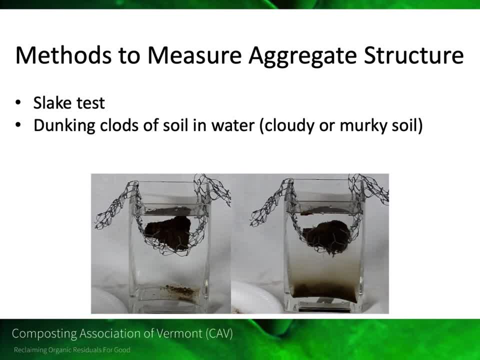 You're not going to see many particles coming off. But if you have a poorly structured, poorly aggregated water or soil, it will look like on the right And you're going to start to see soil particles leaving that and making the- you know the water very murky and cloudy. 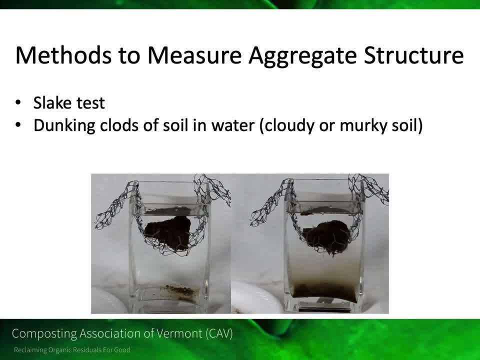 I've seen this kind of idea even demonstrated in an egg carton, where they're putting clods of soil into each compartment where an egg would be and then adding water And you can see how well that clump of soil maintains its structural integrity. 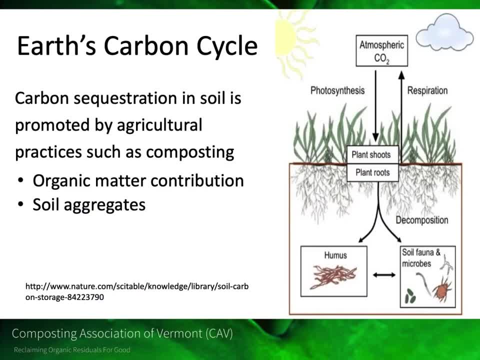 or if it just starts to dissolve in the water. So the next cycle we want to focus on that relates really well to compost is the carbon cycle, Because what compost is all about is the carbon cycle. What compost is all about is a controlled and regulated decomposition process. 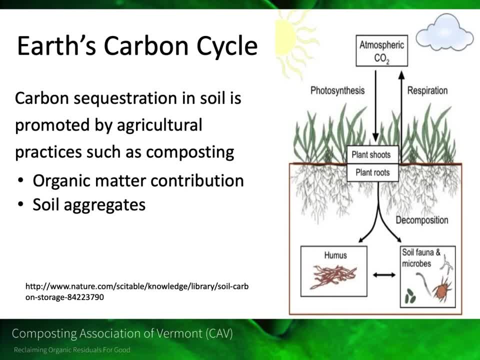 And that's all about carbon. Carbon also connects us with climate change and carbon sequestration. So by having compost and adding carbon to the soil, we're getting more of that carbon in there. Carbon is really how, the connection between the above and the below ground. 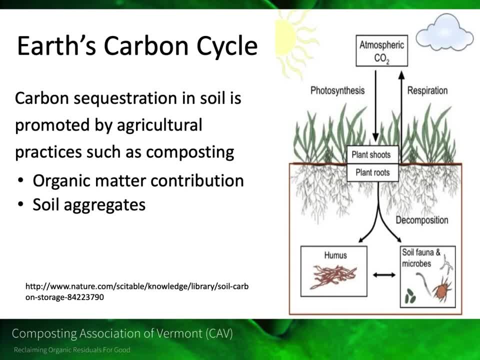 We have atmospheric carbon. that's fixed through photosynthesis into sugars by plants. The plants are putting those roots in. The plants are putting those roots into the soil. Roots are the basic source of carbon to the soil food web. So that's the base of the soil food web, or plant roots a source of carbon. 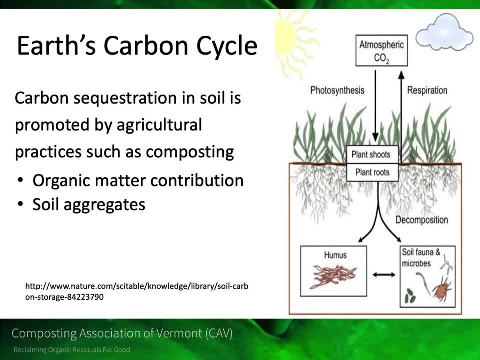 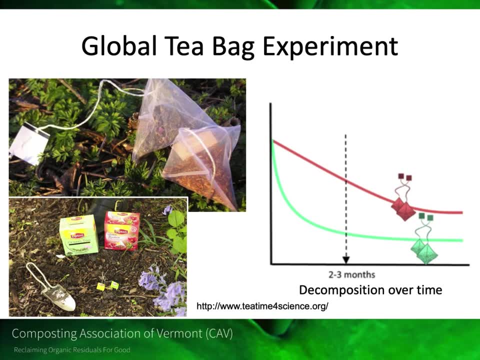 Carbon in this case. you know you can think of it as food, but I often think about it as more as energy. It's kind of a currency, so to speak. There's kind of a. there's a cool citizen science project being performed globally with tea bags. 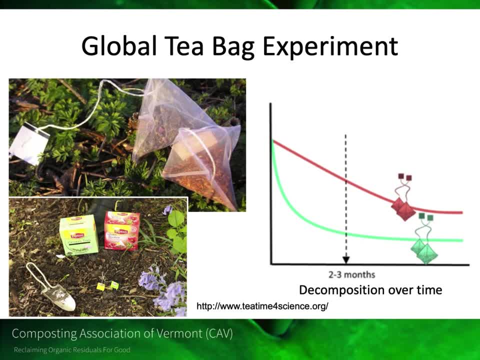 that are a way of illustrating decomposition. You know, by the way, I think of decomposition is a super critical process, probably right behind photosynthesis. You have to have photosynthesis to fix CO2, but we need a decomposition to be doing recycling for us. 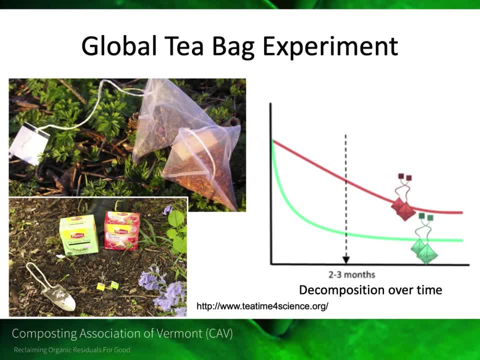 If not we would just we would be buried in detritus and trash so forth. So decomposition is a super important process. So in this project they've done a citizen science kind of. to standardize it across the globe Is to have participants by two kinds of tea. 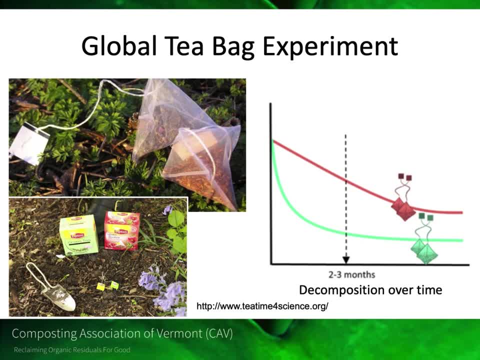 They have to use the same brand of tea But so that we have a constant. One is green tea and the other is a rooibos tea And these two teas decompose at different rates And the graph on the right kind of shows you that the green tea decomposes very rapidly at the beginning. 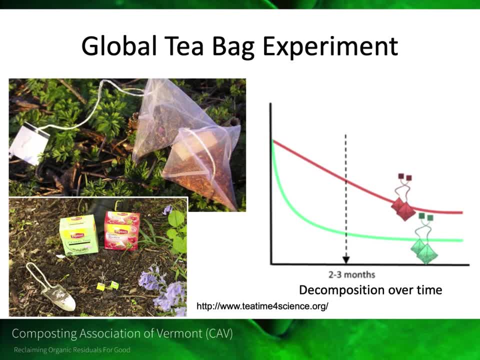 because it contains a lot of components that are easily decomposed, like starches or the cellulose materials. In contrast, the rooibos tea contains substances that decay more or more recalcitrant to decay or decay more slowly, and would contain more of the lignin compounds. 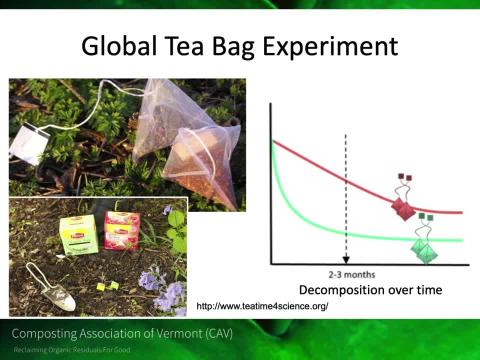 If you're interested at all in learning more about this particular project, I left the URL for the site where you can learn more about that. Now you know, in compost we don't want to promote these non decomposable, non compostable bags that you see here. 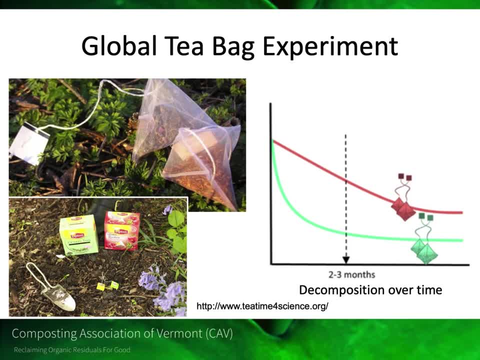 That's an issue, But I'll have to say sometimes we make sacrifices for science because they're wanting to actually measure the changes in weight loss. You know, carbon is the backbone of life And you have a substrate there. as they get, the microbes are converting it to carbon dioxide and the weight goes down. 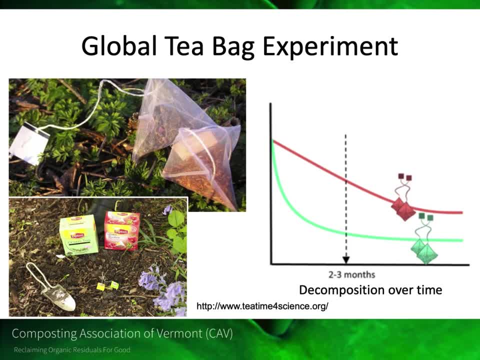 If we had a bag that decompose, we'd never be able to weigh it through time because our container would go away. So in this case we're just doing it for the sake of science. I just was remembering. There's also another fun one. 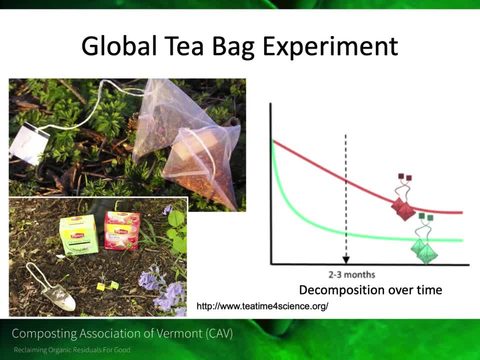 It's called the underpants test, And so you can take, you know, a pair of underwear. You want the 100 percent cotton ones, but you can have the full integrity. and then you bury them for a while and then you can figure out. you can see how those decompose. 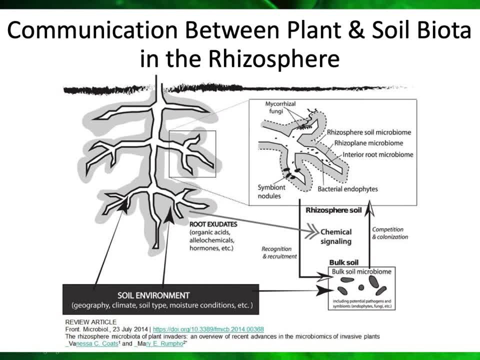 Next, let's look at what's going on with this carbon flow in the soil And the big action is happening in what we call the soil, What we call this rhizosphere. This is the interface between the plant roots and all of the food web in the soil. 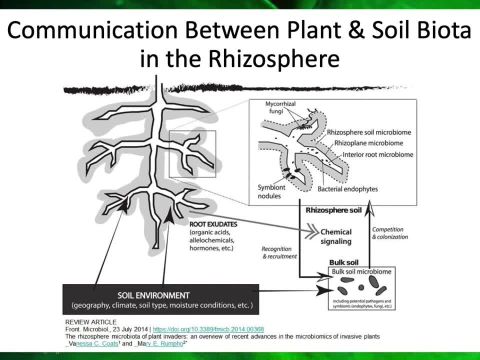 What is defined as the rhizosphere is this area right around the roots and is designated here in the gray color. As a soil ecologist, we usually think of this as what I call a hotspot of activity. You know, there's certain regions that are kind of islands of activity within soil. 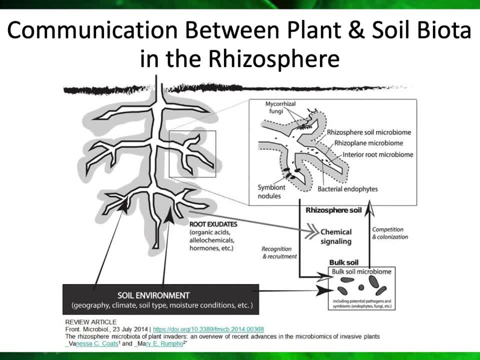 The distribution, spatial distribution of organisms in soil is very aggregated And one of those zones of higher aggregation Is around plant roots. It ends up that plants leak out like up to 50 percent of their carbon through the roots. Roots are very leaky. They're not only leaking carbon but also amino acids. 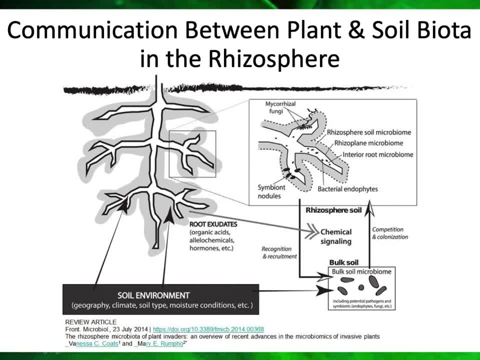 And you might think, is this normal? Yes, it is a normal natural process, because this leakage provides lubrication for a root growth in soil, because the root has to be working its way down into the soil. OK, But you know it. 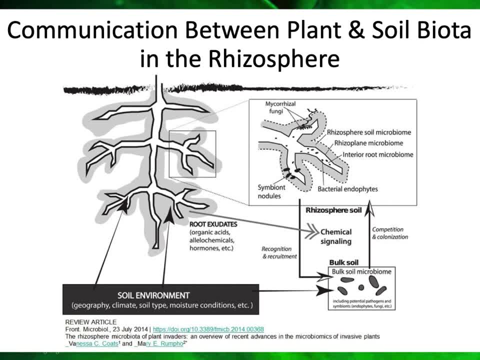 But you know, an indirect result of this leakage of sugars and amino acids is this is providing the energy and nutrients to support the soil food web. And it so happens in this zone, this gray zone that we see, is a lot of communication, chemical communication between plants and microbes. 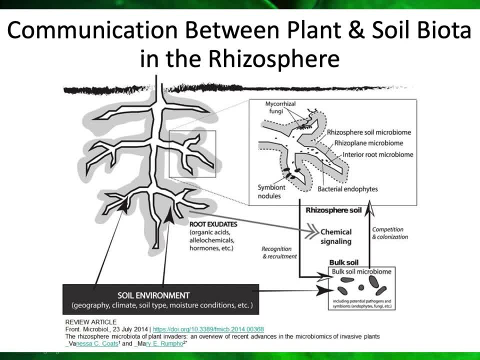 And they're communicating through hormonal or other chemical signals. And that's kind of a hot area of research right now is trying to be able to measure and understand those signals that are going on And understanding who's driving the ship. Is it the plant or is it the microbes? 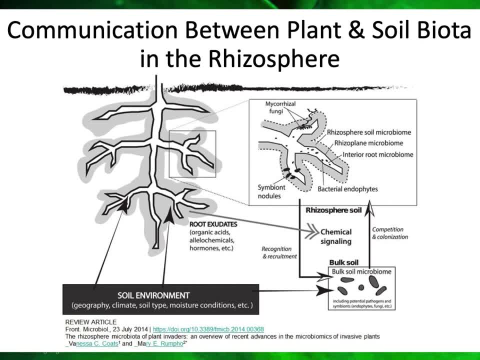 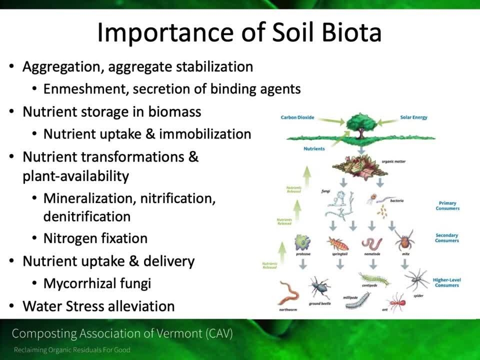 We also see microbe-microbe interactions there too. So this is the rhizosphere. OK, so just to kind of review and recap. biological organisms play many critical roles in soil And we see those listed here. We have this structural aggregation, nutrient storage and transformations of nutrients, nutrient uptake and delivery, as well as alleviation of water stress. 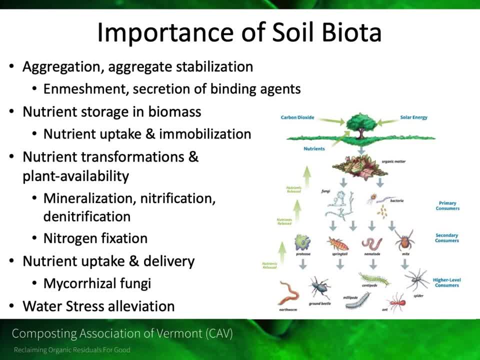 And without the biomechanics And without the biology in life and soil, these functions would not happen. These are all mediated by soil soil biology. On the right hand side you get a sense of how complex that soil food web can be. 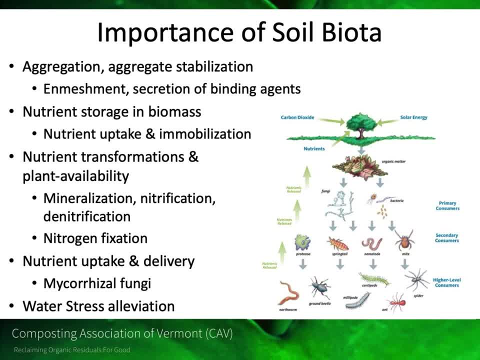 And, like any food chain or food web, we have different levels in the food chain. We have, you know, the, the plant roots. We've got primary consumer, secondary and higher level consumers And I would say a healthy soil is really one that contains these different levels and has a complex. 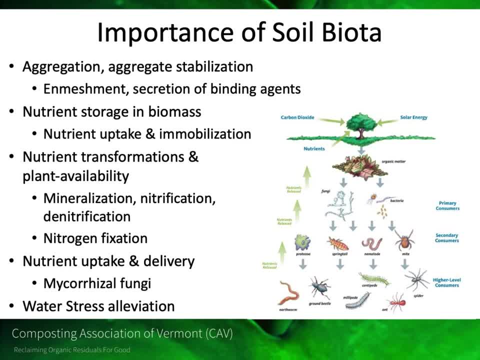 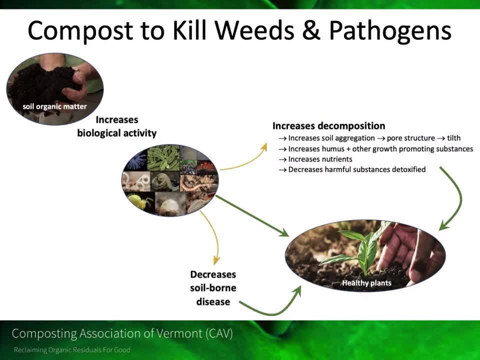 Food web, And by having these multiple levels, you get more regulation, stabilization and resilience within that system. All right, So now we're ready to move on to part two, which is related to looking at disease suppression. This is an area of research I started. 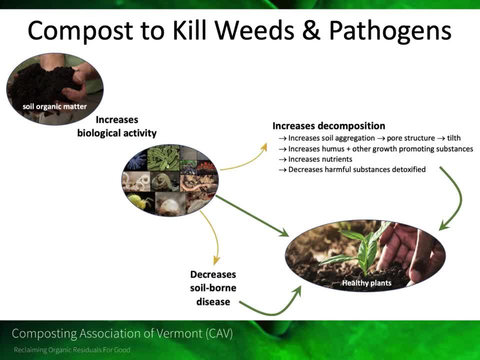 I think it's almost about 10 years ago. I kind of lose track of time, But during that time there was a really severe early blight epidemic. This is a disease that can goes on solanaceous plants like tomatoes, potatoes. 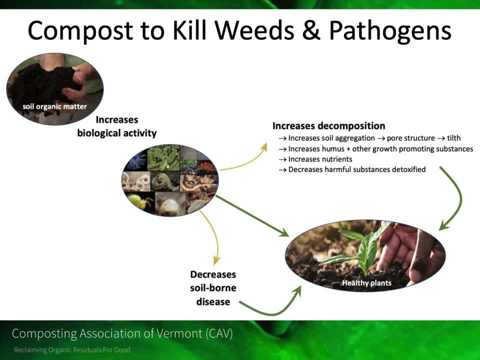 And it's caused by a fungus called alternaria. Well, farmers were asking extension agents what to do with these disease plants and were being told to toss them into the landfill. I was like, oh really, If we do composting properly, we should be able to kill pathogens. 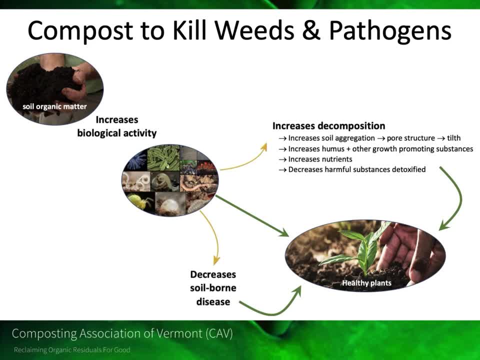 And I added weed seeds here too. by doing that properly And by using composting, we could keep the nutrients on farm and help close the loop. So I embarked on a project Then with Highfield Center for Composting. that's now changed hands and reformed. 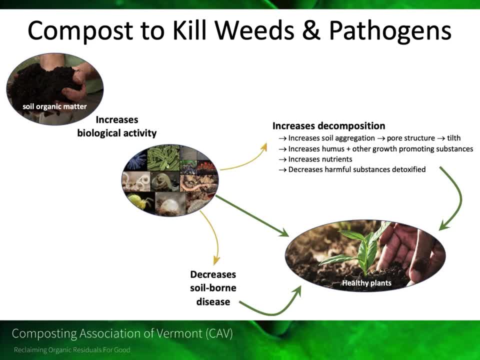 But I just want to say that was a really important partnership in getting me into compost research. We see the soil, organic matter. That's where the biology is happening And the processes that the organisms are doing. they're involved in decomposition. You can see those listed as bullets. 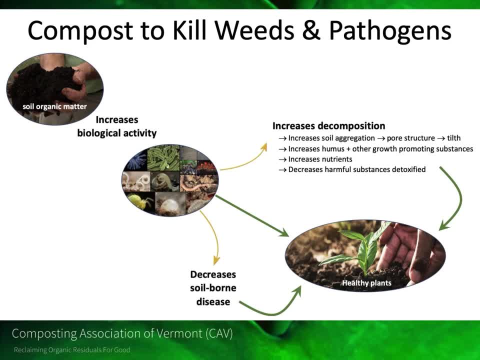 They're increasing aggregation which influences the pore structure, the humus nutrients, And then what I'm getting to is this: This decreases soil borne diseases- OK, those- because those microbes can be antagonizing. There's a lot of beneficial microbes in the soil that can help promote plant growth, either through producing hormones or triggering that, or just simply antagonizing or competing with plant pathogens. 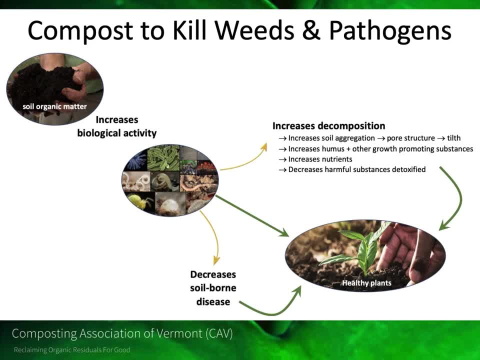 And when we start to explore this, it's a bit like thinking about the gut microbiome that you hear a lot about. We're starting to see this kind of phenomenon of a consortium and community interactions And soil around plant roots. So what do I mean by proper composting? 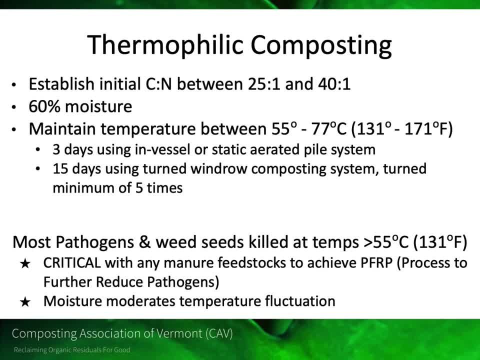 What I'm referring to is thermophilic composting, And I'll just you know, stayed up front, that this is not easily achieved in the backyard, in a backyard pile. This is you know. you need a pile that's more like 15 cubic yards or more at the commercial scale to be able to achieve this, just with the mass. 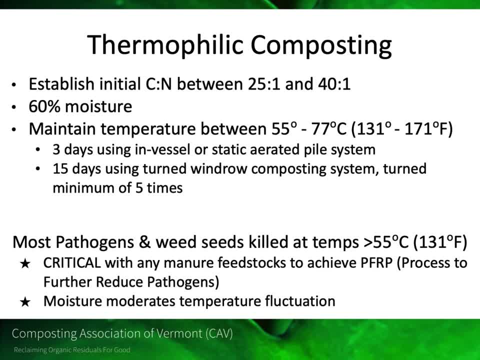 But you know backyard composting, You know what's going into that. But if you're a commercial producer, you're dealing with materials coming, you know, from other sources And you're also likely to be including, especially at our state- manure into those. 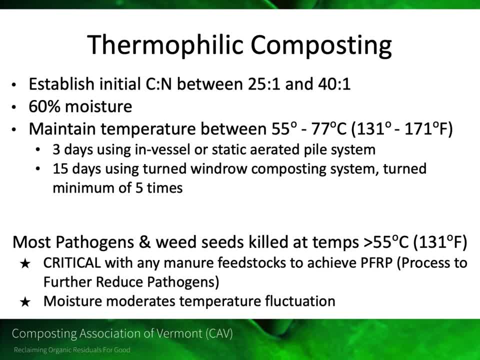 And we want to make sure that we have a good kill on human and plant pathogens. So when I'm talking about proper composting technique, it's employing a thermophilic compost. How do we do that? OK, so remember, soil is alive. 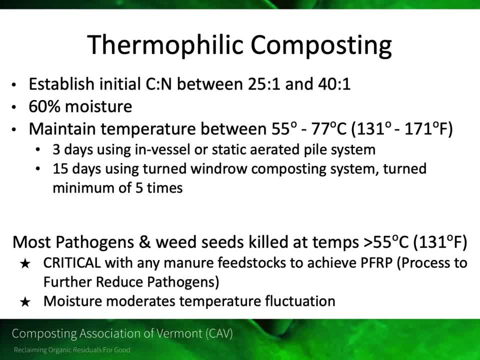 Compost is alive If you're living. you need air, You need water and you need nutrients and you need a right balance of that to thrive. So that's the key. So you need a carbon to nitrogen ratio that's somewhere between 25 to one to 40 to one. 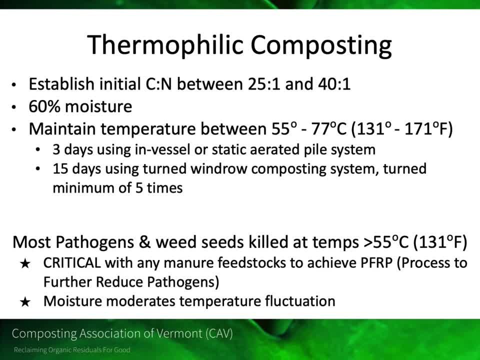 This helps, gives you the structure and helps give you a balance of the nutrients and the energy. You have to have a percentage moisture, but you don't want it too wet because you've got to have some air spaces so those organisms can breathe. So if you get the recipe set up there so the microbes can really kick in and be active there. when they're active they're going to be respiring. 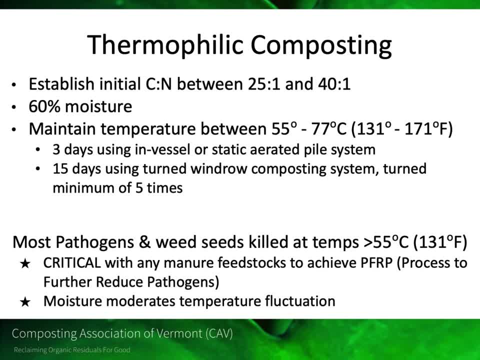 And that respiration is what increases the temperature And that's what you're trying to foster, getting that temperature up there to 55 to 77 degrees Celsius, which translates into about 130 to 170 degrees Fahrenheit. Another key thing to maintaining that oxygen: 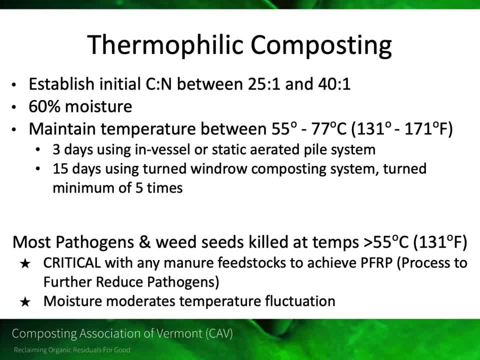 And you know flow is to be, you know is the time and the turning, And it depends on what kind of system you have to what the guidelines are. If you have an in vessel or static aerated pile system, you need a minimum of three days. 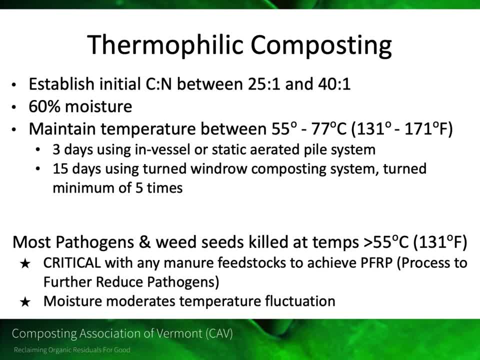 If it's a windrow system, if the recommendation is to turn it a minimum of five times and have it at those temperatures for at least 15 days. Now, there are some variations on this theme. You know whether it's coming out of the National Organic Standards or the PFRP, etc. 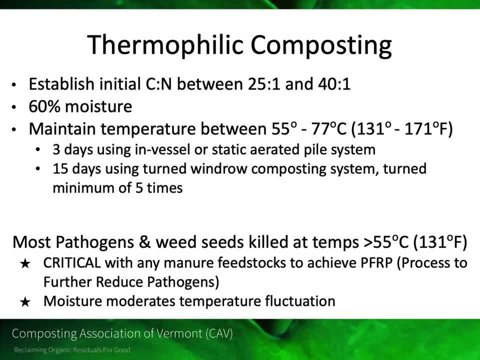 But the whole idea here is really trying to achieve temperatures that you know are going to be lethal to these pathogens and weed seeds. So I embarked on this project. Actually, we wanted to look at if we did proper conservation. We wanted to look at if we did proper conservation. 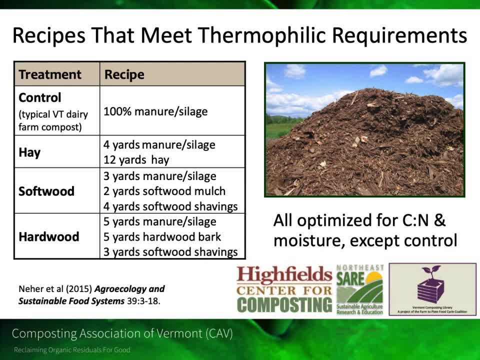 We wanted to look at. if we did proper composting, Could we indeed kill those plant pathogens that they had foreseen that were so bad that year? One thing that's missing from the guidelines is what kind of carbon. It just says carbon to nitrogen, as if carbons are all alike, but they're not. 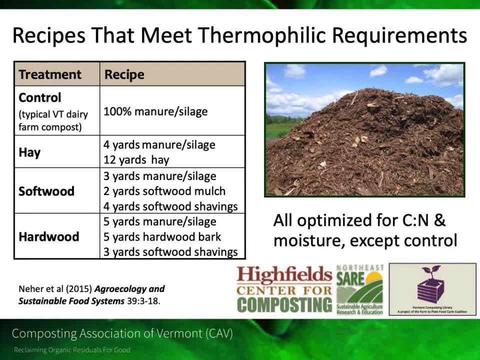 There are some carbons that break down a lot faster, like hay- than others, like wood. Wood is a lot slower And we know from research coming out of the 1980s that some of the disease suppressive compost included hardwood and or bark in that. 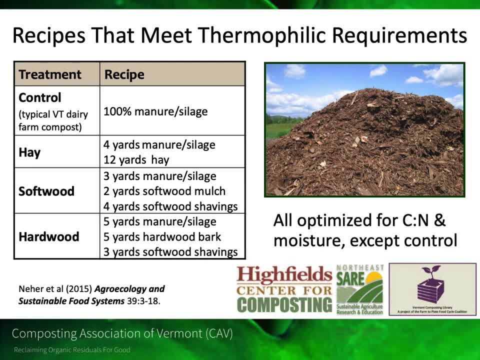 So we wanted to make sure, since our focus was on diseases, to include that as an option. So we established recipes that met the C to N ratio in the moisture with three types of carbon, whether it's hay, softwood or hardwood. 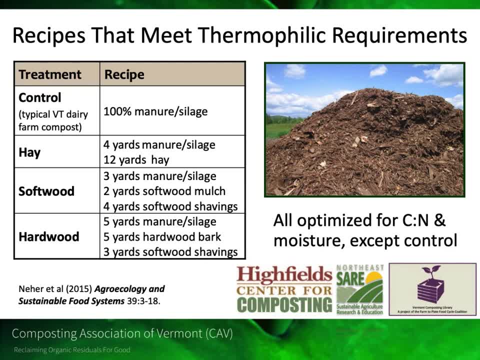 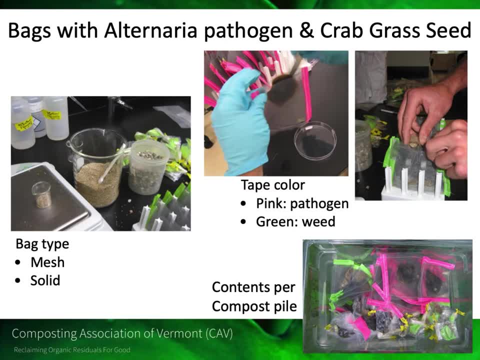 And we used to control that a Vermont dairy farmer would use, which would just be like a mixture of the manure and silage coming out of the back of the barn in the spring. Then we created this. Then we created some bags of a plant pathogen, the Alternaria pathogen, and some bags with giant crabgrass seed. 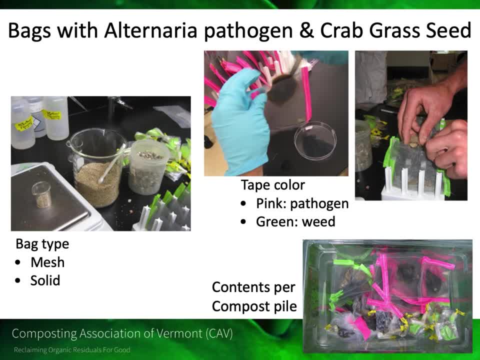 We chose that weed seed just because it's such a large seed, And if we could kill it, then we- you know we're just being conservative. So we used two different bag types: One was mesh and one was solid. The solid bag would allow these to only be exposed to temperature. 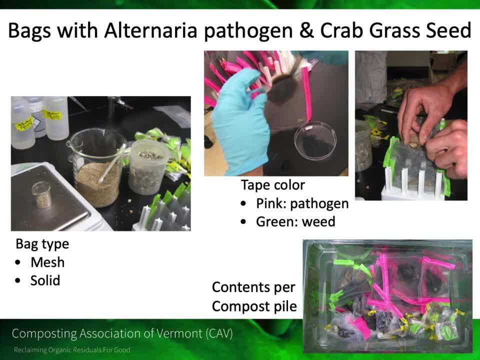 The mesh bag would allow not only temperature but also the microbes to interact with the material. And then we added some flagging tape, sewed it on there so we could find these at different points of the composting and pull them out of the piles. 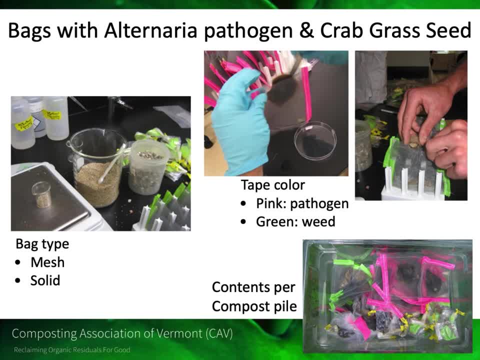 And so we have- I don't know. there's 30 to 50 bags there that we put into each of the compost piles And we marked the pathogen as pink and the weed seeds as green. Then we mixed these into the compost. 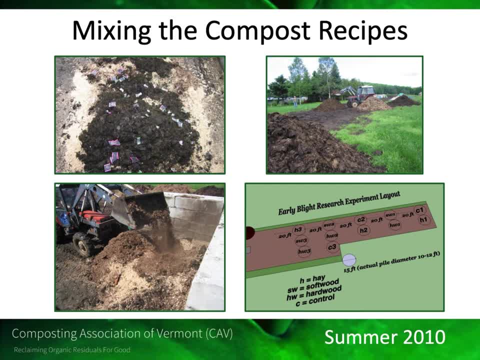 And you can see us doing this. This is at Highfields And this was a replicated trial And you can see the multiple piles there in the background. And so we pulled out bags of the weed, seed and pathogens at. you know, at the beginning and at various time points during the process of reaching these thermophilic requirements and curing. 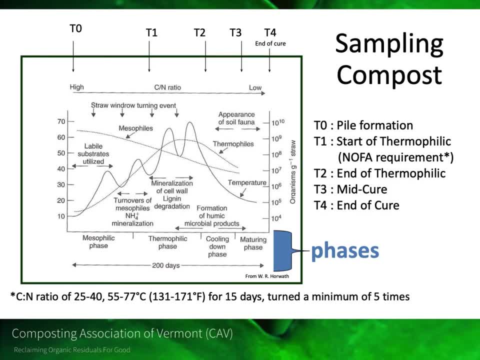 So here's kind of an illustration of our sampling regime. These were all windrow based, so we made sure they returned a minimum of five times Along the top. there you see T0. That's the first time. T1, T2, T3, and T4. 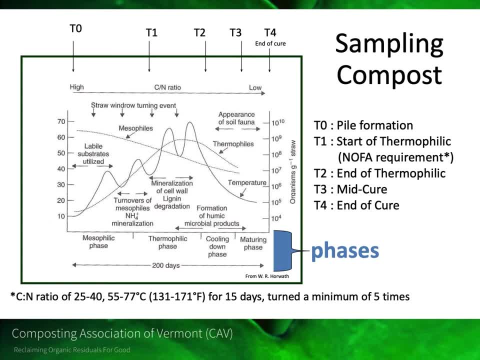 T1 is referring to the time of compost that would match the NOFA requirements, The Northeast Organic Farming Association saying that should be enough for pathogen kill. The stages 2,, 3, and 4 are different stages of maturation and curing. 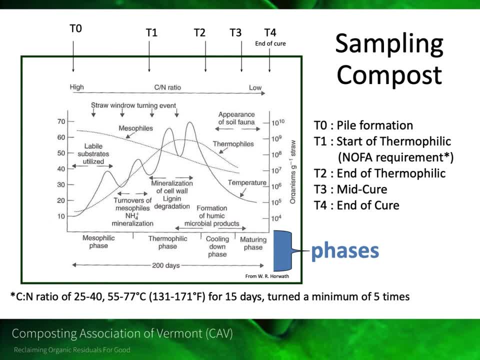 This is a very complicated graph but you know it does show some of the lines that go up and down like a camel's hump in the middle. We're referring to the temperature. It changes and you can see how that goes up at the beginning. 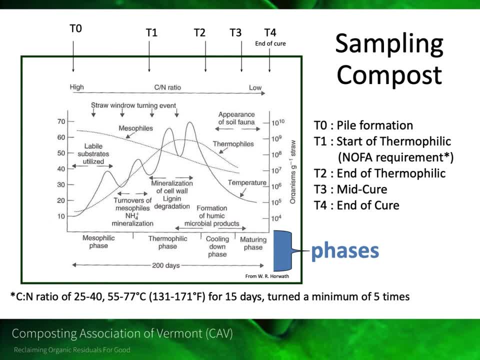 And then the thermophilic phase is when it's really high. But when they dip is because you know oxygen is becoming limited. But once it gets turned, that temperature goes back up again And eventually you don't see that increase and it just declines. 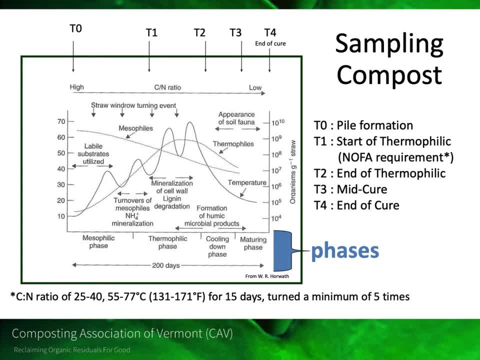 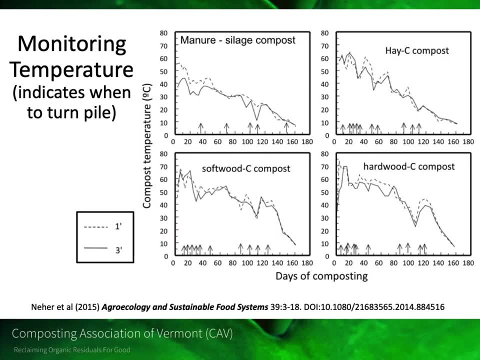 And that would be the cooling and maturation phase. So I'm going to refer to these T0 to T4 time points in the next few slides. It's always important, if you're doing proper composting, to be monitoring the temperature, And so we were monitoring temperature at one foot and three feet, and those are illustrated here. 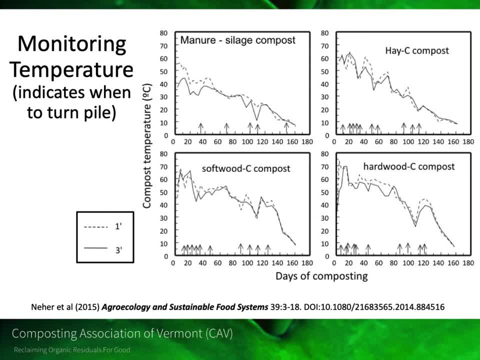 They're plotted versus Celsius, So you have to bear with me if you're used to thinking in Fahrenheit. The little arrows along the X axis are related to the times that we turned the pile, And so we were basing that based on how those temperatures were going. 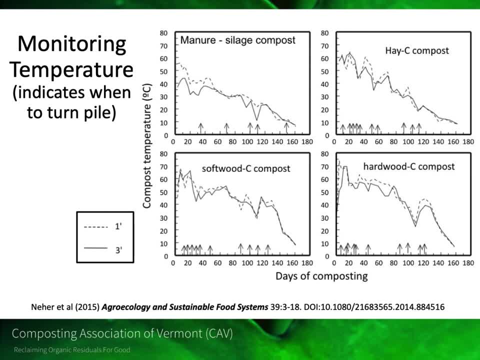 And that way we could keep track that we were following the recommendations for the turns related to temperature. So we're going to keep track of that. So we're going to keep track of that, And then we're going to keep track of the temperatures related to temperature. 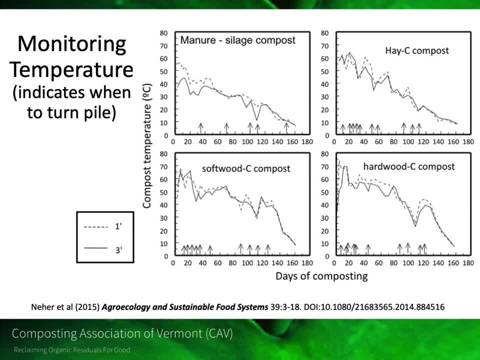 Just a couple of things to note here. One is noting that the temperatures got the hottest in the hardwood over on the lower right-hand side, And they reach those temperatures really fast. Okay, Softwood was the second highest, Hay was the cool was cooler. 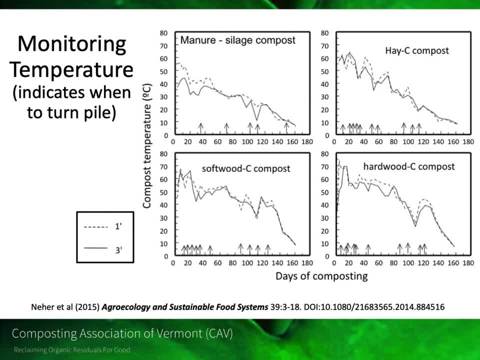 Okay, Just put in your your thinking about how to build a good fire. Your hot fire is with those woods. If you had a hardwood in there, you're going to have a nice good fire. Okay, hot fire. but if you're burning straw and hay, uh you know, for your fire it might be hot for a while. 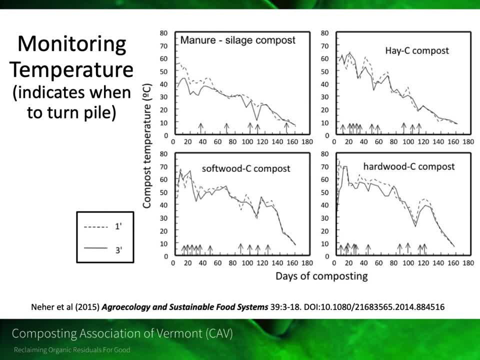 but it's not going to last okay. so just think about how are you building a good fire here? and that, you know, meets these predictions. now we were able to meet the thermophilic requirements for the recipes that we made. true to the cedar iteration moisture, but in the upper left hand. 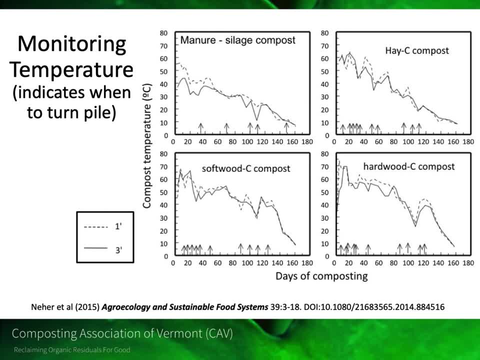 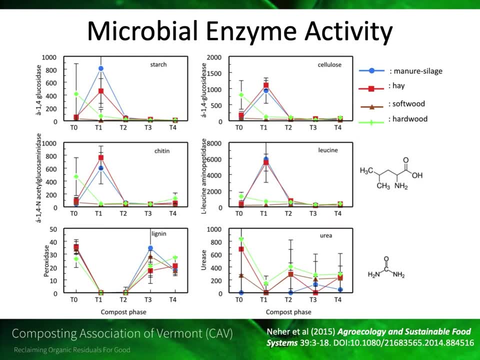 corner our control. it was not to recipe, so we never really reached those temperatures, but we did go ahead and turn it so we can achieve those. so here's an image of the microbial activity that we measured within, within these little bags that we're pulling out at these different times. 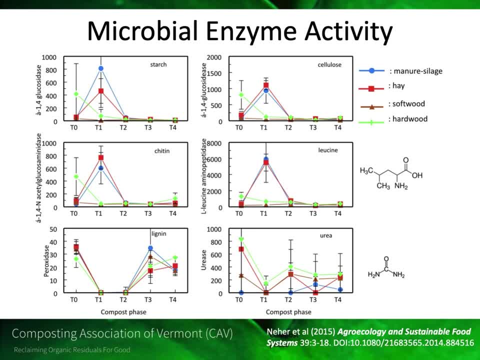 we see t0 to t4 on this slide and the different colors represent the different recipes. microbes produce enzymes outside of their body. their digestion is external, it's outside of their body. so they produce enzymes very specific to different molecules. and, just to keep it simple, we measured some enzymes that were breaking that measured. 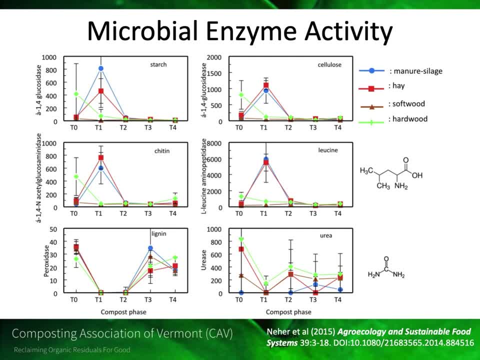 the breakdown of starch, cellulose and chitin, as well as an amino acid called leucine. those are the top four panels and we also have measured an enzyme called- you know would be lignin, which is more like that rooibos tea. the green tea is more like the top bars, but what's really? 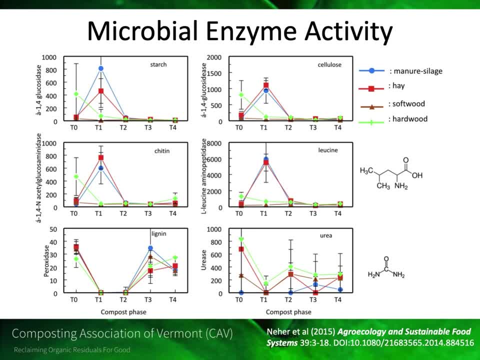 cool about it is it really follows this whole pattern of ecological succession. the first materials to break down are the simple, simpler carbon compounds like starch and cellulose, and so you see those really peaking at t1, and it's lignin that once you get the really easy to decompose carbons first, followed by those that are more resistant to. 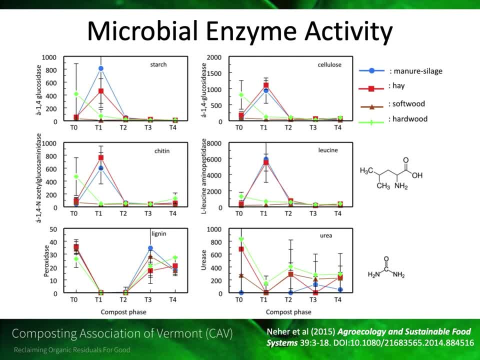 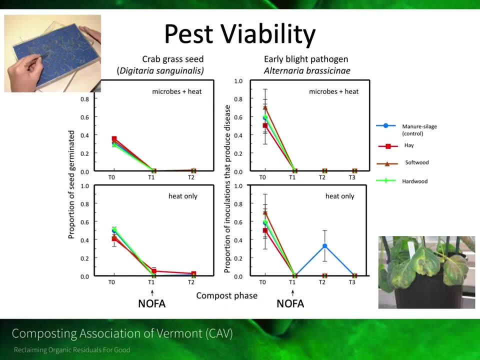 decay and more complex, like lignin. as you can see in the lower left hand panel, the activity of breaking that down came. the peak of that was at t3. so this was just a just a quick test of what's happening in the overall community in terms of kind of ecological succession. so what we really 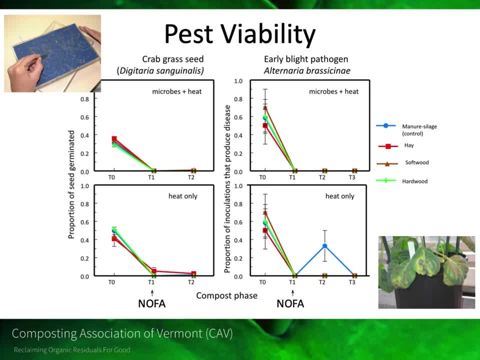 want to see here is test fiability. this is why we conducted this study. so on the left column is crabgrass seed and on the right hand is the early blight pathogen, the alternaria fungus. we measured for the seed. we looked at germination paper where we could put the seeds on there, and look at the 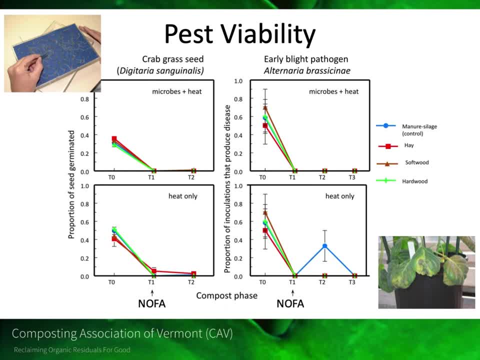 percentage of those that germinated or didn't germinate. if you you're looking for, you know if we had good kill, we don't want germination right for the plant pathogen. we used a bioassay with brussels sprouts. you can see in the lower right hand side. we'd 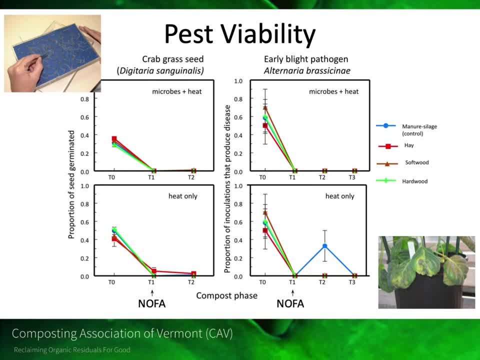 take a q-tip and swab it on there and then put it on the leaf and see if there was a living fungus that caused lesions on those leaves or not. so those were our measures of viability. and then the upper right row is a combination: is the mesh bag the microbes? 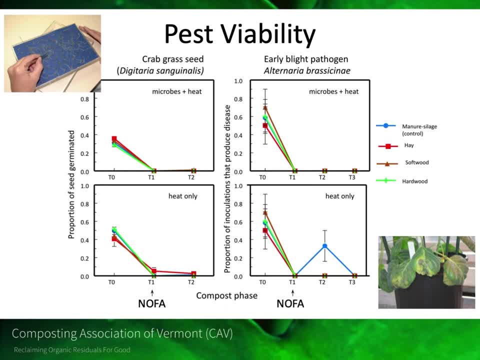 and the bottom row is heat only the solid plastic bags. so it it's a pretty easy story here. it's mostly a matter of time. it's not really the kind of carbon in this case we see for the crabgrass seed. let's just take a quick look, we see. you know that viability or germination rate just tanks. 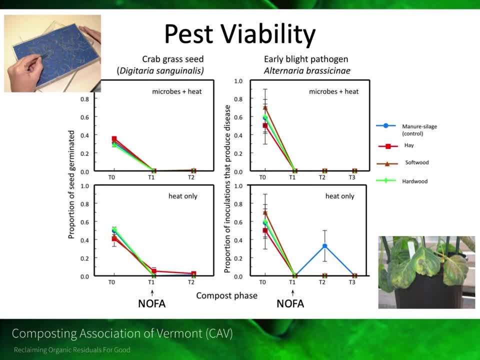 there at t1. so that is the NOFA requirement. so that requirement is: is actually, it's a, it's really working and and killing those weed seeds. now notice, there's it, the uh, the. it goes a little faster when you have microbes and heat than if you only have the heat alone. it's really. 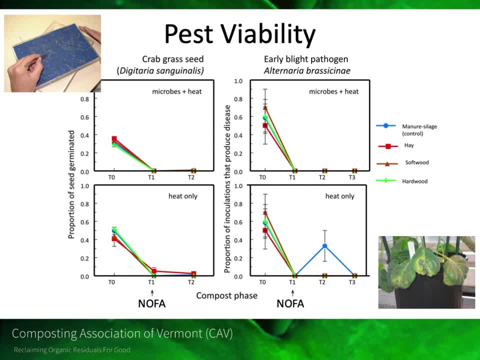 important to have that combination. okay, uh, so you can see, it hits zero in the microbes and heat at t1, where it's not quite a zero, until t2 when it's heat. only on the pathogen. we saw, uh, the plant pathogen. we saw similar results. 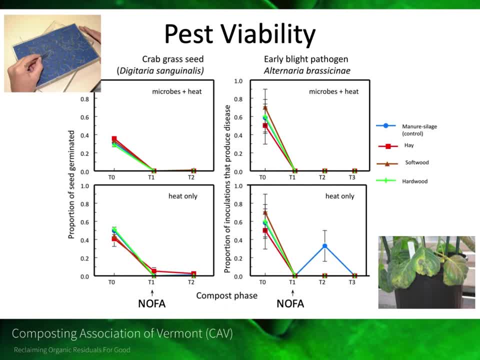 um, really, uh, zero percent viability in all but one treatment, uh, by t1, which is the NOFA recommendations. the one exception we had was for the manure silage, the control there, on the heat only, and we just, you know this is a mean of multiple replicates, so it's a little bit noisy there. but 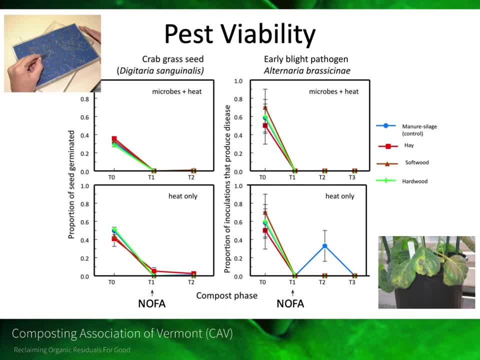 that one was: uh, we saw a little bit of pathogen still surviving at t2, but then it was gone by t3 during that mature composting. so the story with that really is: it will eventually kill the pathogen, it just takes longer. okay, if we'd had it to recipe, it would have gone a lot faster. 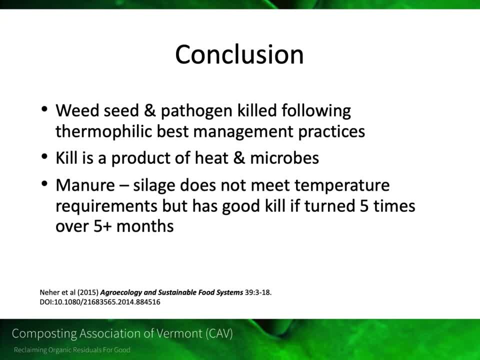 that's kind of a take-home there. so in conclusion, from those experiments we can see that, you know, we do get good weed seed and pathogen kill if we follow these thermophilic best management practices. so composting is a very useful tool to managing pathogens and other pests and helping to close the loop as far as nutrients. 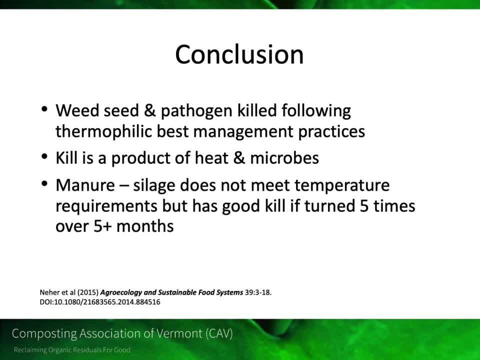 and keeping those on farm. The kill is really a product of both heat and microbes. It's not just heat. Heat is part of the story, but you've got to have the living microbes And that manure silage one didn't quite meet the temperature requirements but it did have good kill, but it just took more. 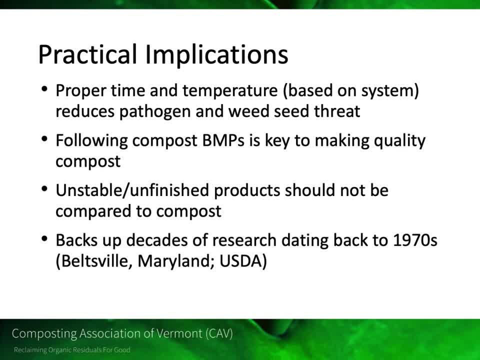 than five months to achieve that. Some of the practical implications of this work is that the proper time and temperature based on your systems helps reduce this threat of pathogens and weed seeds, And following the best management practices is really key in making quality compost, And it's 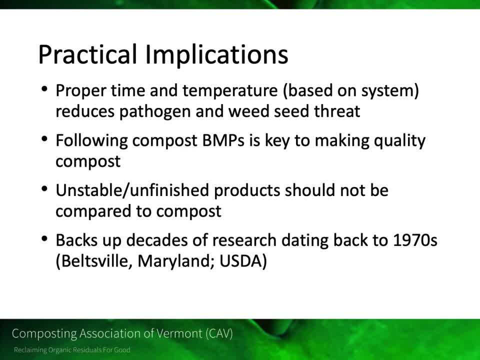 important to have mature compost. They'll be more stable. They're going to contain the suite of microbes that are involved in disease suppression, because those come in. We kill the pest, We kill the pathogens, but the biocontrol agents come later, during the cured, curing and maturing phases. and these experiments help support the decades of research that date back to the 1970s, when USDA and EPA conducted trials in Beltsville, Maryland, that established these thermophilic guidelines to begin with. 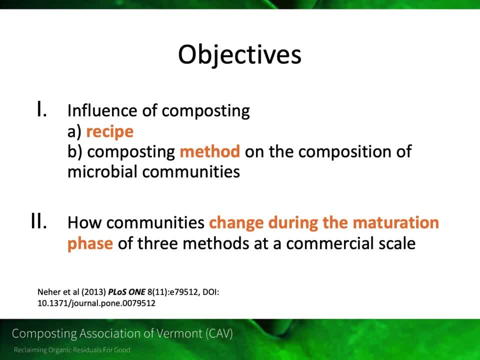 The next phase of my research was then trying to look at the composition of the bacteria. First I looked at the composition of bacteria and fungal communities, For example. if you look at the case of the bacteria, bacteria and fungal communities, they have a lot of fungal impacts on the bacteria. The kind of impact that is there to do with the bacteria. It's too simple to just think about a ratio of fungi to bacteria because you have pathogens, you've got by a control agents, you've got all sorts of different functions within those big kingdoms of organisms. So I wanted to get down to at least genus level of bacteria and fungi. So there were a couple objectives here. One was to look at the effect of recipe on these communities. Secondly, as far as I know, there are a number of different kinds of bacteria that have been active in the community. 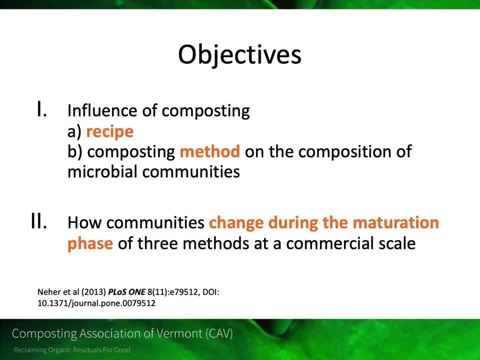 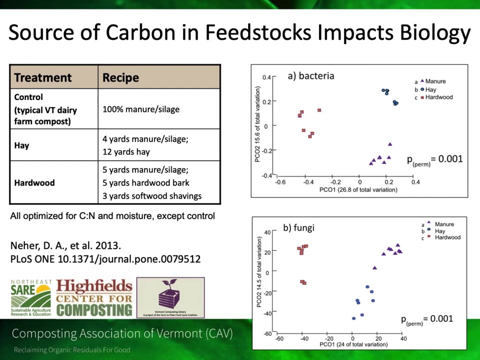 communities. Secondly, to look at the method of composting, and particularly the method of curing and maturation, and then how these communities changed through that maturation phase at these different methods. So source of carbon, it's the same. it's just an extension of the project that. 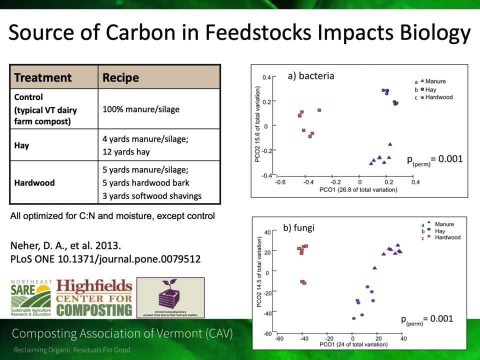 I described previously, where we and we just focused on the control, compared to the hay and the hardwood kind, of the two extremes of carbon and their ability to degrade, simpler, more complex And over on the right-hand side we can see illustrations, kind of cluster diagrams of 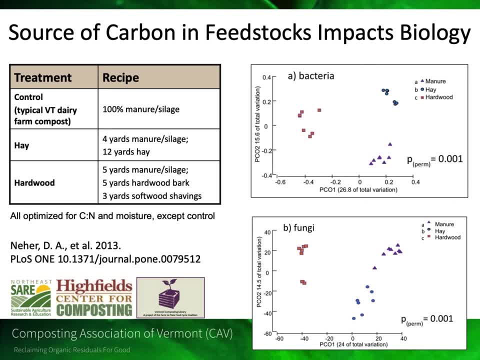 the bacterial and fungal communities. When points are clustered close together, means they're very similar. If they're far apart from each other, means they're different, And the three recipes are coded with different colors and symbols. The take-home message here is: carbon matters. 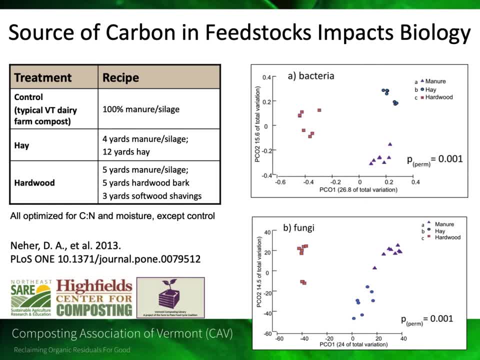 recipe matters. You get completely different bacterial and fungal communities depending on what kind of carbon You put in. So it does make a difference and we should maybe be thinking more about that. The biggest difference is between: hardwood is the most different from the other two. Hay is more like. 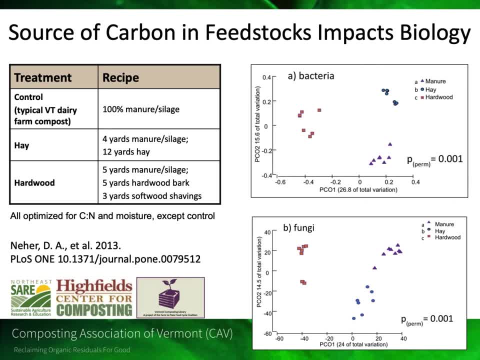 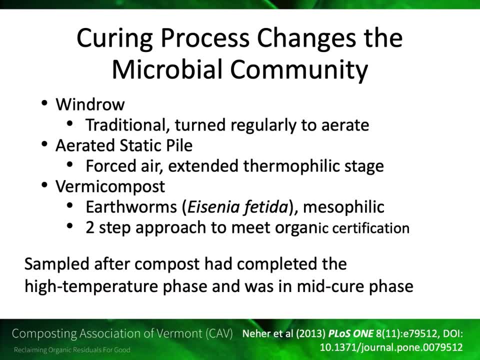 the control that wasn't made to recipe hardwood and that's because there's a bigger separation in the points that you can see there. So bottom line, there recipe matters. So the next one was: take a common recipe, okay, so a common starting point, a common mature compost, and then cure it. 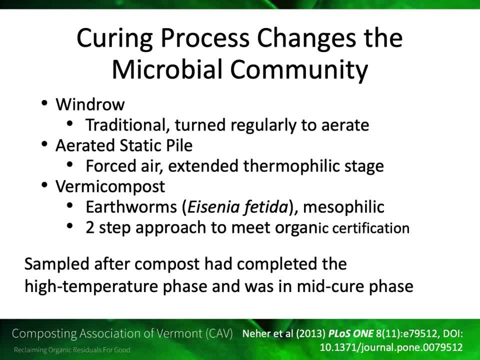 for three processes and then compare what the effect of the curing process is on the microbial community. So we compared windrow, aerated static pile and vermicompost. By the way, I just got to give a shout out to Tom Gilbert because he was involved in all of these studies and very 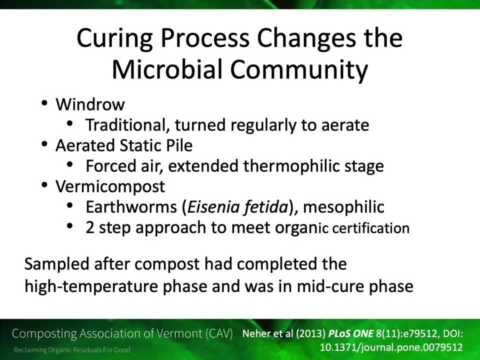 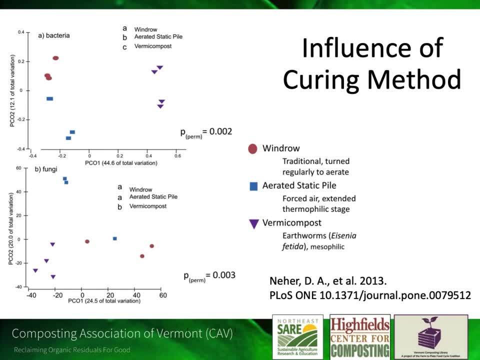 instrumental in helping me deal with the experimental design. So we looked at these three processes and sampled at different phases. Here's the end results of that. The effect of curing method is not the same as the effect of combing the seeders. okay, Same kind of plots that I had in the 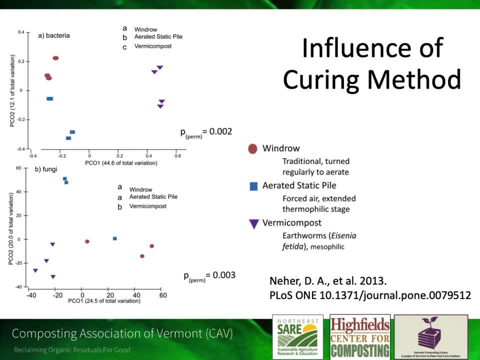 previous slide. The different colored symbols represent the three curing methods: windrow, aerated static pile and vermicompost. Those each clustered into their unique communities, more so for bacteria than the fungi, but, as we can see, in the bacteria the biggest difference. 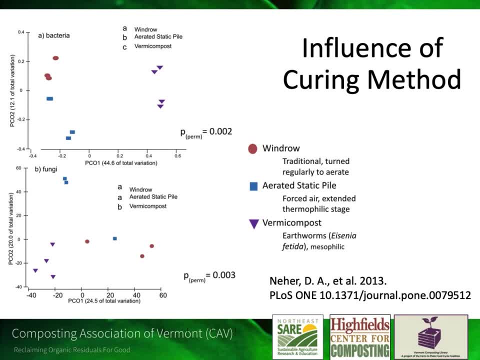 was between this vermicompost and the other two, the windrow and the aerated static pile. So I'll just remind you This- Sorry, I have to hang on. I don't want to be the one who's going to have to talk for an hour. 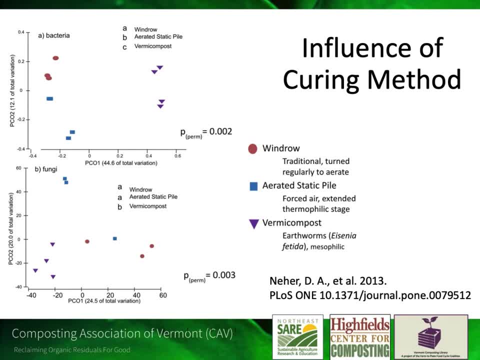 this vermicompost is a two-step process. this is not just throwing material into a little tub and having the earthworms consume it. this went through a thermophilic phase to begin with, and then the curing was in the worm bin. okay, we know curing matters it completely, so they all started with. 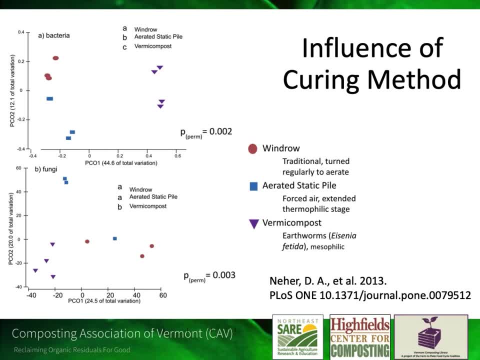 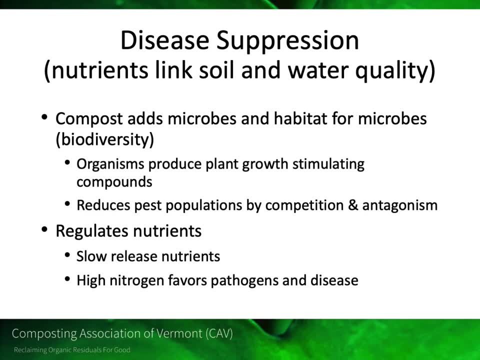 the same community but really diverged depending on the curing method. we know the community differs because of recipe and process. but how does this relate to disease suppression? thermophilic compost will kind of clean the compost of pathogens and weed seeds kind of give it a clean slate. so to 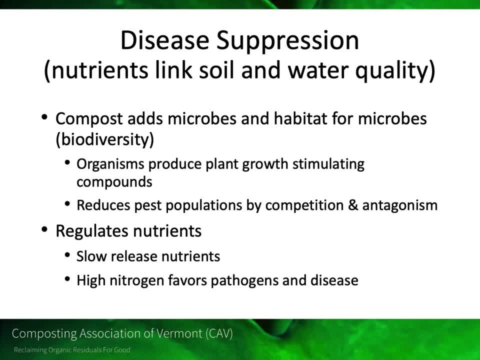 speak, but as the pile goes through a curing, maturing phase, then it allows biological control agents to naturally and successfully colonize those piles. and it's these natural recolonizations of these beneficial organisms that that are the important part of disease suppression. These are organisms that have an ability to 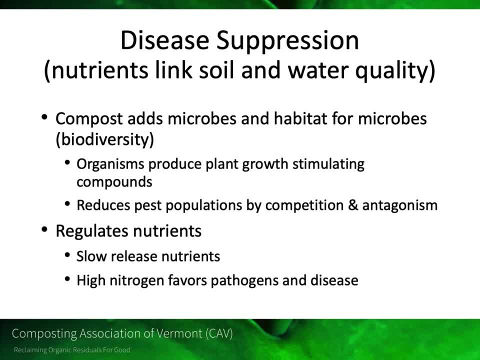 antagonize or compete against pathogens, Or there are also organisms that can help just stimulate plant growth, through by production of hormones, for example. But the idea is trying to learn what microbes are there and then how can we harness those to find the best combination of recipe and 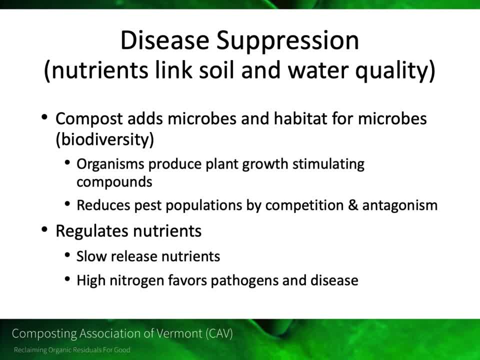 process to suppress disease, And I will also predict that it's very specific to the type of disease you're trying to manage. But I'm going to show you a couple examples. High nitrogen really favors pathogens and disease, And this is another reason we want compost to be part of a slow 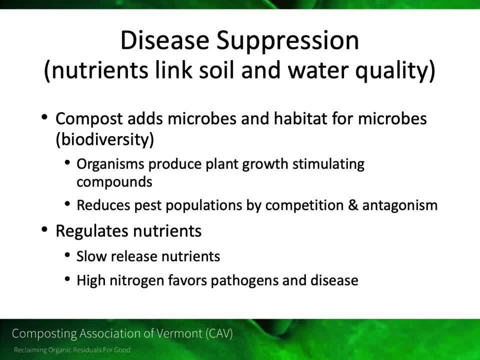 release of those nutrients and matching that with the plant needs, because that's going to help tip the balance in favor of the biocontrol agent over and above the pathogen. So here's some work that was done in the past. I'm going to show you a couple of examples. So I'm going to show you a 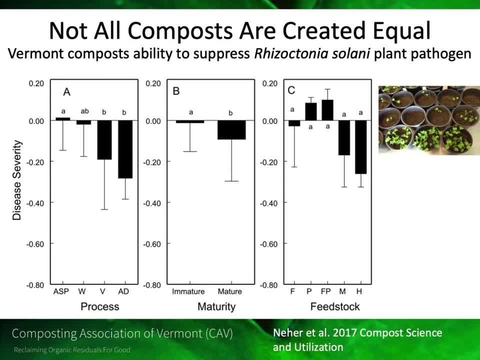 few examples. So this is done by Lynn Fang for her master's thesis at University of Vermont And she collected- I believe it was 14 or 15 different commercial compost from around the state of Vermont And we were looking at their relative ability to suppress a fungus that causes soil-borne. 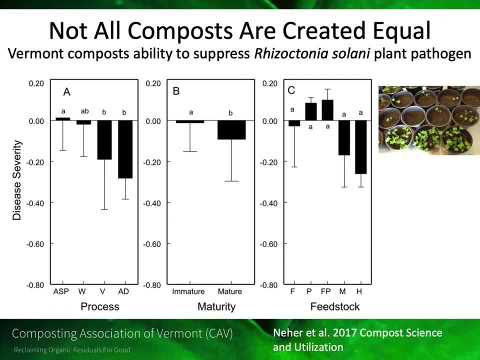 path. It's a soil-borne fungus called Rhizoctonia solani. It's a really tough pathogen to manage And it's a major problem for lettuce growers here in the state. It causes bottom rot on lettuce, So that's how we got started on that. 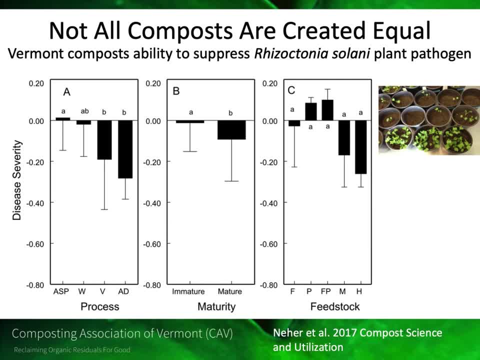 But we created a bioassay over on the upper- in the little image there you can see using radish seedlings. We could take the material and then plant 25 radish seeds in there and then look at percent germination as well as pre-emergence and post-emergence damping off caused by this. 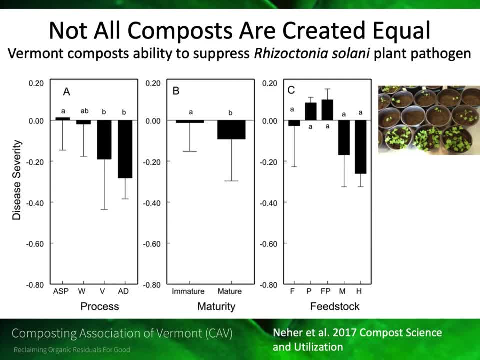 pathogen. In this graph or in these panels you can see we compared process, four different processes, two maturity levels and then five different feedstocks. The way we interpret these graphs is the zero line is would just mean that let's see, it's kind of. 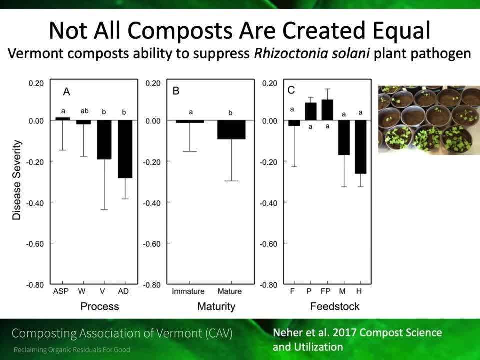 comparing it to a control. If it's above the line means it's conducive to disease. If it's below the line means it's suppressing the disease, reducing the disease, compared to a control. If we look at process, we can see that the vermicompost curing method had the great, great, great, great great. 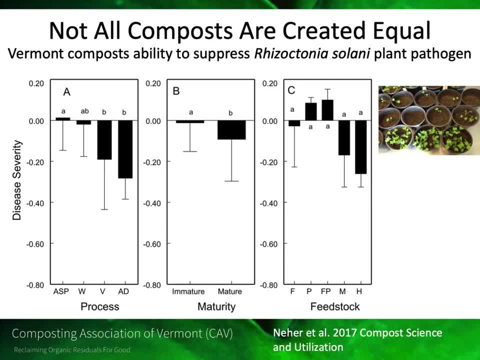 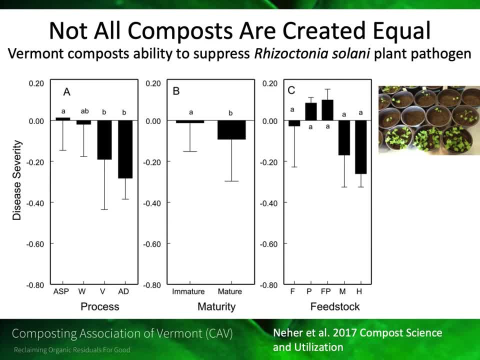 suppressive, but that's not the focus of today. In the maturity we saw greater disease suppression with the mature compared to the immature compost products. And on the right-hand side we have food. waste is the F. P is poultry-based manure, and then we have FP, which is a mixture. 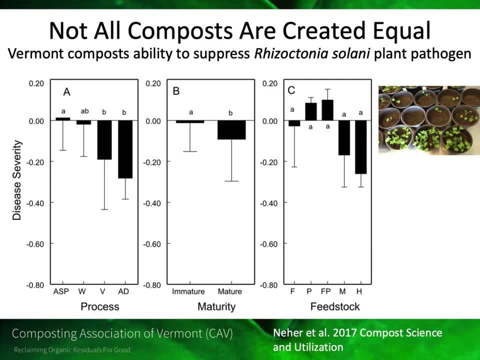 a food waste and poultry M is manure and H is hardwood. We saw the greatest disease suppression with the manure and hardwood And we actually saw those that contained some of the poultry manure to actually be conducive to disease. So bottom line here really is: no two composts are alike. 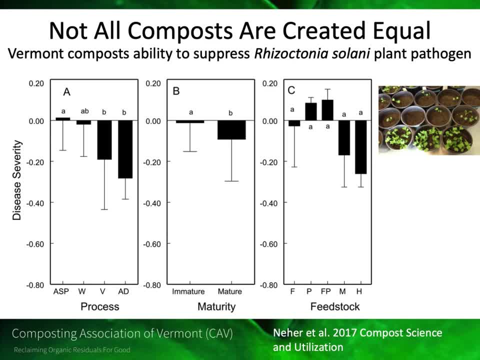 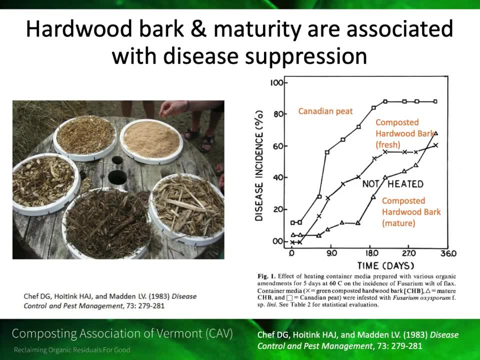 They're all unique And that we also learned more disease suppression with vermicompost, hardwood bark and mature. I wanted to say that these results really support earlier work that was done in the 1980s by Harry Hoyntick and colleagues at Ohio State, And I'm just going to show a couple slides from his work. 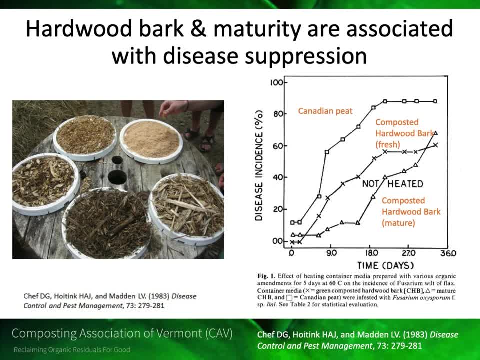 This is one where he looked at the different compost recipes and maturities for a disease called Fusarium, wilt of flax. Fusarium is another soil-borne pathogen Harry did a lot of work on from the Load-in Life for Horticulture Products and, you know, night for the horticulture industry. 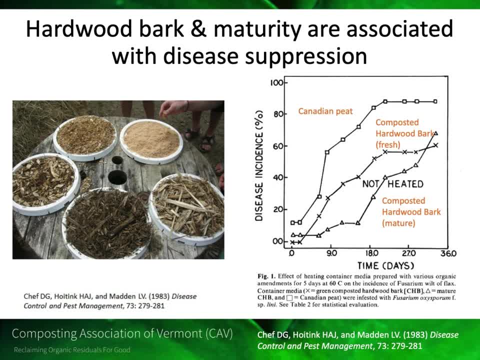 and they traditionally used Canadian peat moss as a soil-less mix and were running into major disease problems. So that's the highest in disease incidence in that in that graph there is with the Canadian peat. But if they made a compost containing hardwood bark and grew the plants in there, they saw a reduction. 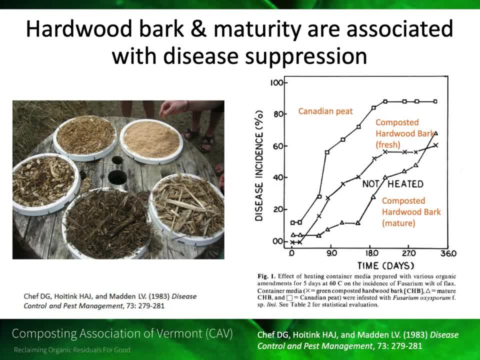 in the amount of disease, John Kroeks 홀 are a little bit lower And the difference between those two lines is the higher one is with fresh or immature material and the lower one is with a mature compost. So the least amount of disease. 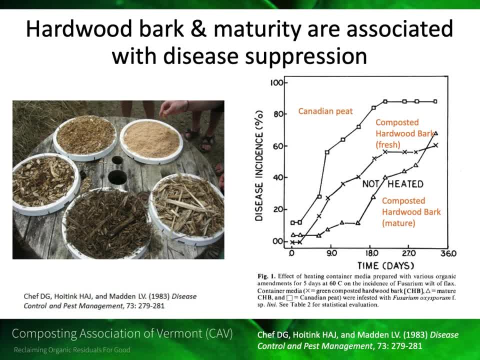 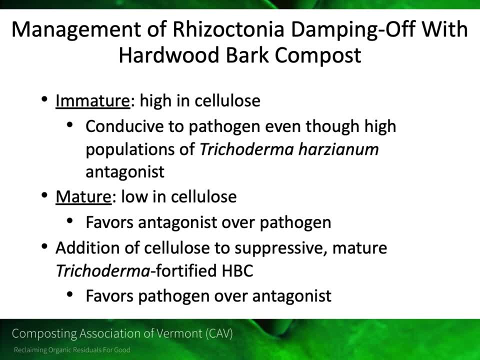 with a recipe containing hardwood bark and mature. This is kind of a summary of a pretty extensive set of experiments that his group did, trying to understand the mechanisms of what's happening with hardwood bark and maturity, And these are from looking at the Rhizoctonia that I mentioned. 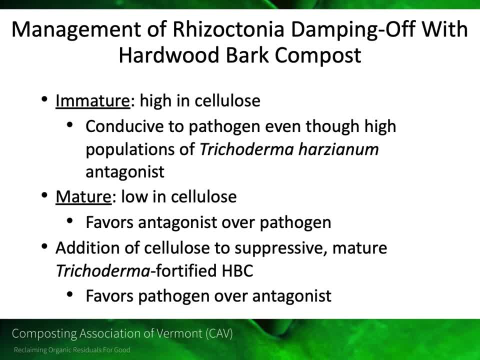 from our earlier bioassay And their conclusions were that we're looking at the maturity and the hardwood bark in. there is really affecting the relative competition between the biocontrol agent and the pathogen, And the immature tends to be relatively high in cellulose. It's those readily 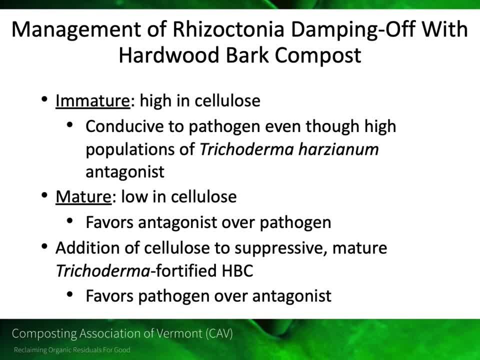 decomposed material, And the immature tends to be relatively high in cellulose, And so it's a lovely beginning to start these experiments, And I think we're hoping that we end up with a good end to that. JEFF SHAMROCK. 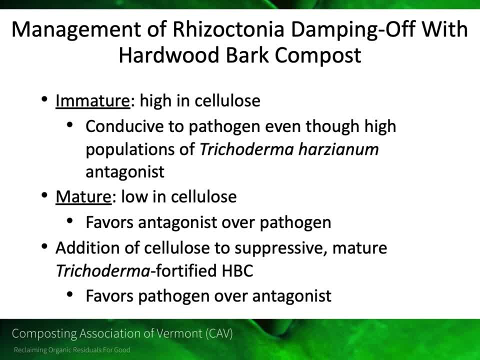 That's brilliant, And I think part of what those scientists are working on is perfect boots, Because this is where it's quite hard to keep track Brock failure to show JEFF SHAMROCK. sure, Schmidt, you want to startie? 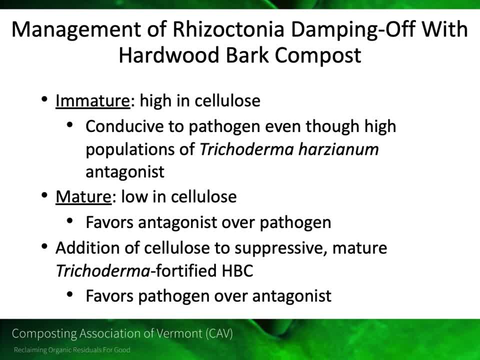 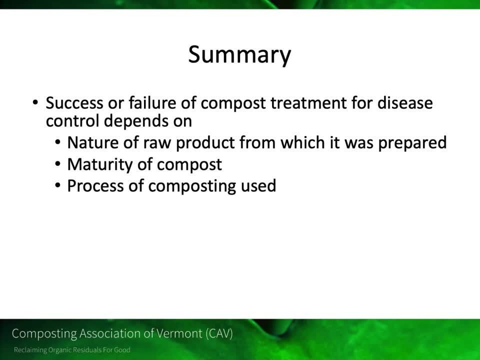 agonist, the biocontrol over the pathogen, and so that's the mechanism that Harry's group was posing. so, and they're finding that this works well for like pythiums and phytophthoras as well. So, in summary, the success or failure of compost treatments for disease control depends. 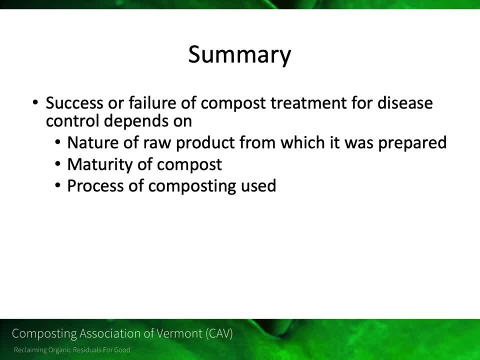 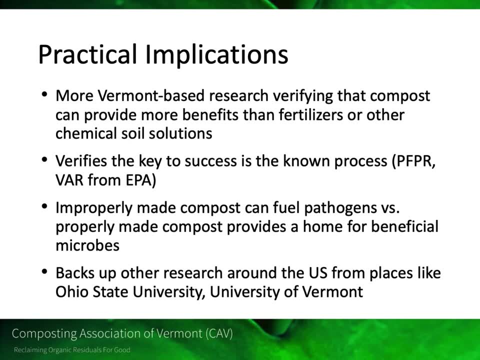 on the nature of the raw product, the maturity and the process of composting. Practical implications are that more Vermont-based research is verifying that the compost can provide more benefits than fertilizers, and it's verifying the success that we know from some of these thermophilic processes. 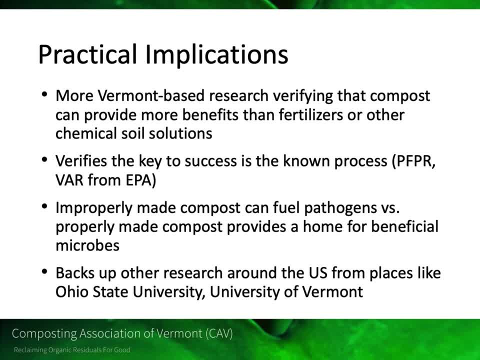 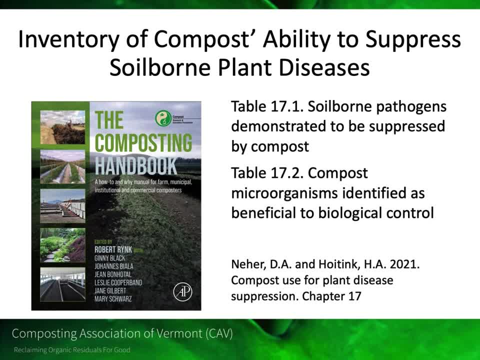 in the long-term in the making by Robert Rink the new composting handbook, So I have a chapter in there and I just wanted to point out that we have two very extensive tables on the use of compost for managing soil-borne pathogens, which microorganisms and compost are identified to be. 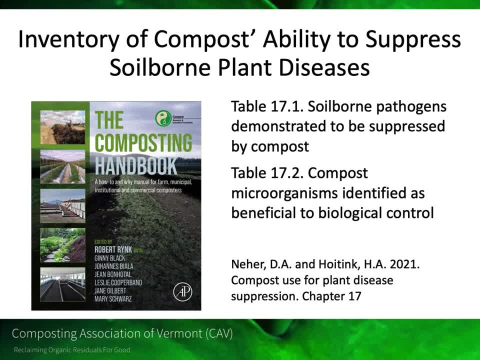 beneficial to biological control. So that book's going to come in print as well as digital. I think it's running about $99. a copy is what I saw advertised, but I think it's about 400 pages. It's going to be quite the book. And then another resource we have if you want to learn more about. 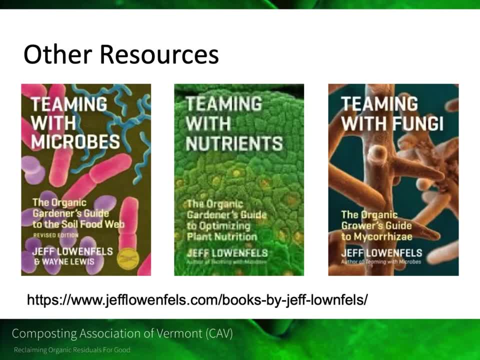 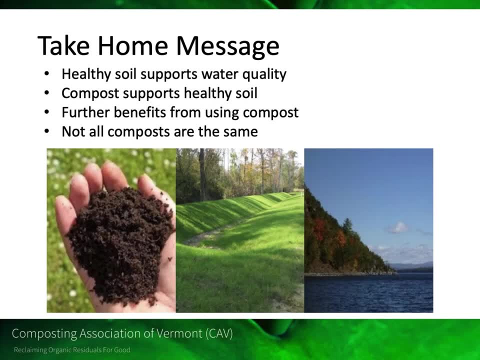 the microbes, or these suite of books by Jeff Lowenfels- just a shout out to him. We'll put all these resources on the CAF webpage. So the take-home messages here. big picture is: healthy soil supports water quality. The compost supports healthy soil and there's additional benefits like 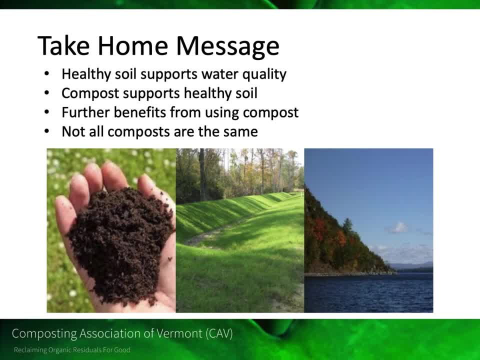 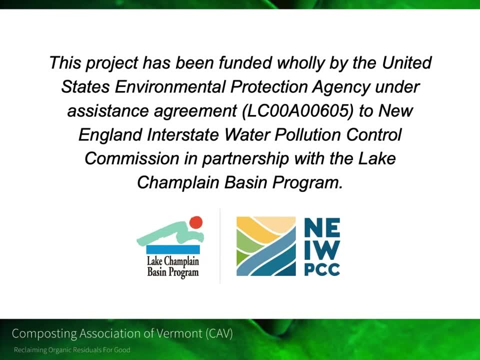 disease suppression. that can come from using compost, and not all composts are the same. I think we're going to have to look for a future of designer compost. Thank you so much, Deb, And I'm just going to give one more thank you to our funders. 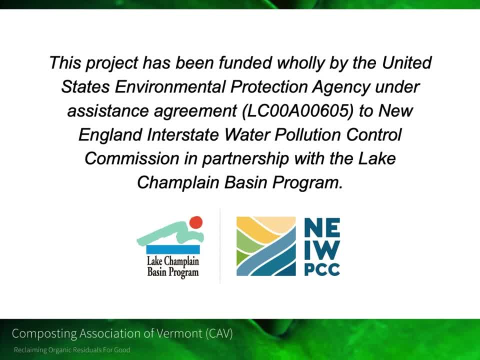 Lake Champlain Basin Program and the New England Interstate Water Pollution Control Commission for supporting this webinar and the entire Soil Builders webinar package. We do have 10 or 15 minutes for time for questions and some did come in And I'm actually going to. I think we have. 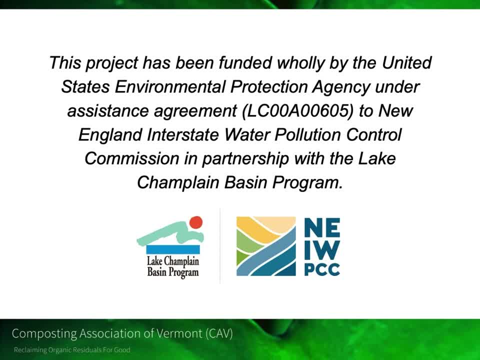 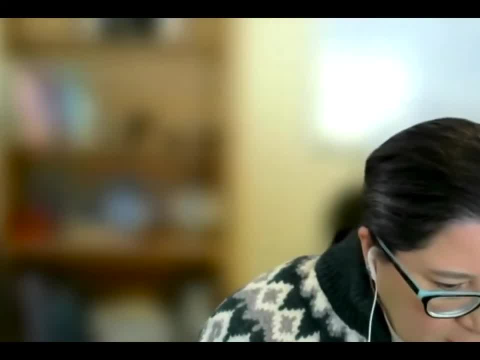 time to get through all of them. I'm going to go through all of them. I'm going to go through all of them. So I'm going to go actually in backwards order, Deb, because the later ones, of course, refer to your reference, your research, more So one thing came in was 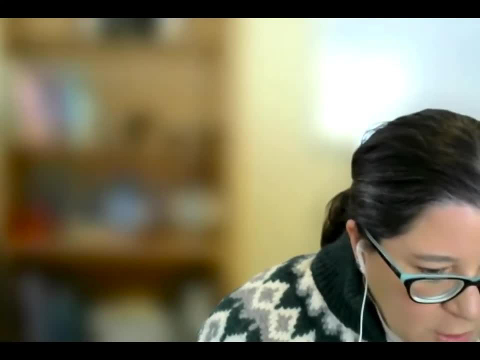 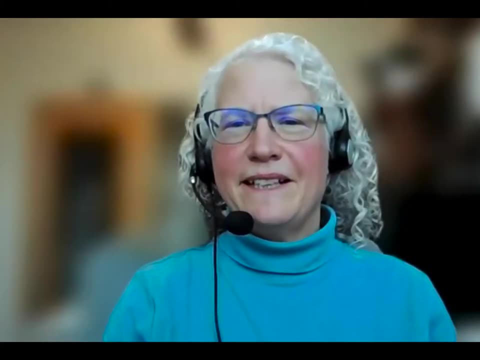 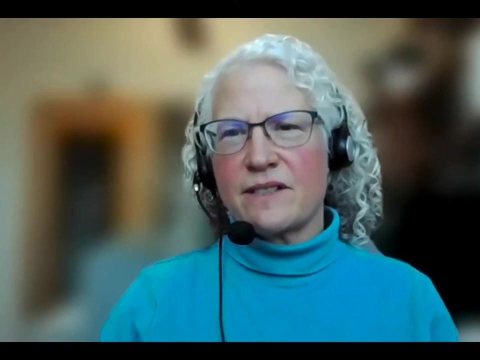 Sarah says my seven-year-old wants to know what happens if there are too many mushrooms in a compost pile. I don't think that's a problem And the fact is, when your mushrooms- those are Basidio mycota which represent- and tell you it's a late stage of succession. So that's going to tell me that you're going to have to do a lot of research And I'm going to go through all of them. So one thing came in was Sarah says my seven-year-old wants to know what happens if there are too many mushrooms in a compost pile. I don't think that's a problem And the fact is. 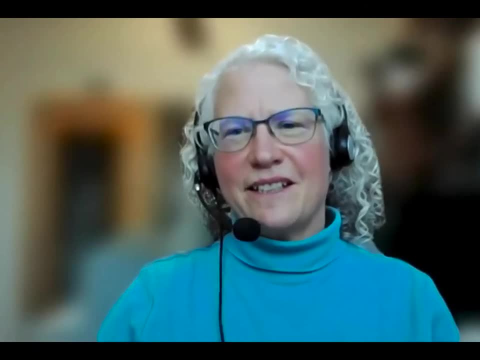 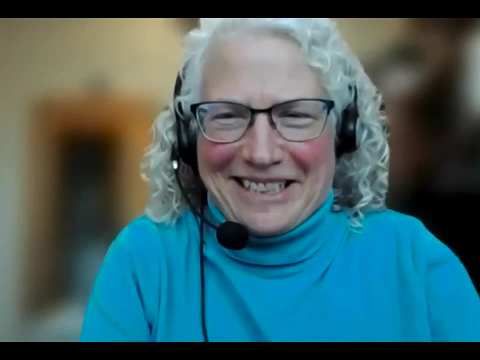 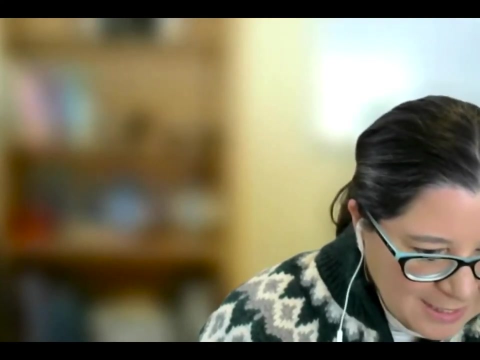 probably decomposing the lignans, And so I would actually think that's probably. that's fine. I can't imagine you'd have too many mushrooms would be a problem. Good question, though. I love it, Thank you. Megan says the UVM Soil Lab does not perform aggregate stability tests. Are there? 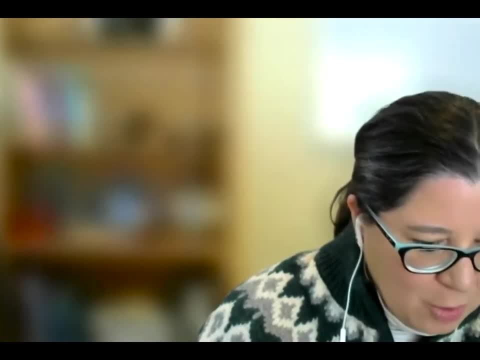 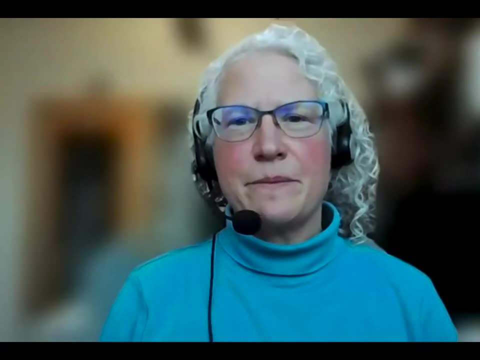 recommendations on where to have tests done or how to incorporate this into nutrient management. That's a great question And it's something that's on our mind because it's super important. I know Josh Faulkner who is managing that lab right now. 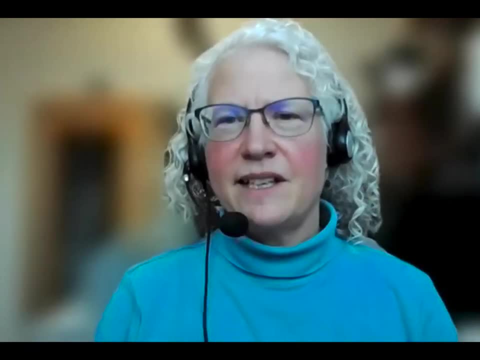 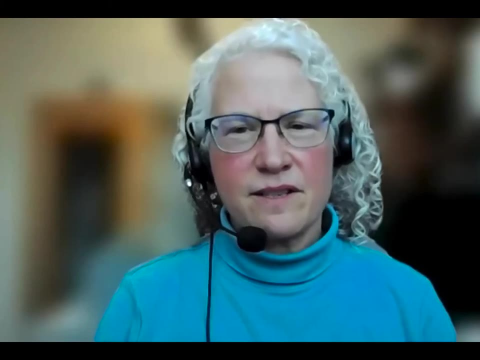 and I've talked and that's high on our priority list. Once we can, we're trying to find resources that we could add that as a metric. We just don't have it yet, but we're in those conversations. We do. I'll just mention that UVM- this is our first. well, it's be starting in the second year. 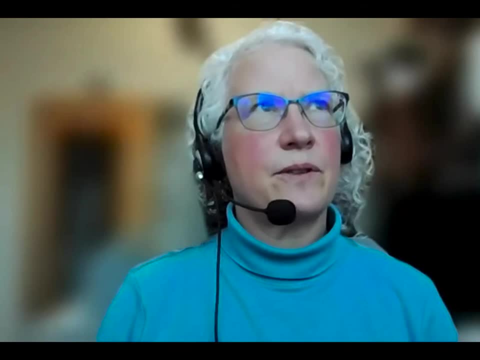 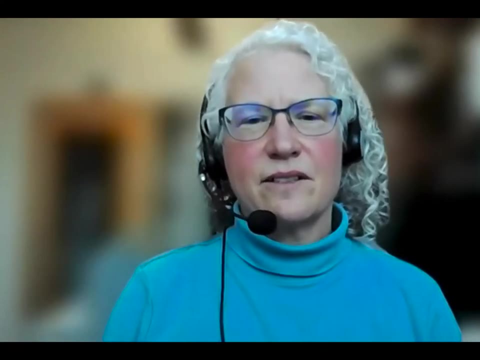 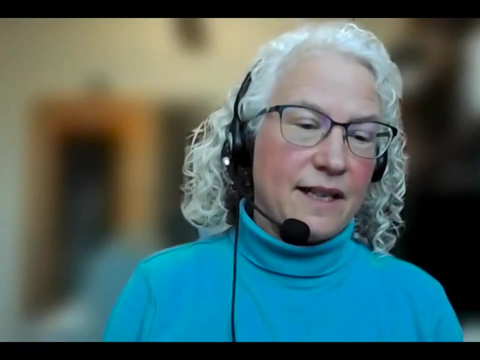 of a new center that's a partnership with USDA ARS, the Ag Research Service called the Food Systems Center, And Joshua Faulkner and I were. I was leading the soil health component of that group so- and Heather Darby was also on that group and I think we had a group of about 10.. So 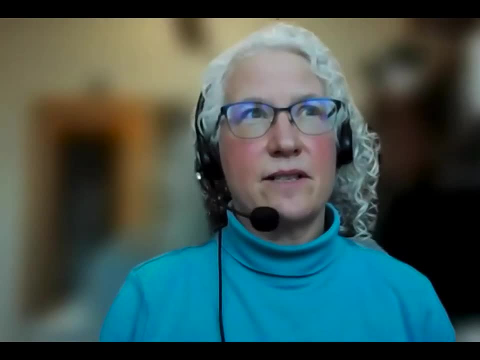 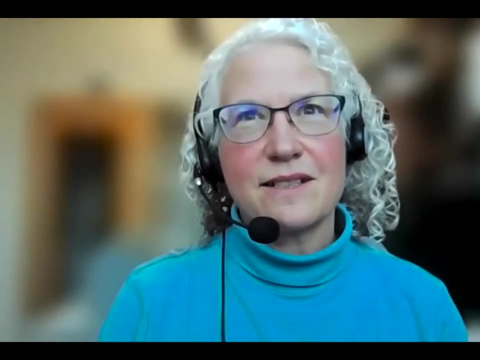 I honestly don't know of a commercial lab that does it right now. We've only been able to do it mostly at a research level. We do have the equipment, It's just so. I don't have a good answer, but I think 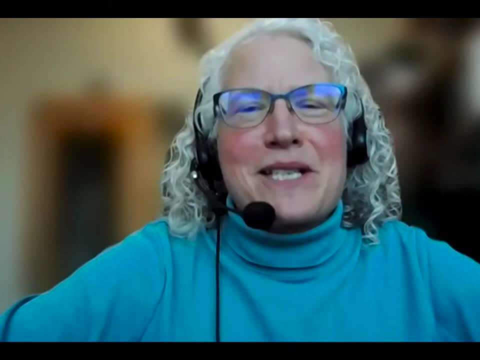 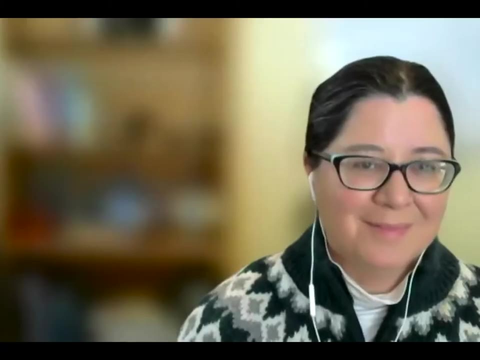 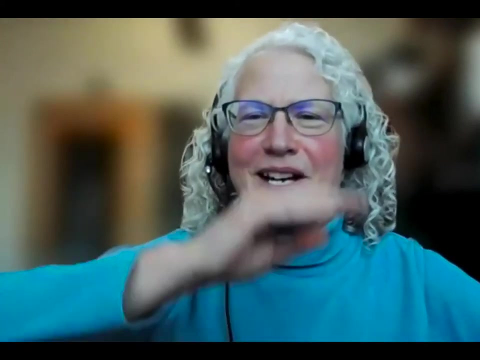 think if anybody tells me if they need to add a metric, i would say: do that one. it's just laborious, it takes time, it's not hard, it just takes time. um right, thank you. it's like doing a thousand of those little slate tests, in a way, except you're dunking all these different sieves and measuring. 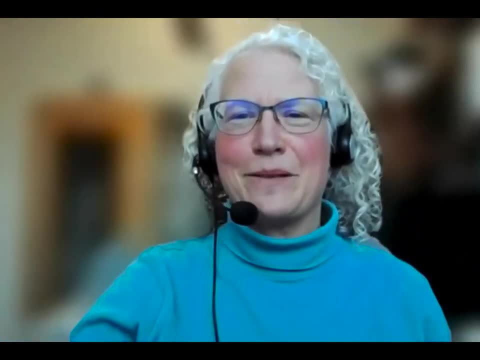 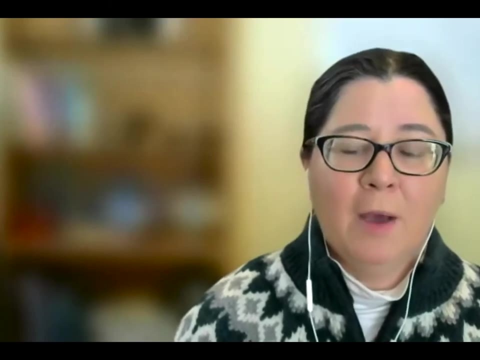 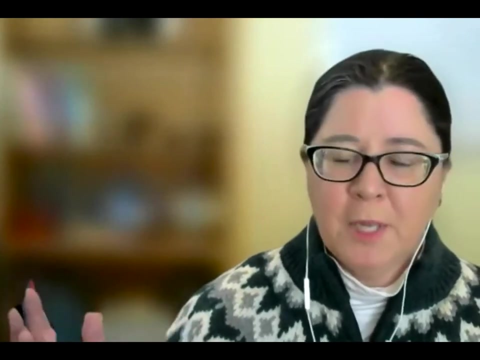 how they fall through different sizes of sieves and weighing them. at all that level you can do some of the other tests just to get at least a qualitative idea of how your soil aggregate is. and so, depending on you know if you're looking for something that would take multiple samples to. 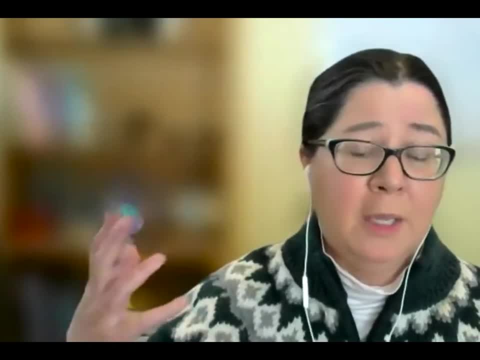 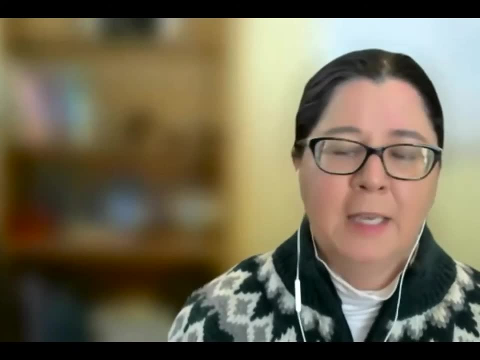 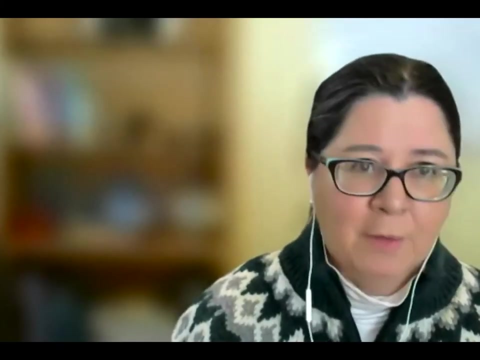 get an idea of different areas of a field or if it's smaller scale, like in a garden, um, there's some really neat opportunities that i there's a ton of youtube videos about how to do slate tests and and and other things, so that's something to just think about. um depending on on um the scale. 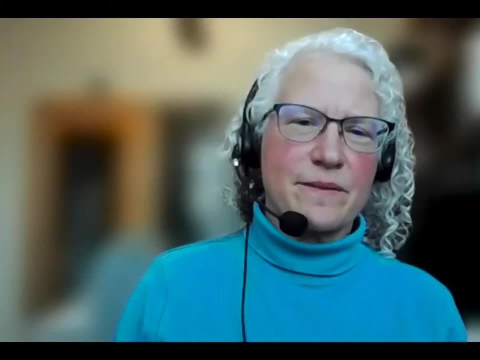 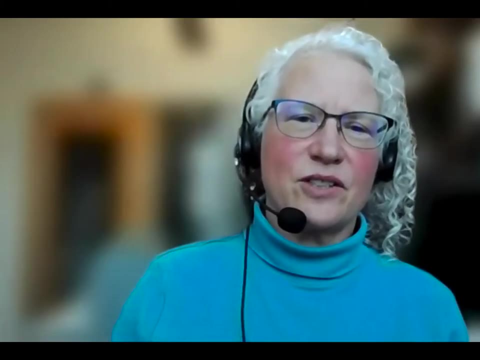 of course, of what you're doing. i see, uh, lynn fang popped up and said cornell does them. oh great, i don't know what the cost is, but i would guess it would be a sizable chunk. but if you just need an idea you could try. 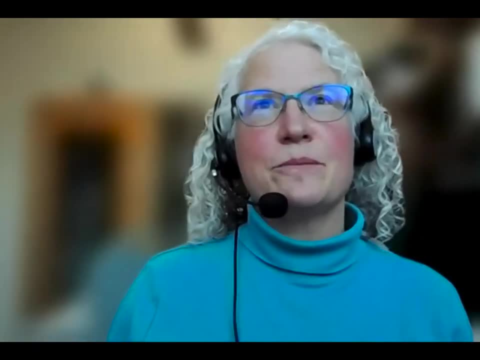 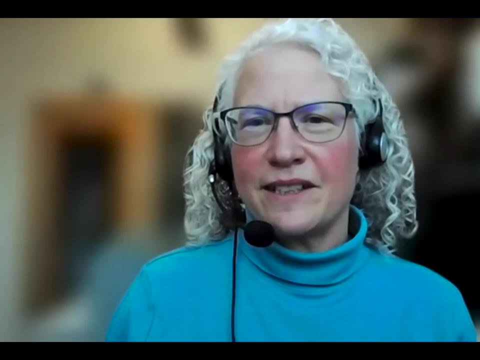 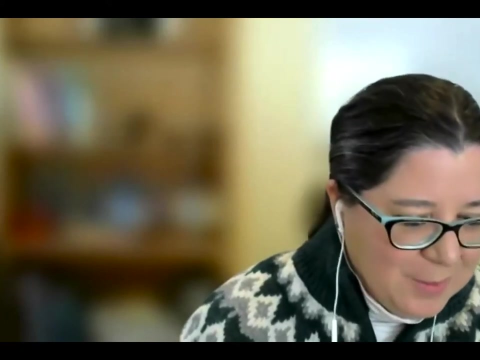 yeah, she says it's expensive. i'm not surprised, just because it is laborious, um, but you could try that, designing your own little slate test or, as i mentioned, with the egg carton, and you're going to be able to. you can do relative comparisons. yep, and those are easy. yep, okay, um, a question. is. does thermophilic composting also kill bromus tectorium or polygonum species, japanese knotweed? hmm, i have not tested them specifically but uh, based on my choice of the giant crab gas, if it can crab grass seed, if it can kill those, i would uh predict that it could. 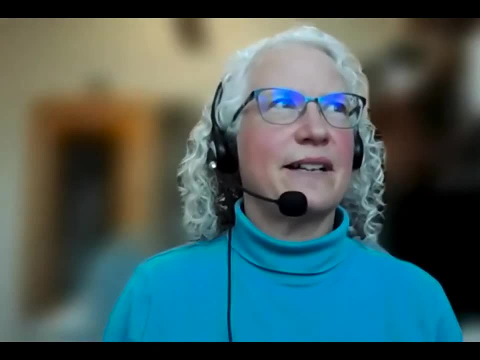 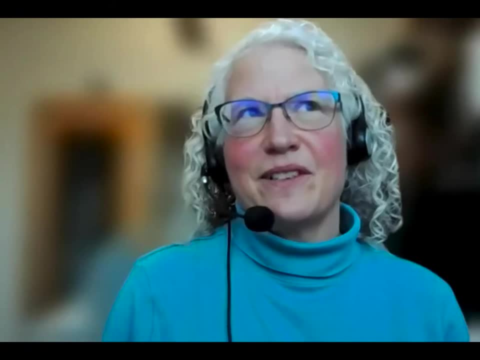 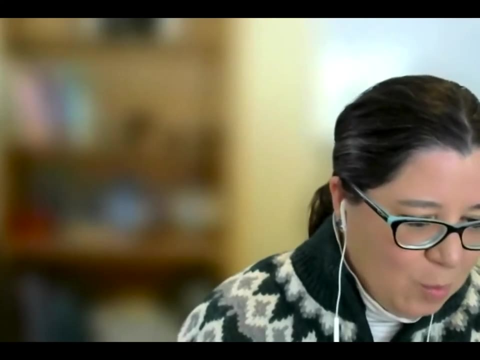 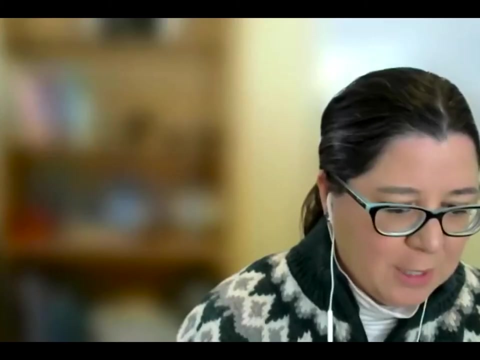 that was part of why we chose the seed we did because it would be, you know, kind of the most difficult we could think of. great thank you. um. were the compost piles covered or allowed to be subjected to different rainfalls during your trial? um, that seems like it would be a large. 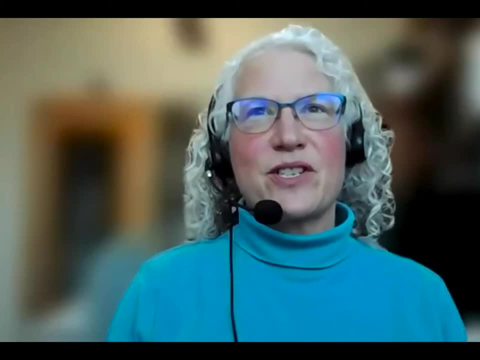 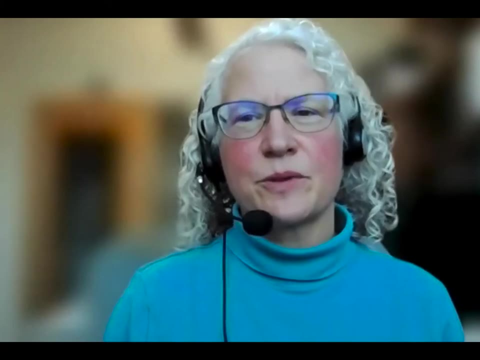 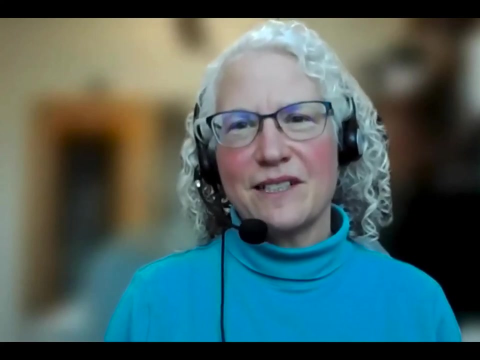 variable potentially? yeah, that is a good question. um, our in our system, to my knowledge, they were not covered. they were open, so, but you do have to really monitor the moisture. that's really important. you don't, if you're going to get a lot, it's going to be exposed to a lot of rainfall. then we need to think about doing some. 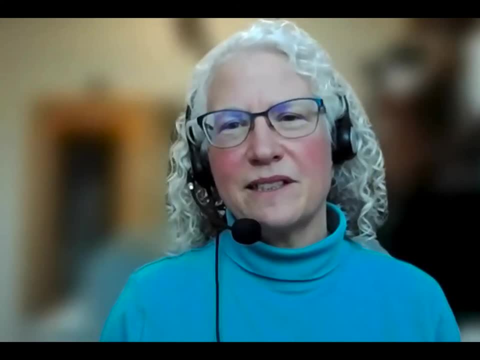 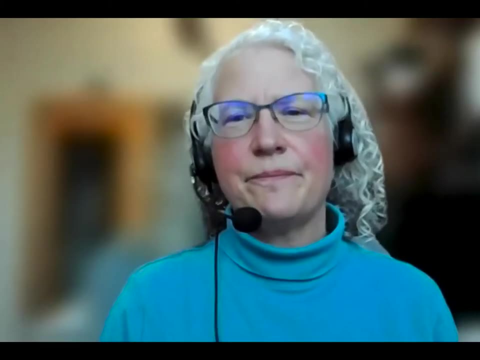 covering. but in my particular prod experiments they were open. yeah and deb correct me if i'm wrong- but they were all basically in the same field and so exactly side by side, not like they. one was getting a ton of rain and another one was getting no rain, so at least it was. 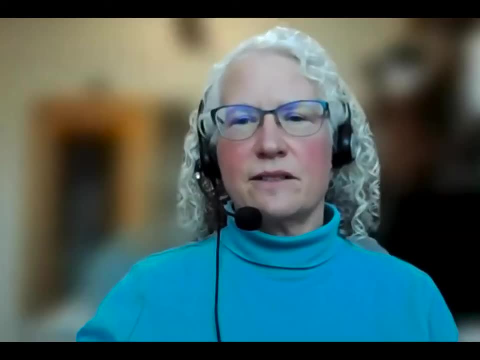 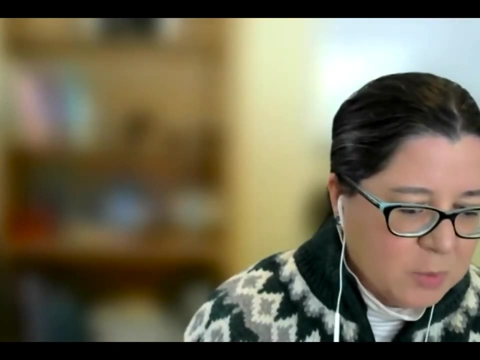 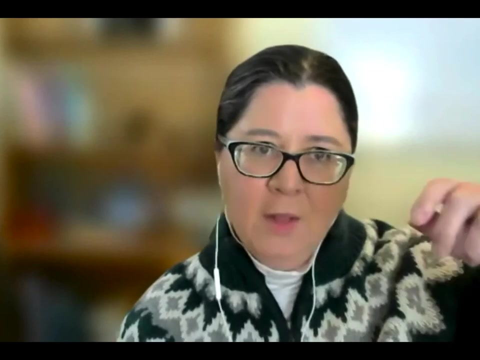 controlled more or less for that. yeah, they were all within an acre space. yeah, great. um, one person said that they didn't realize that the those little triangle tea bags were not compostable and hopefully they're removed after the fact, and i think that is actually specifically in the directions and the whole idea of that citizen science project. 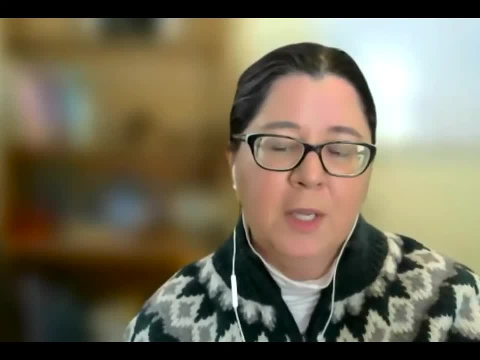 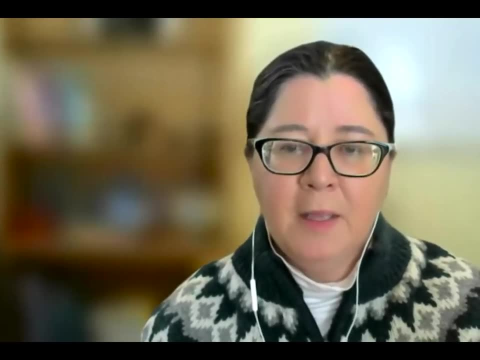 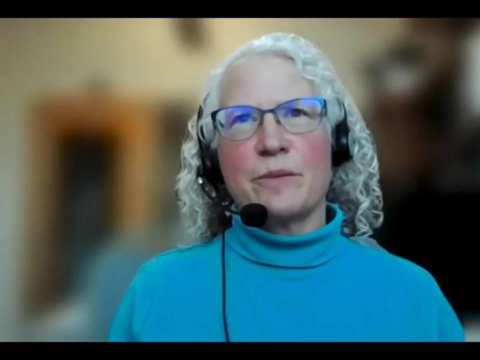 is to remove them to measure the decomposition, and so, um, there's not, uh, you know, direct supervision of everybody participating in that study, but it's, you know, clearly the intention of that. um, it takes removal to actually get your measurement, to send it in, because you got to bring it in and weigh it. 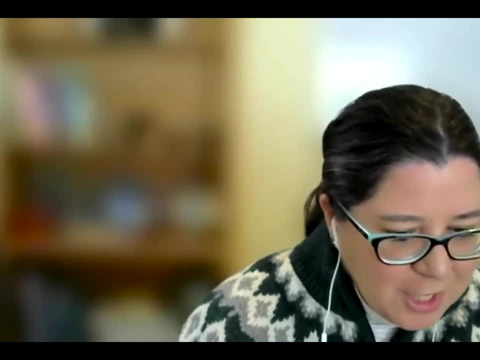 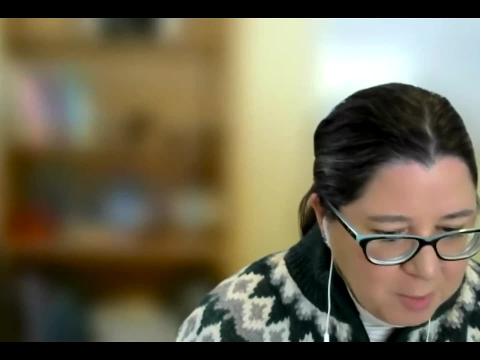 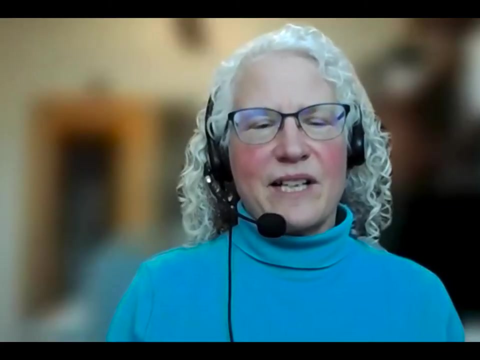 yeah, yeah, um, with climate change, are we getting too much water? this person says their compost pile has been saturated. is there any way to prevent this? should they be covering it with drop cloths? that's a little bit more general of a question. do you want to? well, i would if you're. 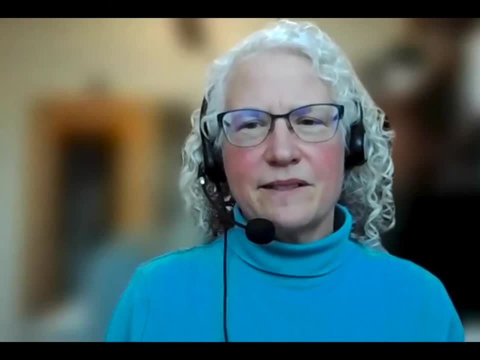 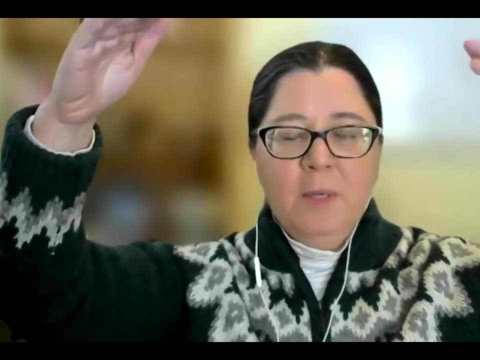 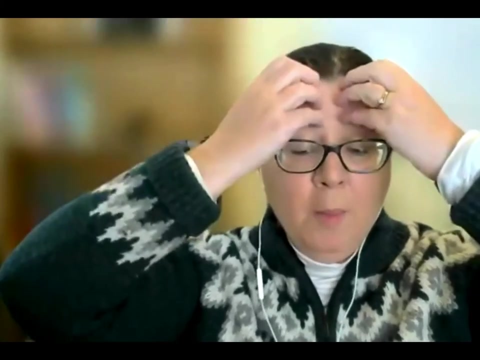 at a risk of getting too wet, then i think you do have to start thinking about some kind of coverage. yeah, yeah, it could be a tarp, depending on where you are. i've also seen people um like put up like the, just like the shelter, like a roof with a pitch where the water will run off. um one person i worked. with. actually, we ended up moving their compost pile, because it was just where all the water from a pitched roof was running on to their manure-based compost pile. um, which was it was creating a big mess. so, yeah, you don't want a lot of leachate, i mean a proper moisture, but you want to, so you. 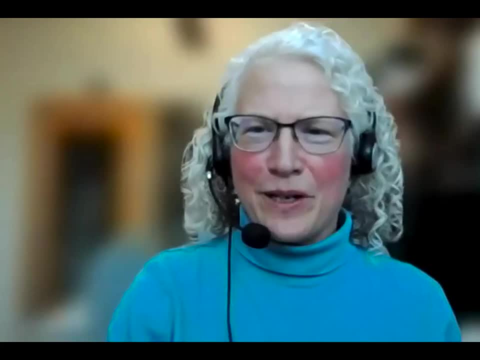 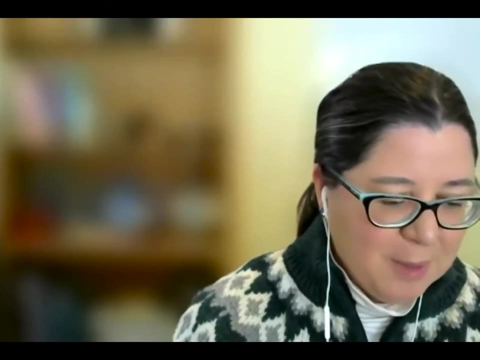 could squeeze it in, and then you could squeeze it in, and then you could squeeze it in, and then you could squeeze it and see it glistening between your knuckles. but you don't want water, free water running off of your pile. yep, exactly, um, okay, and this one is referring to a figure and i can bring. 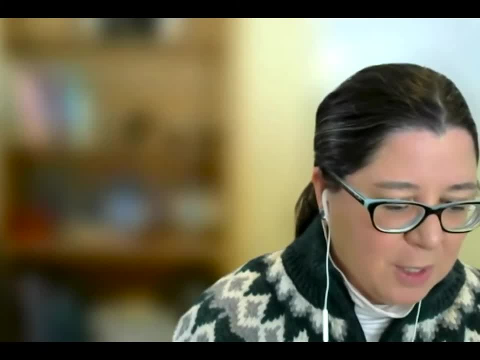 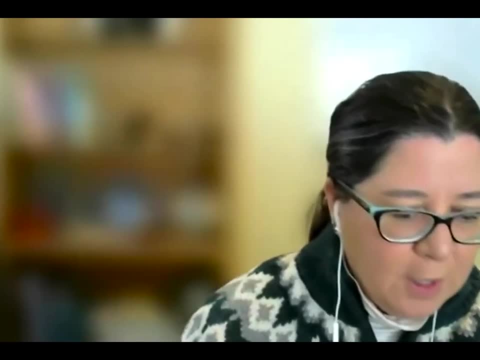 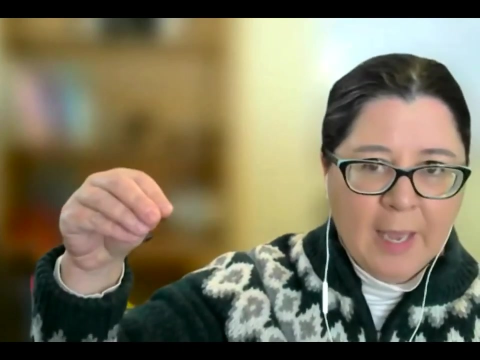 it up if you need it? um deb but, but we could also maybe just talk about it. so let me know um figure one on the water holding, carbon and bulk density graph. um the water holding did not keep increasing with when, even though more compost was being applied. can you talk about? 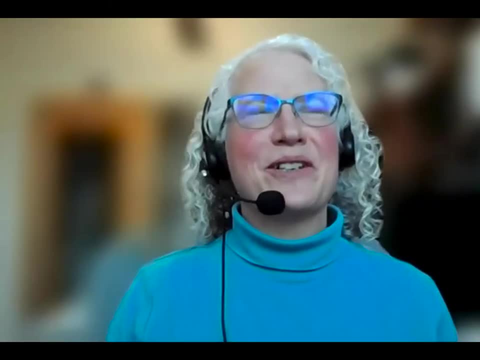 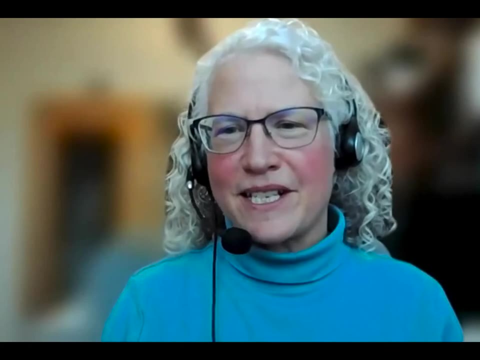 what was happening with the water holding did not keep increasing with when, even though more compost was happening with that. yeah, i, i did notice that when we were doing the slides. i i can't really explain it other than say this is a mixture of like 13 different studies and i think 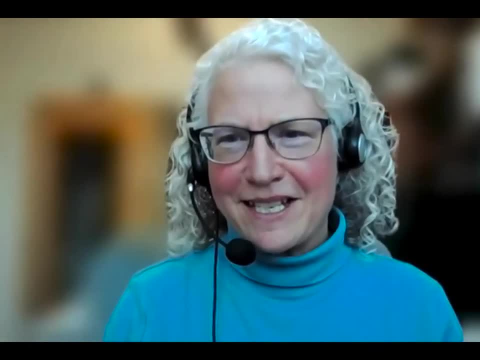 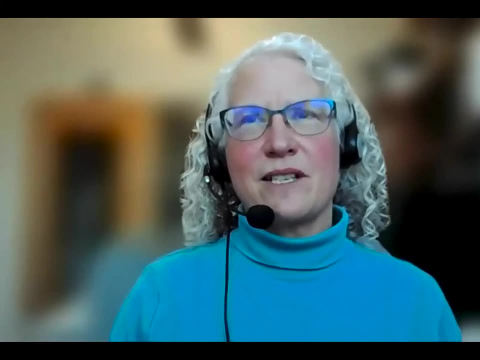 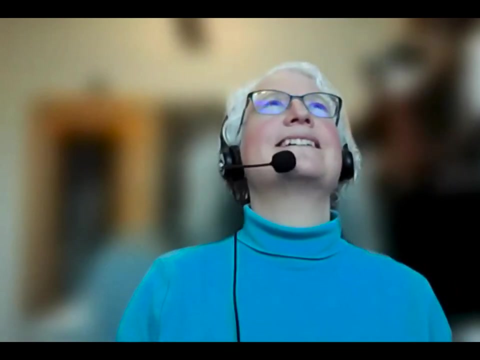 it's just an artifact of that. combining those studies, i mean theoretically, you would see that increasing, but i you know. another thing to keep in mind is these soils have different soil textures, like percent of sand clay and and sand clay and silt, and that's something you can't really change. you can change the carbon in there and that's the. 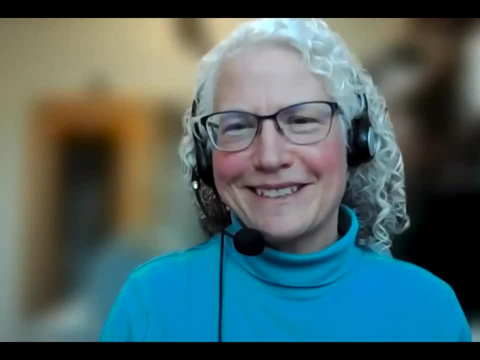 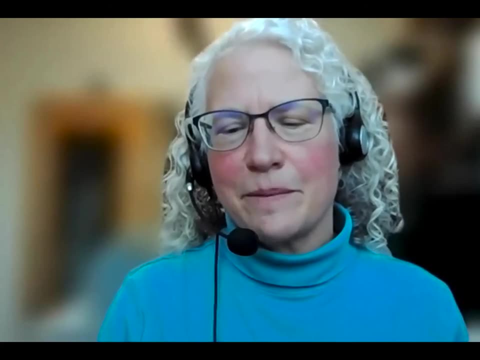 part, that's the water holding capacity, really the part that you can change. but i think, yeah, i mean it is a little disconcerting to see it, but i think it's just an artifact of this really representing a mixture of different kinds of uh systems in different geographies. great, thank you so much um. 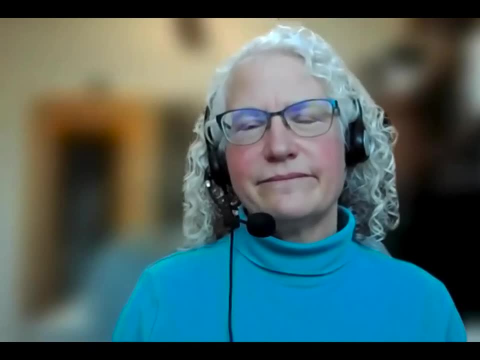 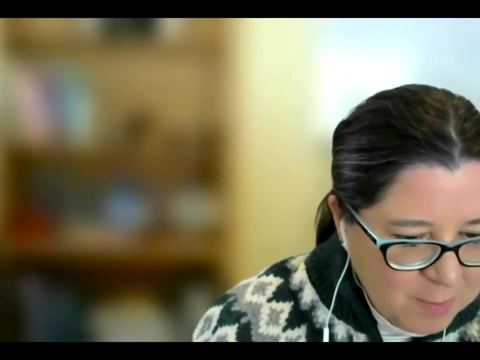 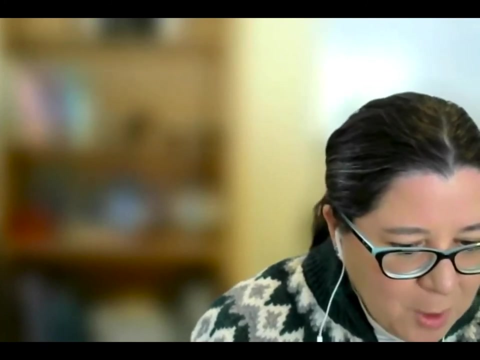 okay, we have one question saying um, what do you think about the use of a water holding system? or saying, um, obviously a continuum from a pile of debris to sophisticated composting. um is anyone looking at mulching? isn't mulching really a form of composting? we're experimenting. 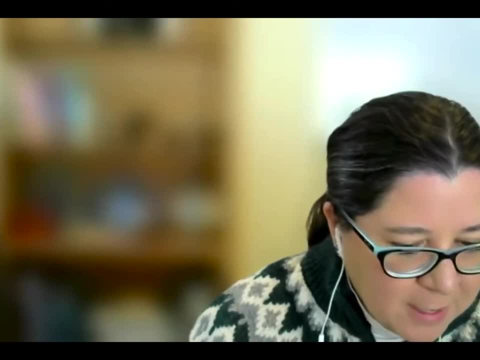 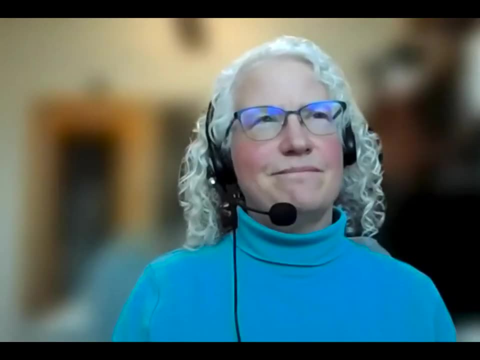 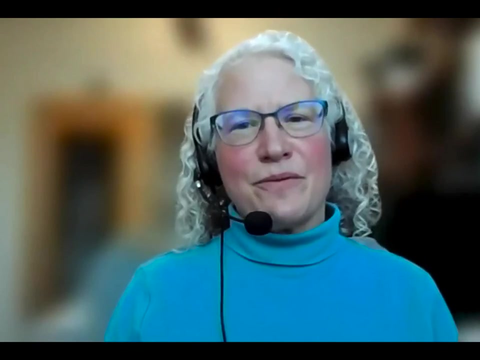 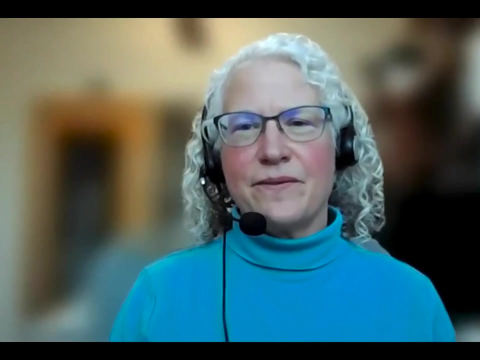 with this german mulching technique on our community raspberry patch, deep layers of organic material from hardwood to leaves. i would. you can use compost as mulch, but i would not call mulch necessarily compost. compost is a very prescribed process. it's a regulated process driven by biology. that's been. it's not just a pile of debris, you know, and i think a lot of. 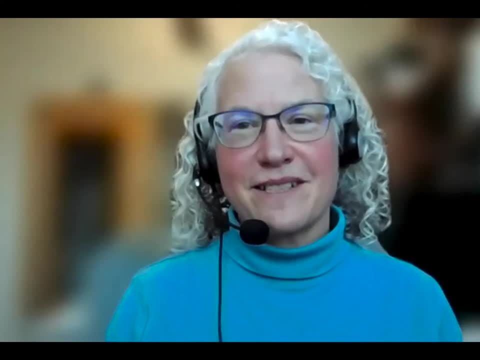 people want to say it's compost, but it's a very managed, controlled process and i you can, and i think it's very um, it's very regulated process. um, it's not just a pile of containing a pile of material, tooyu contrast: material from hardwood to leaves, i would, you can use compost as. 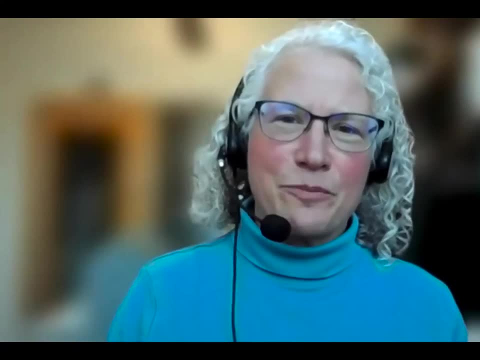 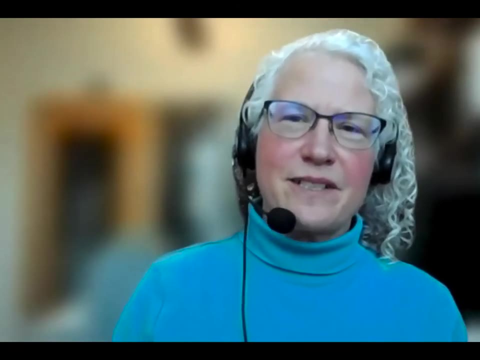 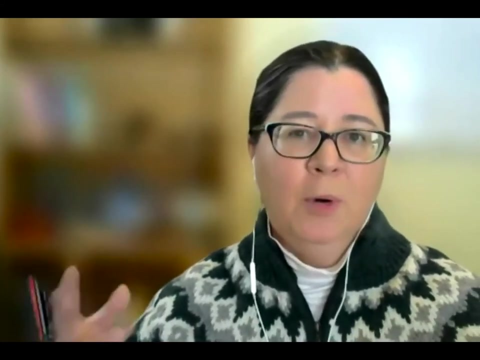 jump in. uh, natasha, but i, when i think of proper compost, it's really going through that thermophilic phase and it would have a different name. if you're doing something else, yeah, and i mean that will break down. i mean it will. you know, just like on a forest floor, it will just decomposition, it's just. decomposition, so it's not exactly compost. yeah, yeah, unless, unless you're managing it on the sort of like a spread out composting system perhaps. so what's what's cool, though, now that you bring that up, is really the process, the succession of organisms you see in the compost. 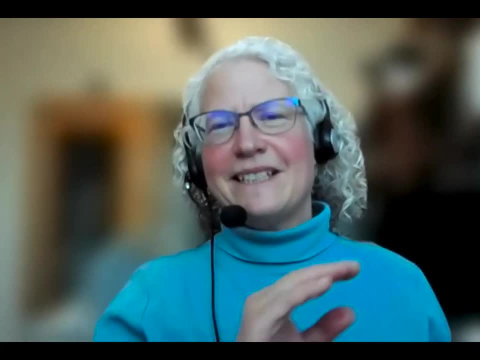 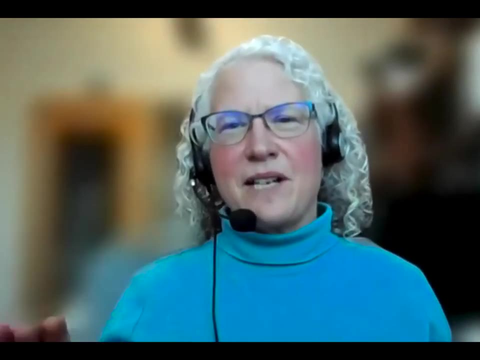 pile do mirror what you see in nature in decomposition. if you were out in the forest soil, for example, or in a pasture, you know they follow the same kind of patterns as far as who comes in early in in the decomposition and who comes in the middle and 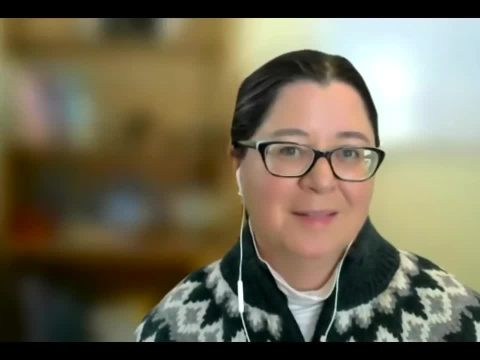 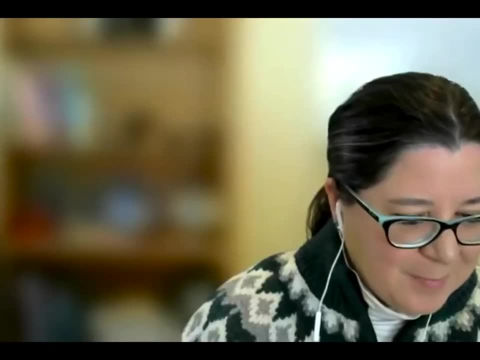 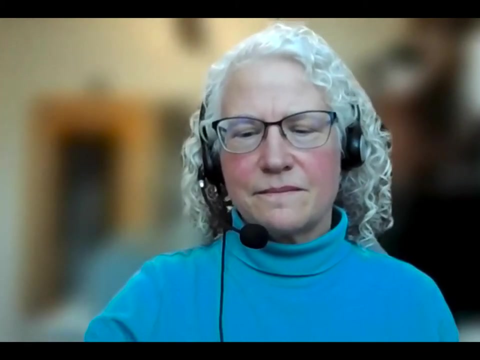 later, nope, nope, so we can learn from the natural systems about what we might expect in the composting. thank you, um, uh, someone would like you to discuss the use of compost tea as a pathogen suppressant. oh, that's a tough one. tea is tough because it is has a short. 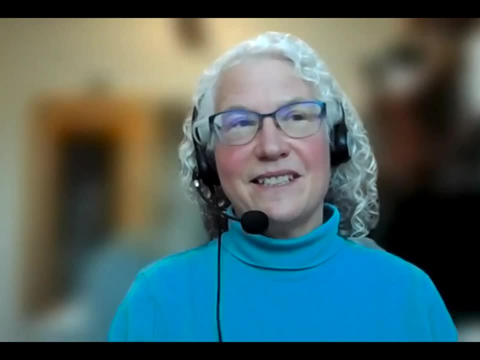 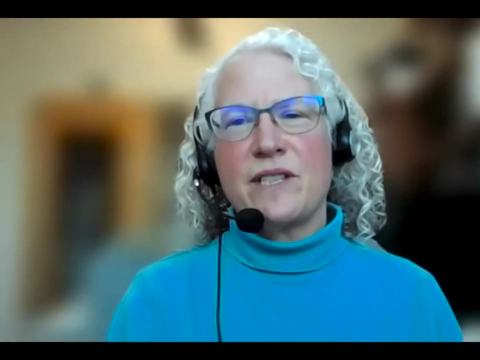 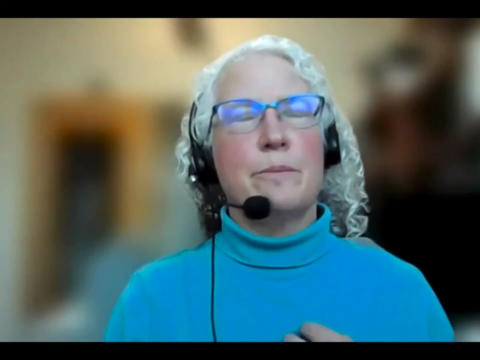 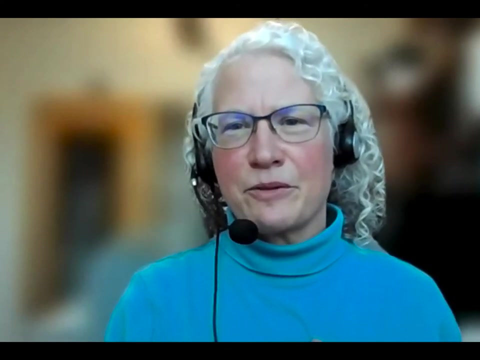 shelf life. potentially, there's uh and how it's managed and treated, whether it's aerated or not, you know. um, i think it has potential. my professional opinion would be it might be more useful on uh above ground foliar diseases. perhaps it would have to be spread regularly, because every time it rained you might be. 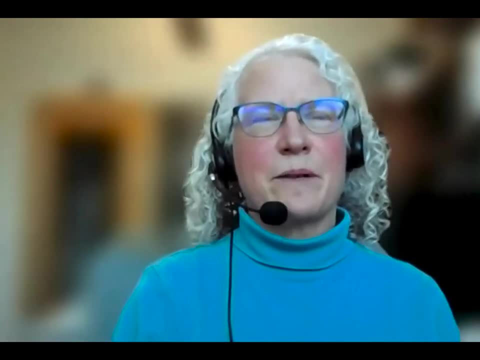 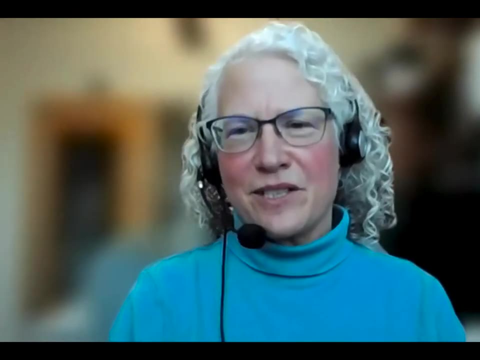 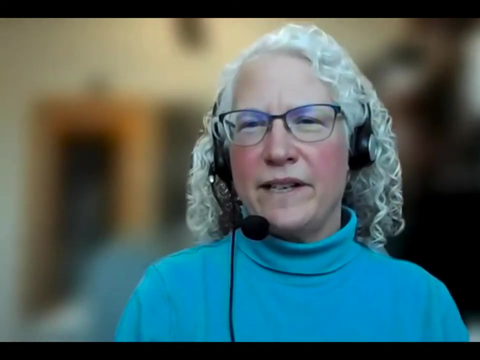 washing it off, but it's something. i had tried some experiments in the past. i was just unable to replicate the disease in the greenhouse environment that i was hoping to. um, so i some. i don't think it's been studied as well as, as you know, the solids. 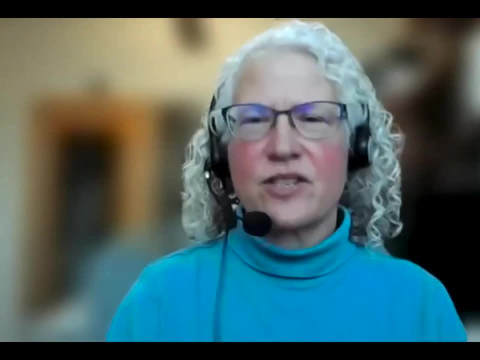 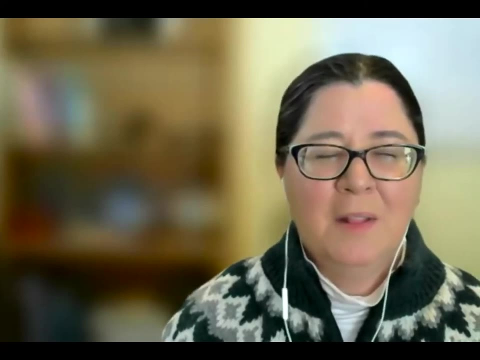 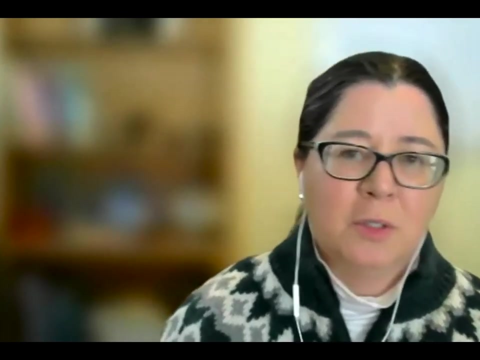 so i think it has potential. i just don't think we have a lot of strong evidence to give you concrete case studies. yeah, and the what i, what i can think of, has to do more with foliar application than a soil-borne um disease suppression. so that's yeah, that would be my 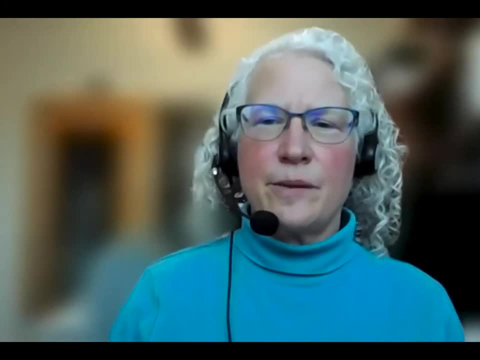 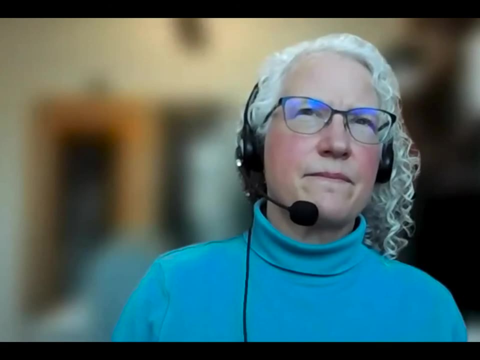 prediction is foliar and i was thinking, because i have talked to people about maybe strawberry diseases, since that's a high cash value crop as an idea, but the interest of botrytis. there's also some- uh, we were looking at one on cabbage, i can't remember what it was, another one that was having 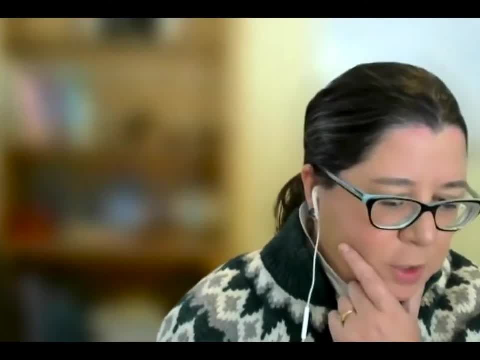 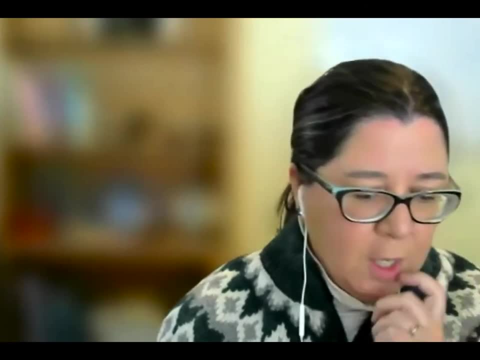 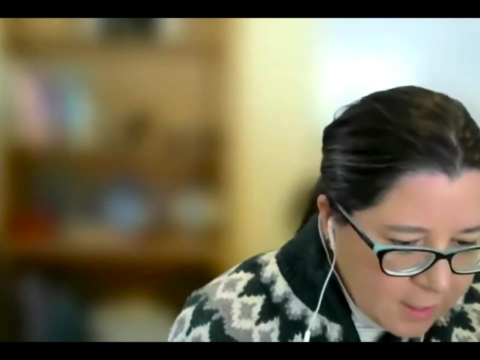 problems. we have two more questions. so one is about um, whether compost- and i'm going to insert here thermophilic compost- um, has there been, has that been found to have an effect on the jumping worms? i've- they say they found them in their home compost and is 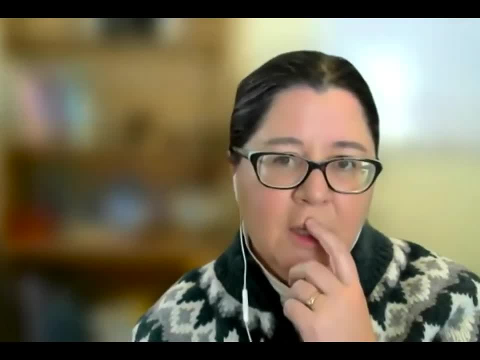 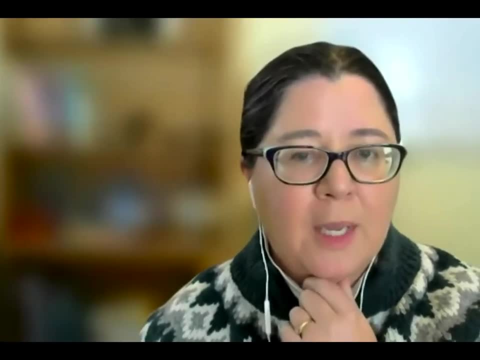 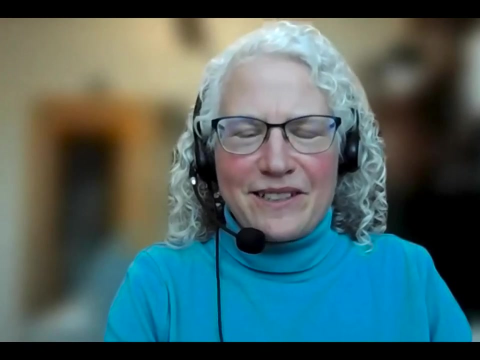 their way to get rid of them and still use the compost. oh, are they talking about earthworms, the jumping, the invasive, the invasive ones? yeah, the snake worms or jumping worms, and are they? i'm not sure how did that? did they get invaded? or they were using jumping worms as their? no, i think it's. 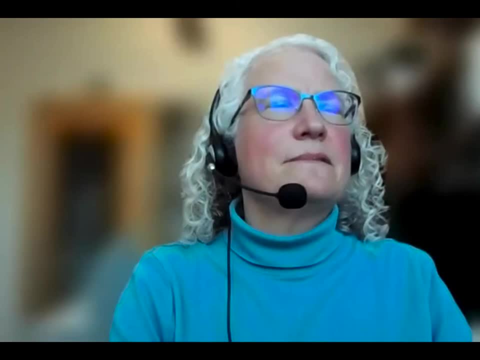 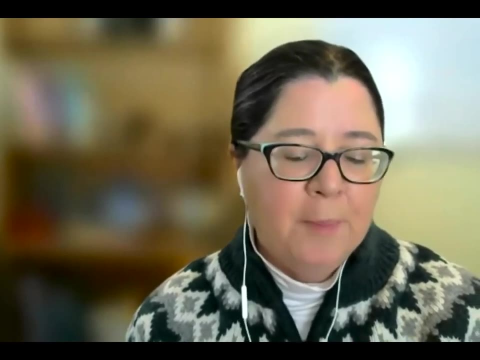 the compost pile just there was invaded. that's invaded. that's my question. so i actually, do you want me to jump in, because i've actually done a little bit of work with dr joseph gores on this at uvm. he's definitely the local person, um, and maybe we'll have him come and do a talk for the 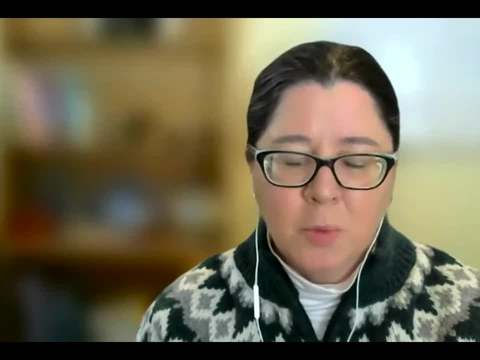 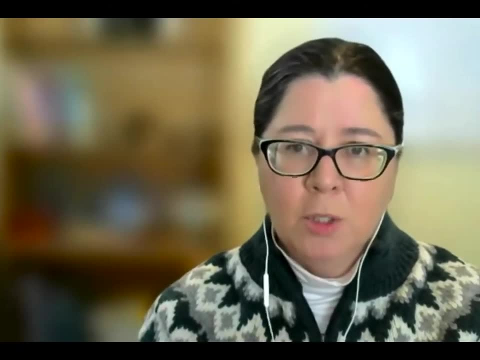 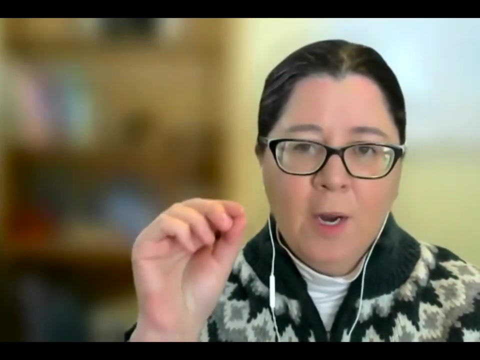 um, this coming may there's the next vermont organics recycling summit, because this is definitely becoming more of a problem. so what has been found is that those hot temperatures will kill jumping worms as well as their egg sacs, but those little creatures are very adaptable. 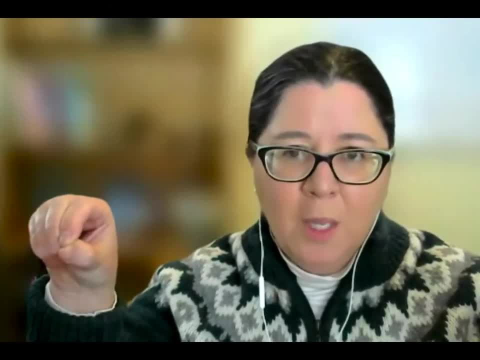 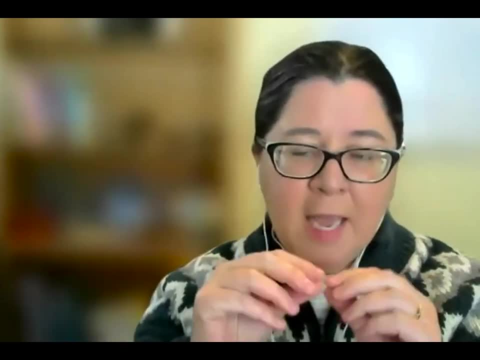 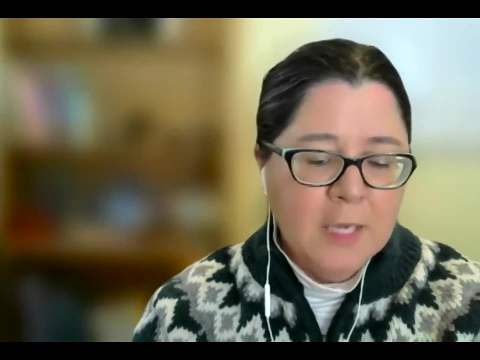 at moving to the colder edges of the pile. and so there have been cases where you see, um, you know the, the egg, obviously the little egg sacs can't move, but they you won't get a full kill. and what i actually was just speaking with him about this, a few weeks ago in fact, and he said: 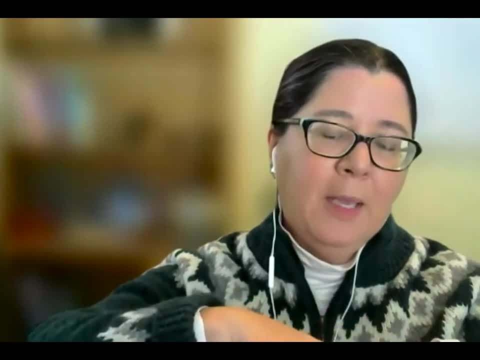 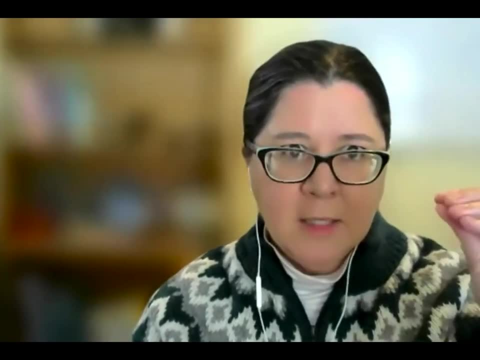 that he's had really good luck with solarization. so really wrapping, and you can do this at your home- compost. so wrap that compost pile that's infected with- uh, you know, with good plastic solidly, and then you can do this at your home: compost. so wrap that compost pile that's infected. 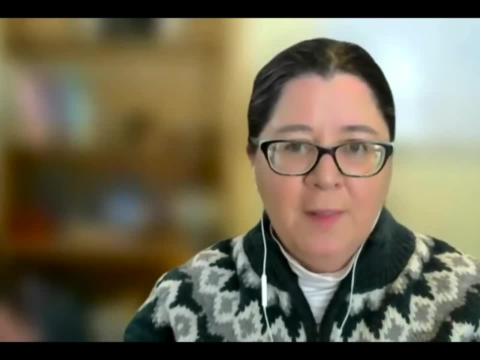 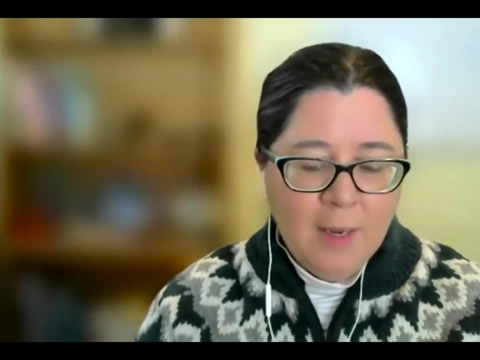 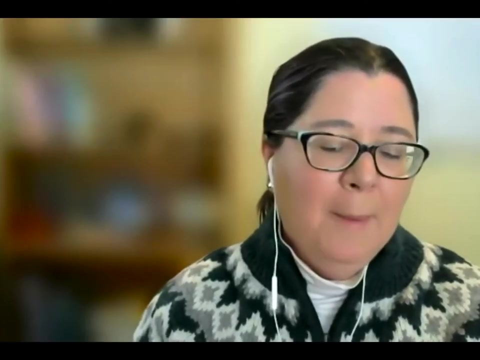 with a layer of plastic and actually weight it down at the edges, and that will kill them, because then it'll get nice and hot. so the temperatures do it, but those critters are very. you got to constrain them spatially and force them to be in there. yes, right, that makes sense. yeah so, yeah so. 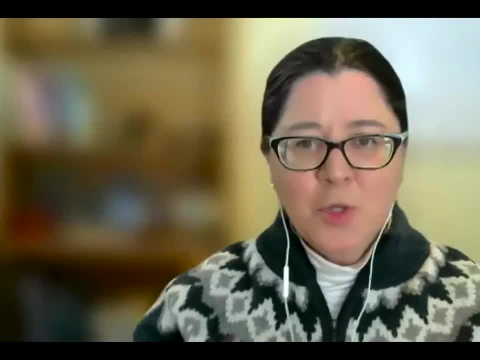 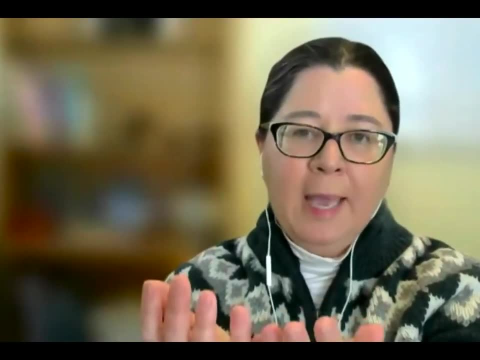 the temperature piece is still working. it's just you got to confine them, that's right. so if you think about a pile, it's always warm in the middle right, and that's why we turn it to let all of that material get up to temperature. that's why the temperature piece is still working. and then you 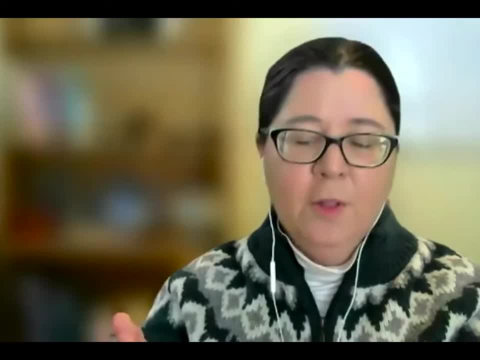 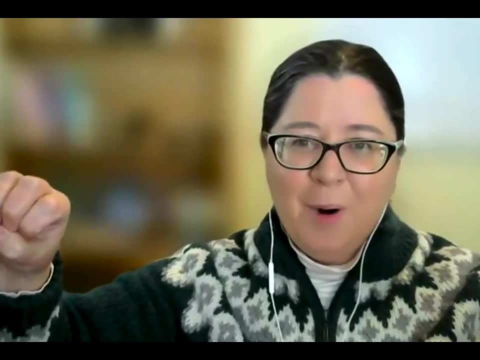 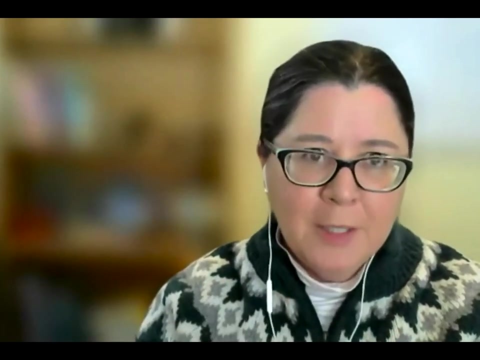 the best management practices are in place with, with the, the turning of the compost for different systems, but they're quick enough to leave the, the hot part, and just hang out on the edges where it's cool enough for them to survive. the other thing i'll just say about that is, if you do manage to kill them. you really want to make sure that you're not reinfecting compost piles by leaving them out, because you can have maybe a a clean compost pile that's finished, but, depending on where it is, it might get reinfected or invaded by these, um, by the jumping or snake worms. well, and while you're, mentioning that some people complain and say my compost has weed seeds. well, two reasons could be. one is it didn't reach the thermophilic phase, but secondly, it could have been clean and maybe the seed blew in be another reason to cover by birds. if you didn't um, cover it um. and then the other. 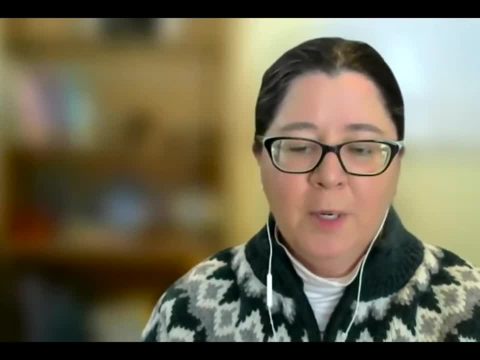 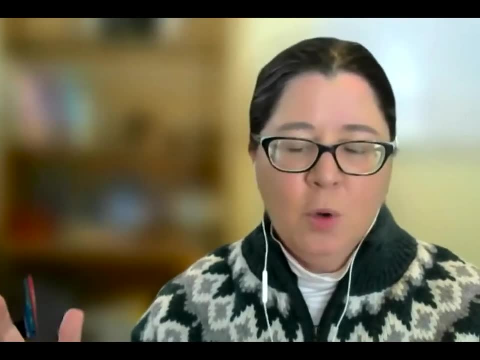 thing that i'll just mention that we've talked about a little bit it just in other webinars, so, just briefly- is just to remind folks that you're applying compost and you are actually, you know, making that soil a more habitable place to um, for things to grow and soil. has a natural seed bank in it, and so you could also be creating a much nicer environment for those weed seeds to come up, and so it really. you know this. it's not always the compost's fault specifically. so, yeah, you just use your hoe when you open. that's it allowing those seeds to to. germinate, and yeah. so just to keep that in mind, good point. and then, uh, let's see. um, to prevent the loss of nitrogen from compost spread on a garden, this person has heard that you should cover the compost with a little topsoil to cap it. i'm not familiar with that. i'm not sure either, are they? 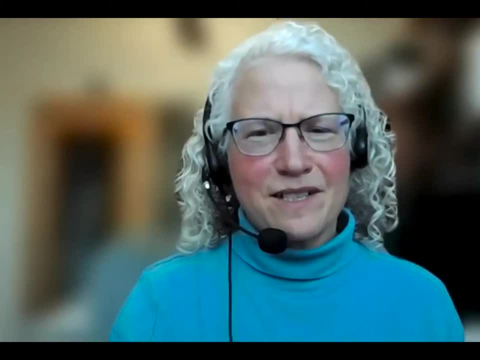 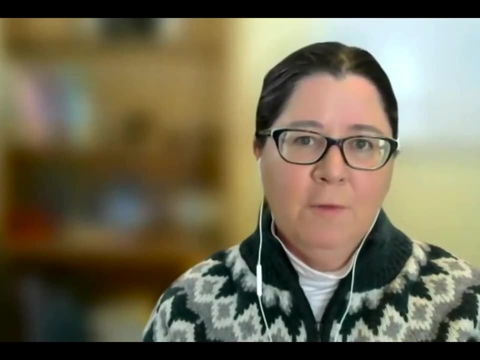 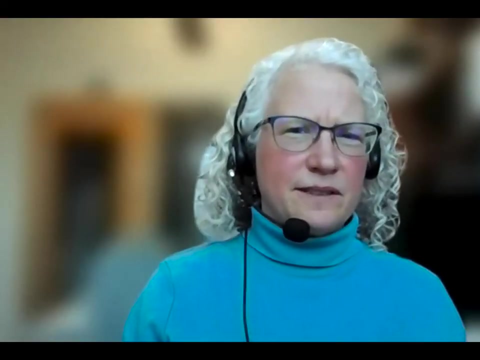 thinking of when it's in a pile and capping. i mean, i've seen some capping when you're making it, yeah, yeah. so ideally you're not going to have volatile nitrogen in a finished compost product, which is when you're applying it to gardens. i think that's a sign of being immature, yeah, yeah. so on the, the composting association of 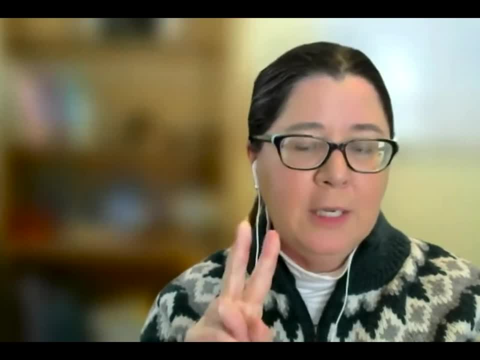 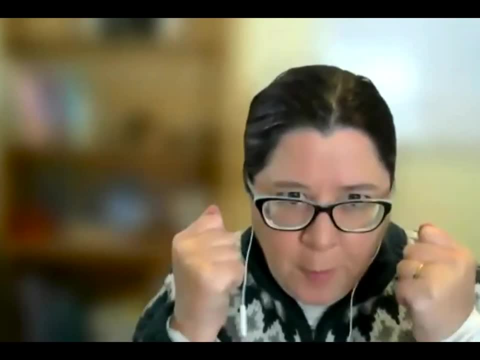 vermont's website. we have a little thing about two different easy at-home tests to do. one is a ziploc bag test where you put some compost in it, you close it up for three days and then you open it and smell it right away and you can get more information about how to do this. but if it smells like ammonia, there's still nitrogen. if it smells kind of sour, there's still carbon, and that's just an indication that you haven't. it should just smell like nice moist earth when you open it up. um, and if you know, those are materials that are so involved in the phytotoxicity problems. 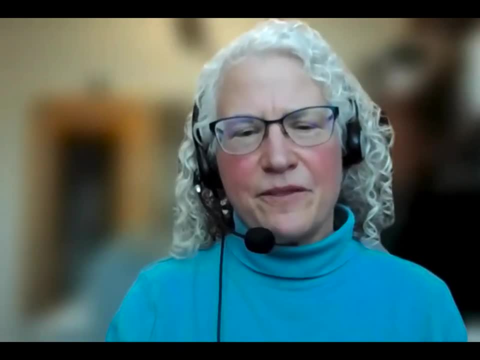 if you're using immature, it may, you know, be phytotoxic and inhibit plant growth. so that's another reason to have it mature. let all those organic elements grow and age, because their bacteria are going to start to die. would you imagine that that would happen to them? i mean you. 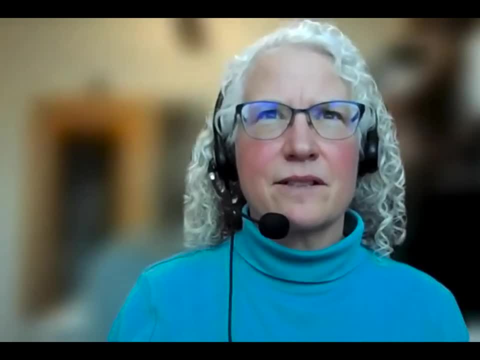 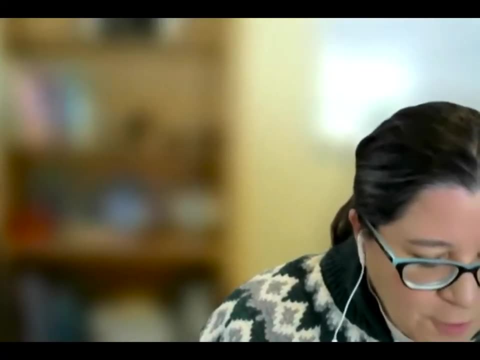 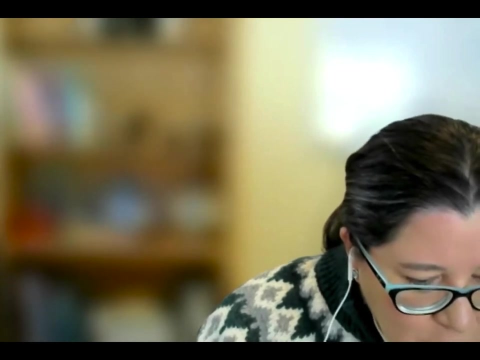 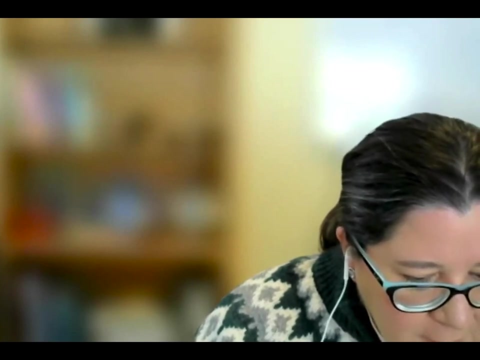 acids dissipate, not have the ammonia, etc. yep, but that's a great test, great simple test. yep. and the very last question, um should for today. should, uh, we till native soil with compost to improve root penetration or drainage, or should we just use the no dig method and lay the compost on? 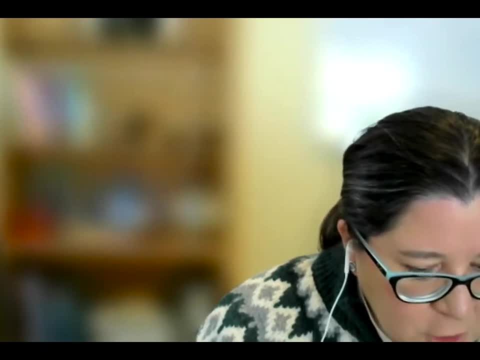 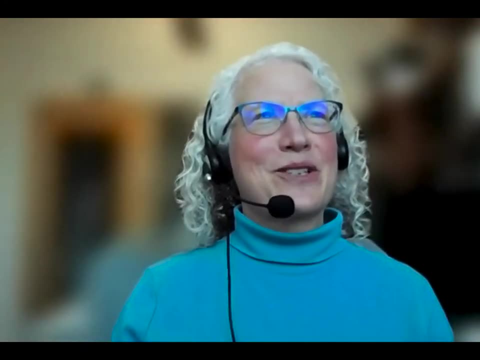 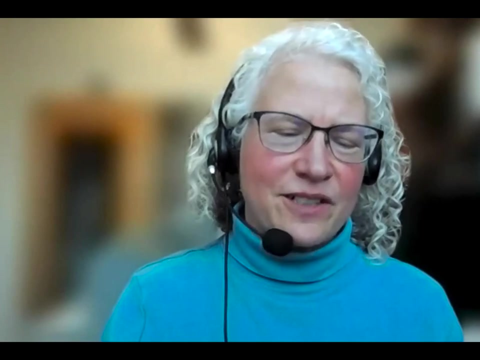 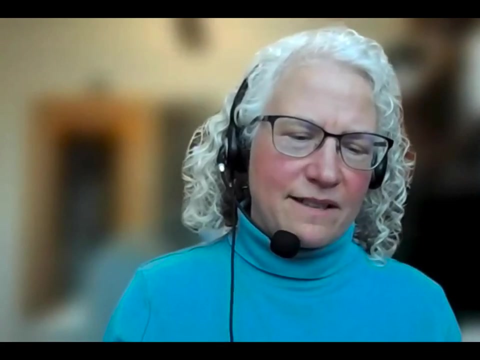 top of the soil, just wondering about what is best to prevent destroying the native soil structure. that's a great question and one i kind of- yeah, always struggle with myself, because tilling and disturbing it always really, and changing the physical structure has a huge impact on the food web. so, okay, so, um, i've done, i've tried both myself, just experimenting on my 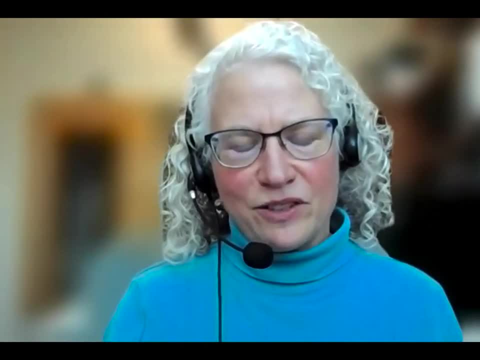 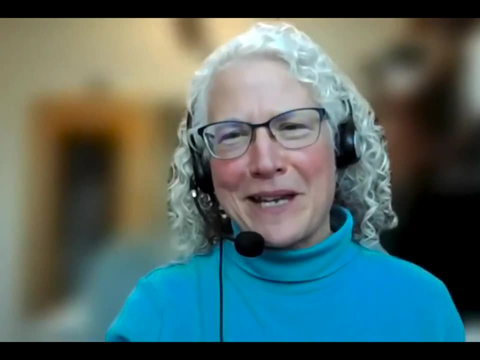 own yard. i've tended to mix it in, but if you layer it on, the thing is you need something that's going to be moving it up and down for you, and if you had a native earthworm, that could be one option. you know some kind of soil organisms that will help you work it down, because somehow you're 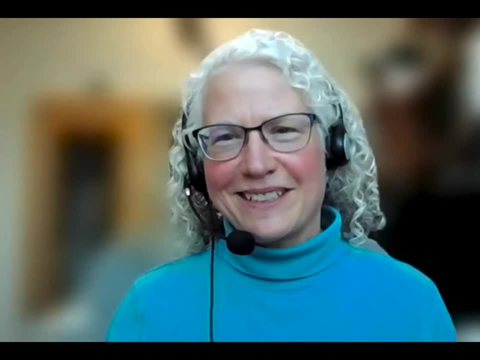 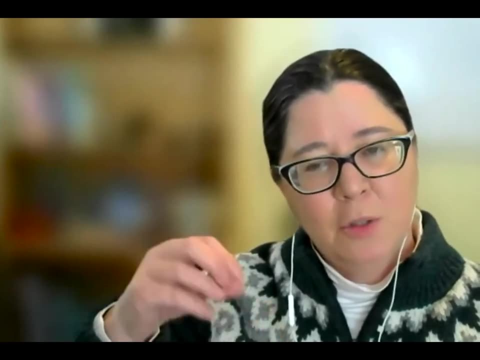 going to need to get that in the soil, otherwise it's going to just be like mulch, but you you may not also want to plant directly into compost, and so there is going to be some mixing, and so just a couple other things to think about. one: i often, when i get that question, say it can really depend on the soil, that the native. the native soil that you're using. is it like a nice, healthy, uncompacted, not, you know, overly used soil, or is there that hard pan because there are times where you may want to do some incorporation? so it depends a. little bit on how degraded the soil is at the site that you're using the compost on um, and then as well there are. you can just sort of like spotting the soil and then you can just sort of like spotting the soil and then you can just sort of like spot, use compost, so like, if you're dig you know you need. to get a seedling into a garden. you can't mix, you know, when you dig that little hole, you can also just sort of spot apply the compost there and then mulch with compost around the top and it will integrate, i think, over time. but um, but those are just some things that i think about. i'll mention 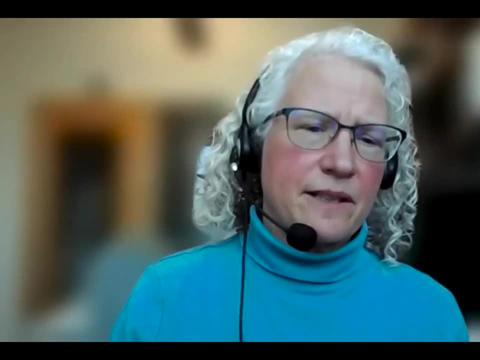 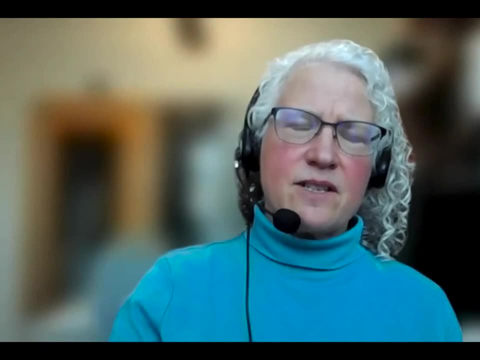 another thing that we've been experimenting with- and you know we haven't wrapped up all the results yet- but the idea of mixing the compost in with a starter mix, that you put your seeds in, so when that seed germinates, all those little rootlets get covered with the. it's kind of a prophylactic. 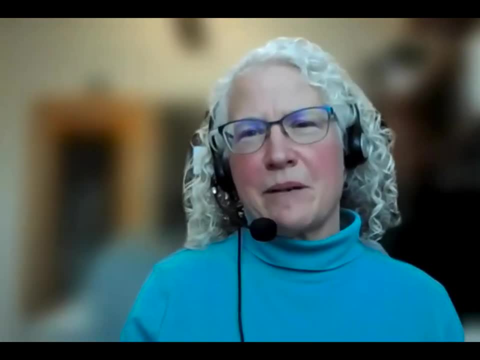 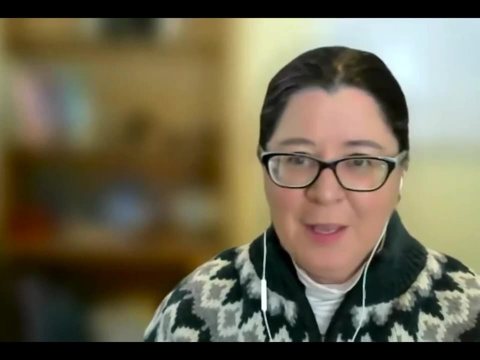 covered with those biocontrol, so we're experimenting to see that might be another way to introduce it into a system. but yeah, yeah, there's a bunch of different ways we can go here. well, thank you so much, deb, for joining us for today's program, and thanks to all of our participants for taking some